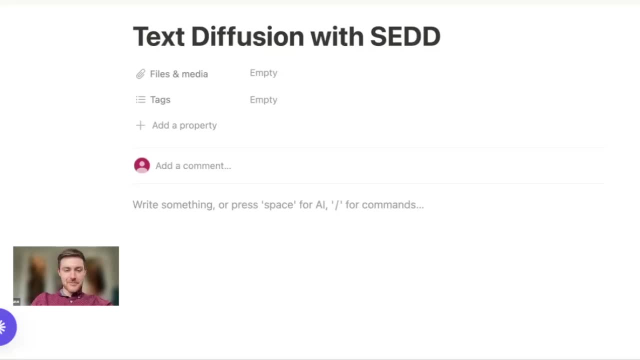 Welcome everybody to Archive Dives with Oxen AI, where every week we dive into some of the newest and coolest research papers in machine learning and AI, with the hopes that you'll then be able to apply them to your work. So this week we are going over a paper called Discrete Diffusion. 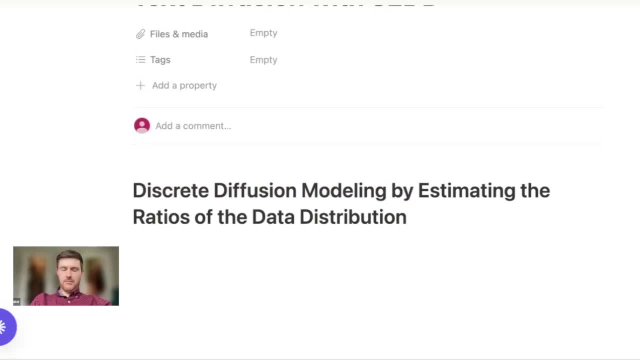 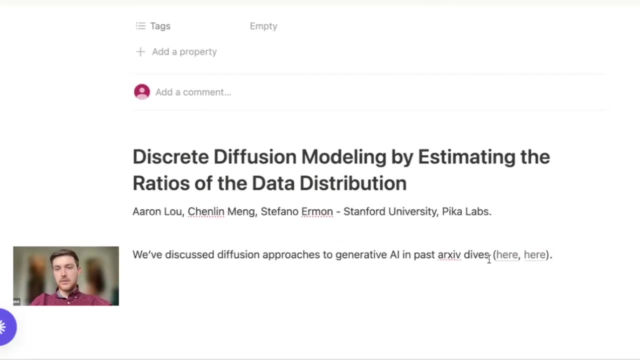 Modeling by Estimating the Ratios of the Data Distribution by these three wonderful researchers at Stanford University and Pika Labs, And this is a paper that is fundamentally about applying diffusion techniques, which we've discussed in past dives but also are kind of more widely known. 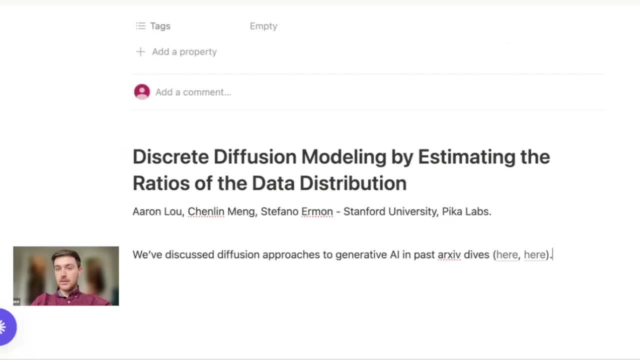 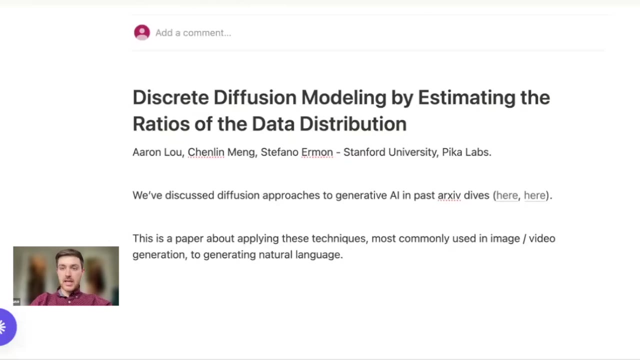 for image work, like stable diffusion, and video work like Lumiere, and taking those and applying those to natural language generation. So this paper is not the first time that you know a group of authors has attempted to make text diffusion work. There have been, you know, past. 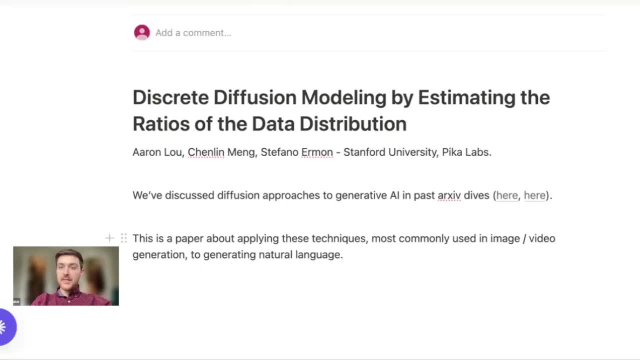 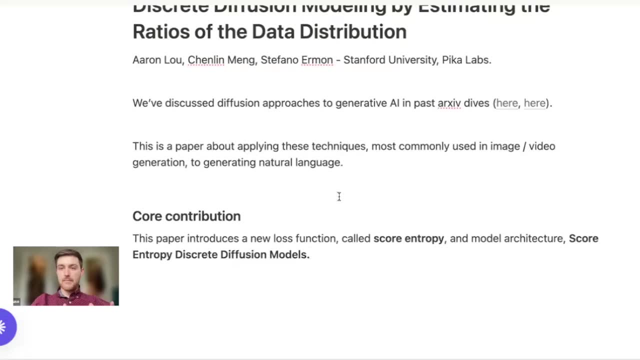 stabs at this with varying success. but this kind of paper's core contribution is that it's the first time that a group of authors has attempted to make text diffusion work. It's the first time that those approaches have been competitive for the same model size. 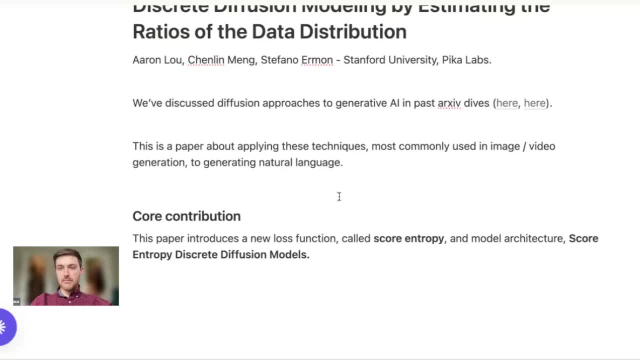 with the kind of autoregressive next token predicting models like the GPT series. The way that they achieve this is through a novel loss function that they introduced called score entropy, And you know, that's kind of how we get the name of these score entropy. 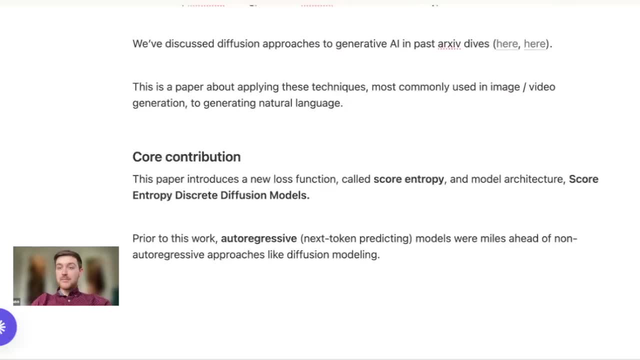 discrete diffusion models. So autoregressive modeling was completely dominant before this, and the discrete diffusion approaches that have existed for text were never really able to match up. Like I said, because of this loss function, these models are now able to match performance at a similar 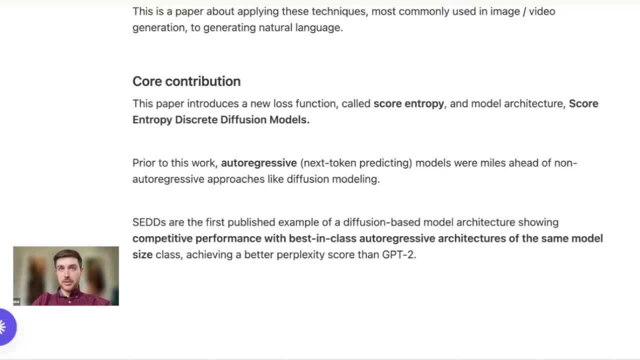 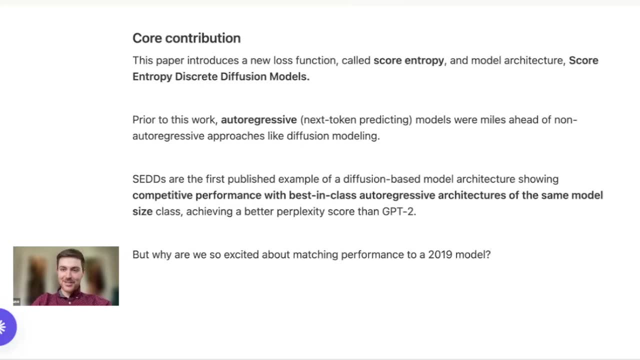 model, model architecture and model size. on GPT-2, which is really exciting because we were really nowhere close to this before this paper, But I can hear the objections that you know. GPT-2 kind of was published in, I believe, 2019.. We are on GPT-4, GPT-4 plus five right around the corner now. 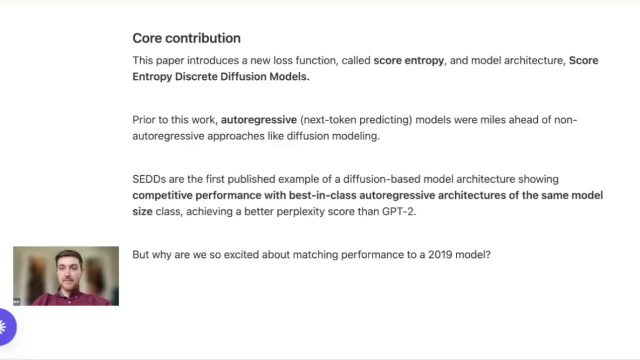 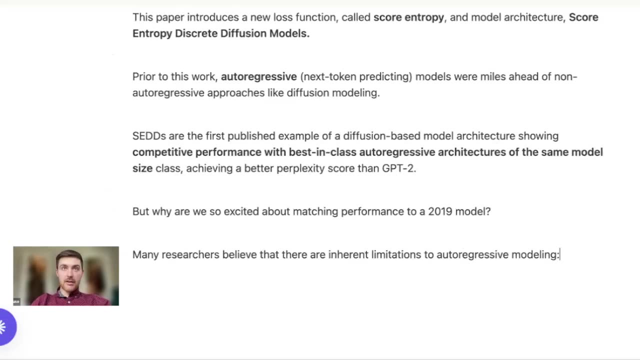 So what is so exciting about a diffusion approach that is matching performance with a 2019 cloud? Well, I think it's really interesting to see how this is going to play out across autoregressive model. The biggest thing is that a lot of researchers believe, and I find it pretty compelling. 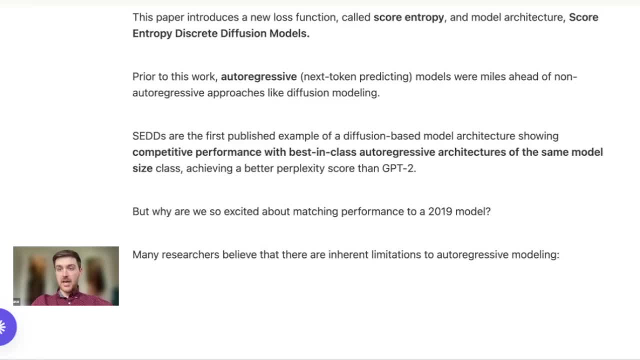 that there are some inherent limitations to this autoregressive style of modeling where to predict token i, you use all of the tokens i minus one back to zero before that to condition that distribution First. one of these drawbacks is that you have to 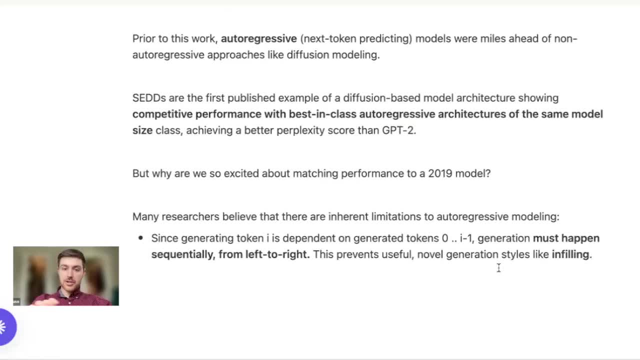 you know, sample your tokens and you have to produce your generation sequentially in order from from left to right. There are things that we can do to parallelize this more effectively at training time, but at inference time that still kind of imposes a structural limitation. 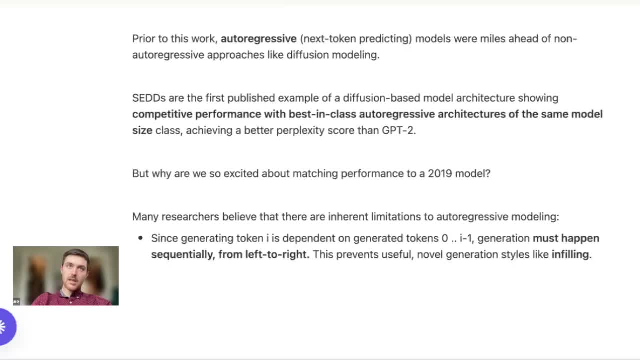 on how the data is actually being generated. This also kind of prevents us from doing techniques like infilling, where, if you think you know there are examples in imagery diffusion work where if you kind of take a square out of the center of an image, you can fill it in using 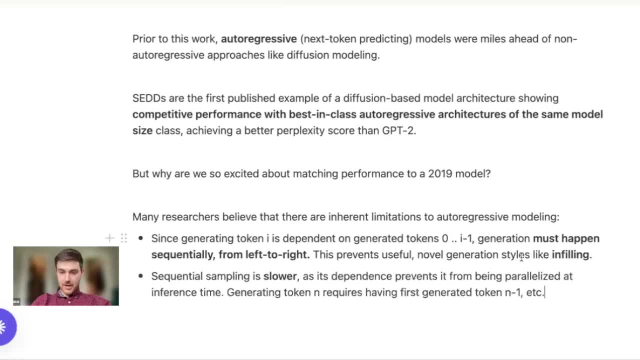 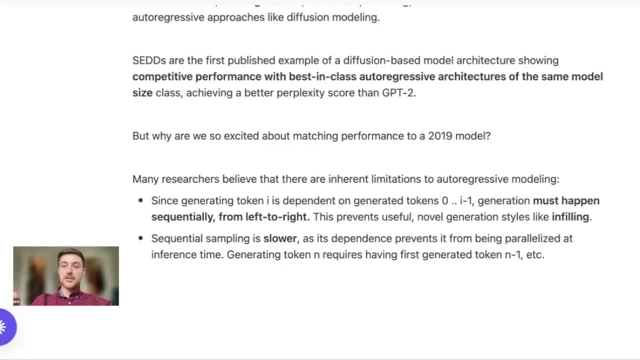 a diffusion model. We can't do that if we're strictly prompting from left to right And prompting from left to right. sorry, generating tokens from left to right is also slower, less parallelizable, because we have to know what came before a token before we generate that token. 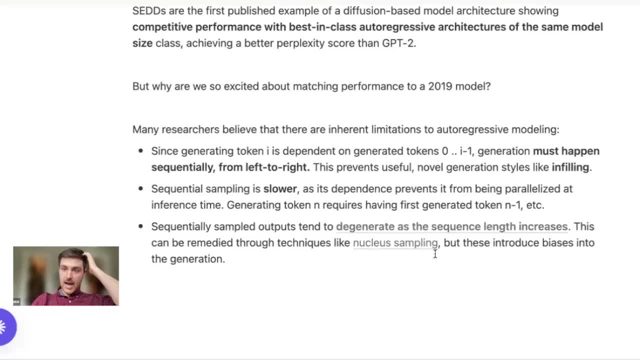 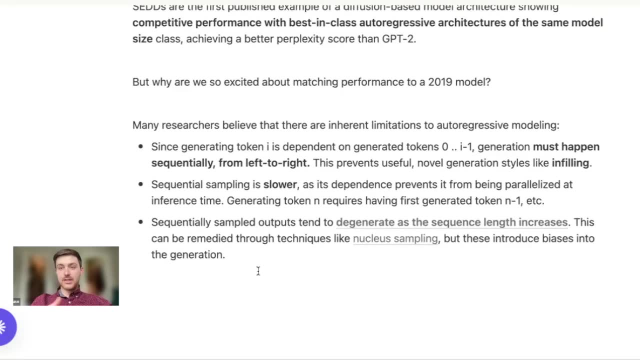 Last big reason here- and we'll go over these again at the end when we talk about how this SEDD model improves on this- is that sequentially sampled outputs have been shown to degenerate as the sequence continues to go on, you know, and continue to generate tokens. 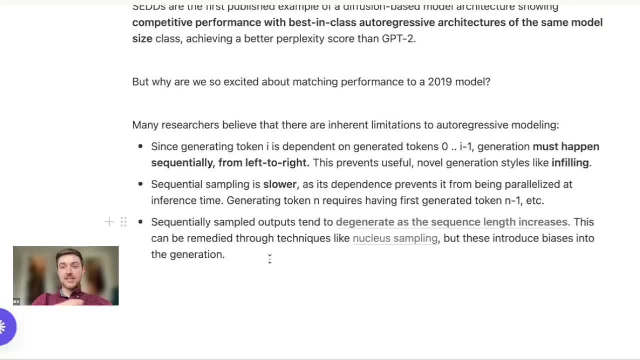 There are techniques that have been developed, sort of as the sequence gets longer, to ameliorate this called annealing techniques. One of them, which we'll talk about later, is called nucleus sampling, and the authors posited this. as these authors are able to, 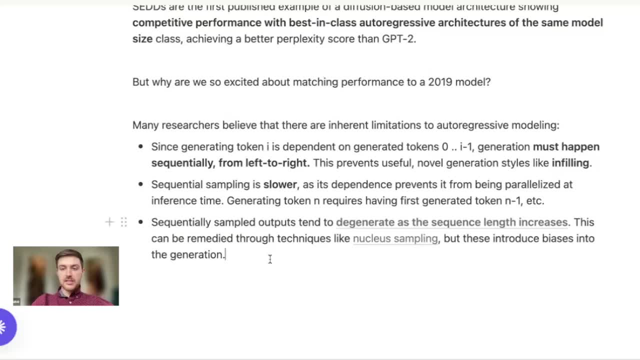 through diffusion, be able to achieve the same level of performance as these autoregressive models without having to kind of bolt on these additional techniques, that kind of clip and and change the distribution as they go. So that's kind of why we are interested in the first place. 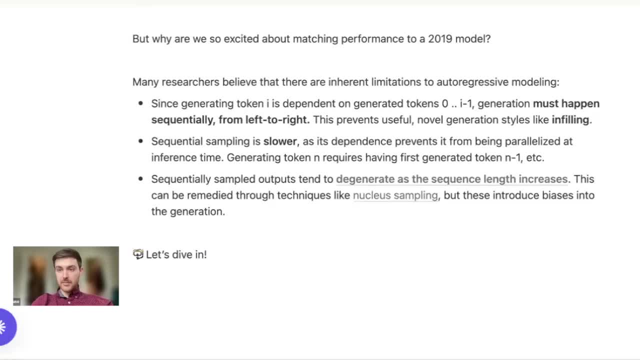 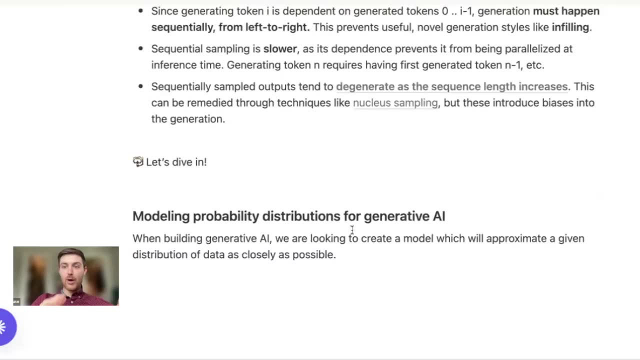 in kind of this different modeling approach, this non-autoregressive modeling approach, and doing this via diffusion. I want to step back from this a little bit and motivate why we want to do this diffusion modeling and why this is kind of where we arrive when we look at ways that we 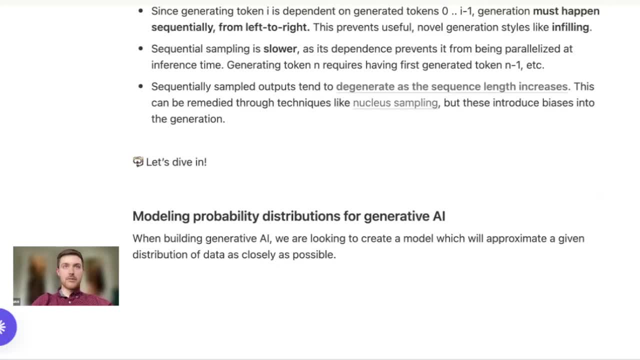 can- uh, you know- generate text without being auto-aggressive, and fundamentally, what we are doing when we are trying to make a generative ai model is create something which is going to approximate a data distribution or data population that we care about as closely as possible. that 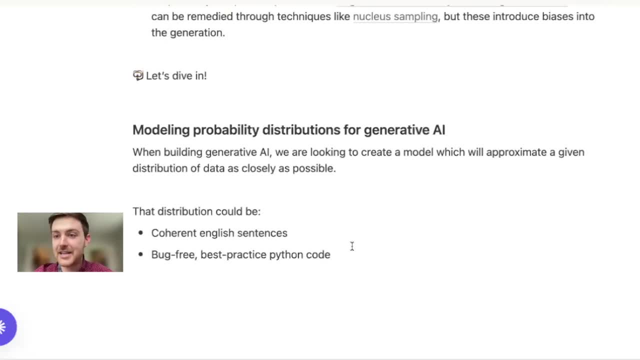 distribution could be anything. um, it could be like the entirety of you know nice, well-structured sentences. it could be bug-free best practice python code. and then, in the worlds of generative imagery and video, it could be, you know, photorealistic images, or cute cartoon images, or 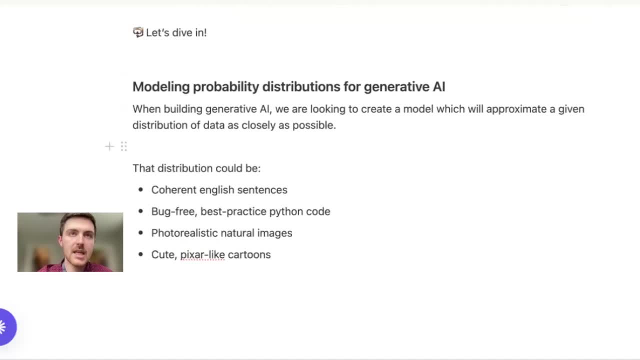 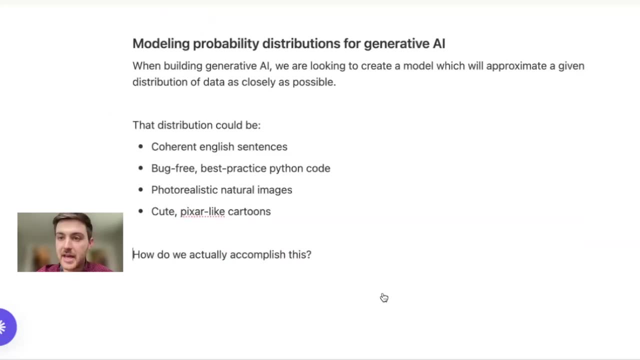 you know any type, and we condition it from there, and that's our goal, right, but how do we actually go about accomplishing that? so there's a thought experiment, um, that jeremy howard uses in his um series. i believe is called like machine learning or, you know, foundations to stable. 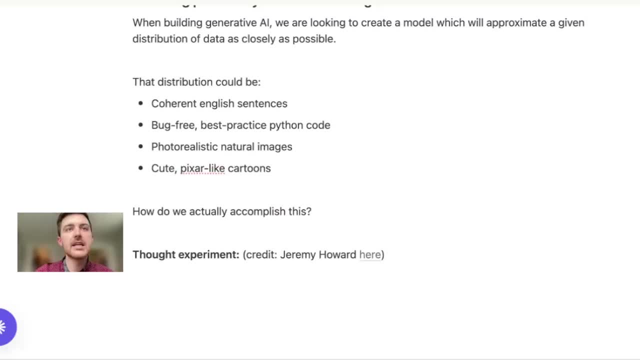 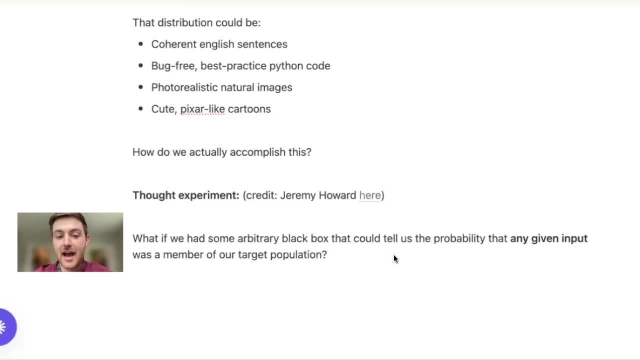 diffusion. it's available on youtube and linked here- and his thought experiment that i think motivates us really well is: what if we had some arbitrary magic black box that, for whatever input we give it, um that it would tell us the probability that that input is a member? 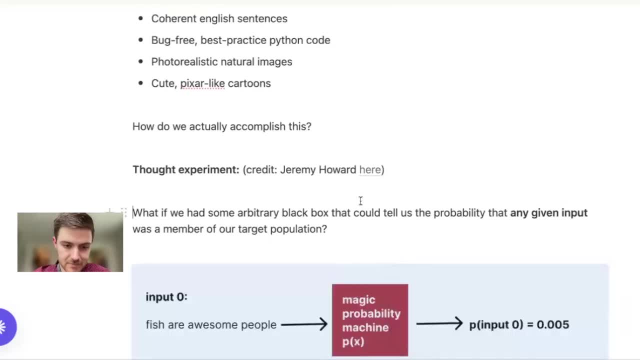 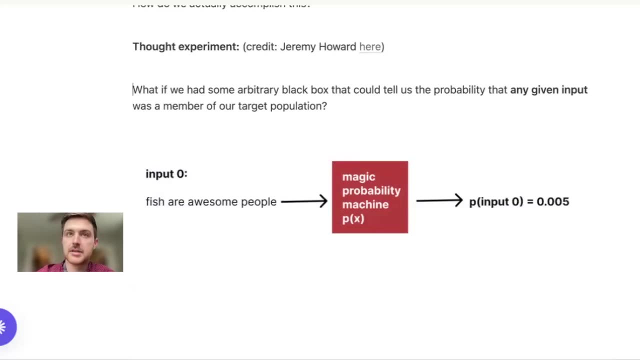 of the population that we are looking to model. so if we feed in a sentence that says, like fish are awesome people, that would give us a, a probability. we don't really know how to contextualize this yet, um, but if we have this, is there a way that we can use this magic thing, assuming that it? 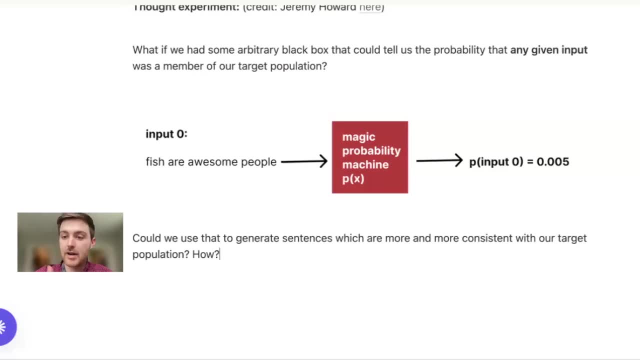 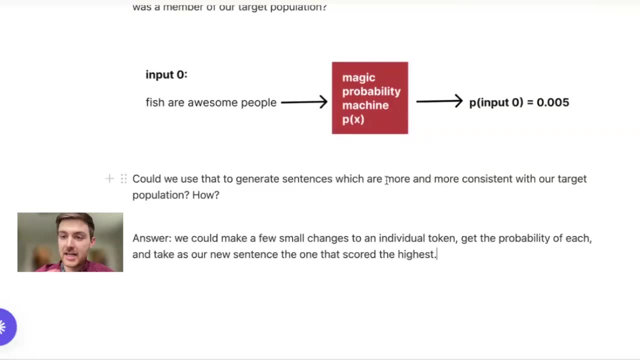 exists and works well, perfectly to generate progressively better and better sentences over time. and how would we do that? the answer to that is that we could make a couple of tiny changes to that input sentence, to those tokens that we're feeding in, and see how the probability changes in the output as a result. 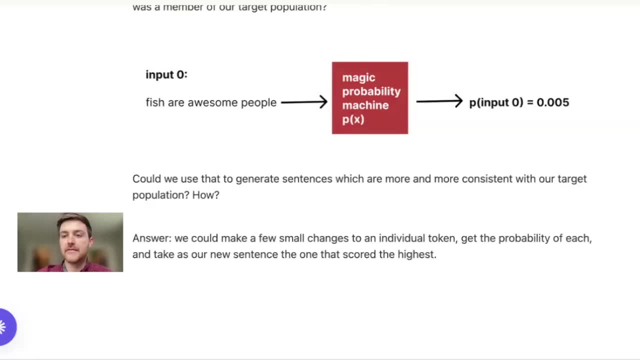 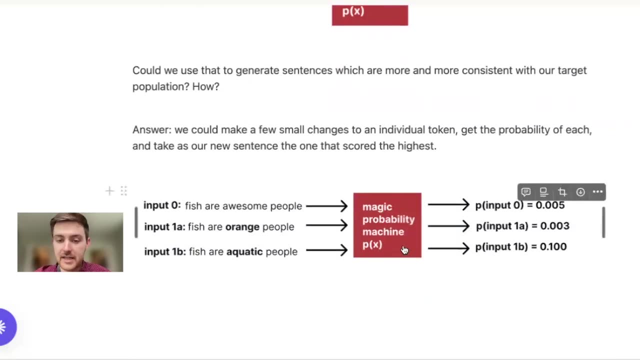 and then we could take the best output and continue to refine it from there. this would be a very lengthy process to do manually, but you can imagine computers being able to do this a lot more effectively and in parallel. so yes, if i had an example here of an example of a transactional function布- withdrawal. 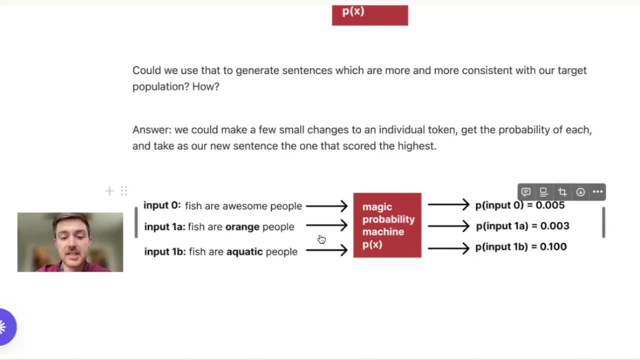 okay. we continuously increase the likelihood that we need anything to start with, to continue arius' or roughness, or even be case case as an example of that. where we take our fish are awesome people input, we feed into our magic block, our magic black box, some other variations on that. 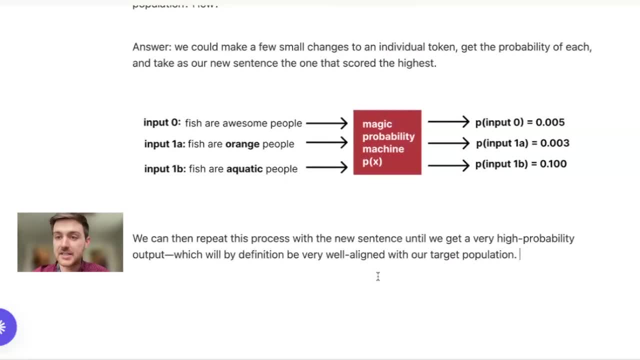 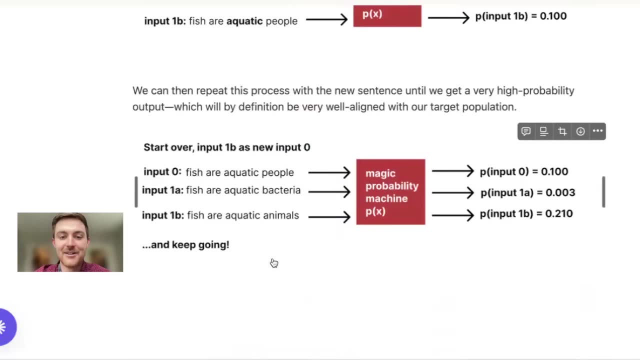 fish are orange people. fish are aquatic people and these have uh kind of changed option from the previous iteration. We could take our fish are aquatic people, because we saw that was some type of improvement, and continue to move forward from there. So now, instead of riffing on, 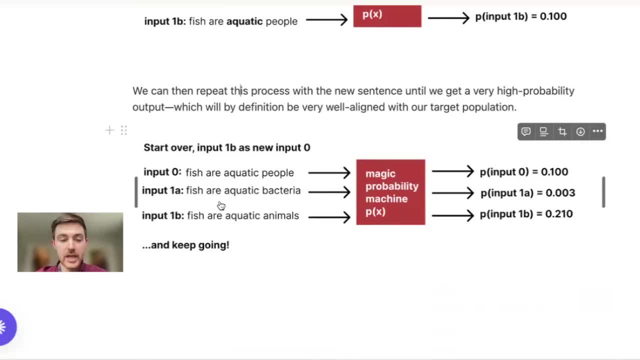 fish are awesome people we're riffing on. fish are aquatic people. Now one of those tweaks leads us to say fish are aquatic animals. We see a huge jump in the probability there and we keep going from there, And now we're able to reliably generate more and more faithful sentences to our 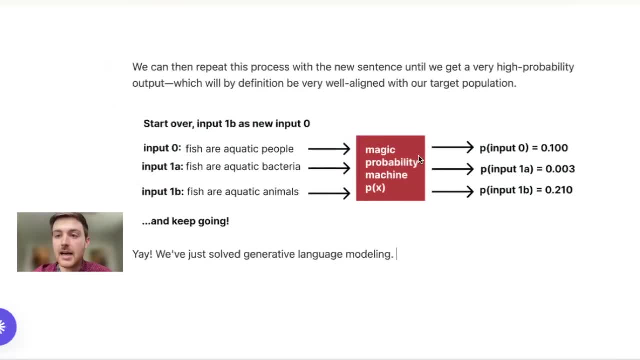 underlying target population And end of talk. we have now solved generative language modeling, and that's wonderful, but obviously not the case. So this is something that just kind of you hear it and you're like, yeah, that probably doesn't work, But let's investigate why, so that we can. 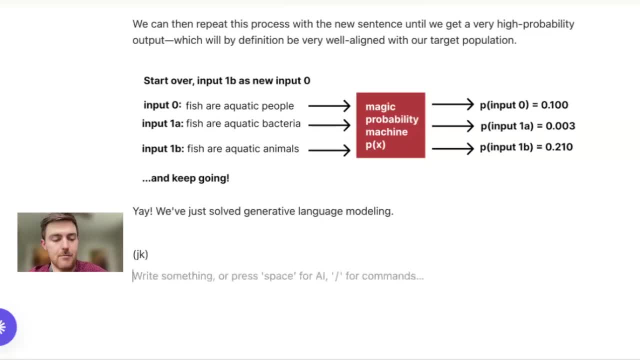 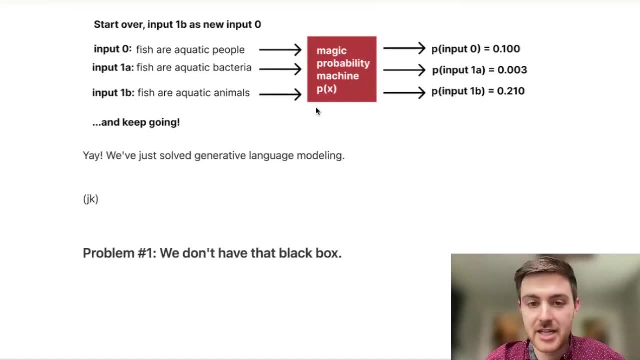 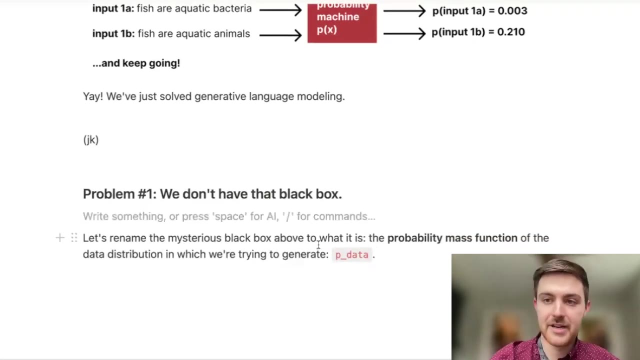 see how diffusion solves it. Any questions up to this point? Cool. So the most obvious problem with this is that this p of x function, this magical black box, is not something that we have, So in statistics land, we can call this by a different name. We can call it the probability. 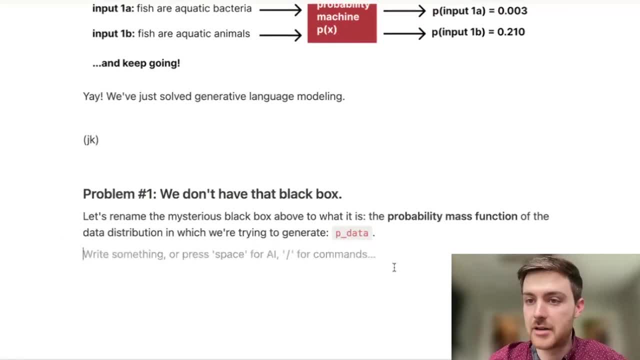 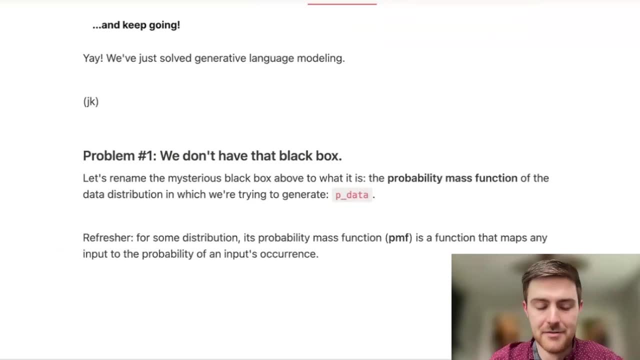 mass function of that data distribution that we're trying to generate. The authors refer to this as p data throughout the paper. I find that very reasonable. As a statistics refresher, we know that for any distribution, the probability mass function, which we just defined, is a function. 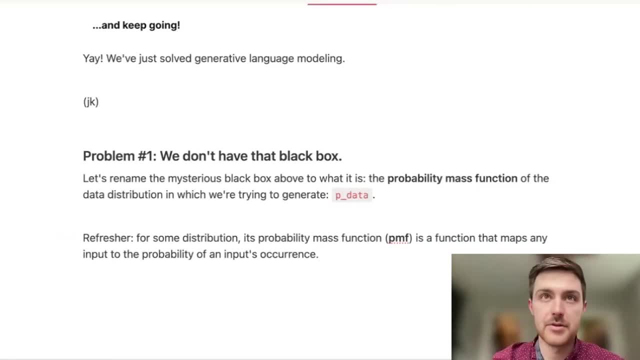 that maps input to their output probabilities under that distribution And a kind of concrete example of this, which, by the way, was auto-generated by I don't know, I don't know, asking ChatGPT to give me this thing and is by all indications correct, is the random event of 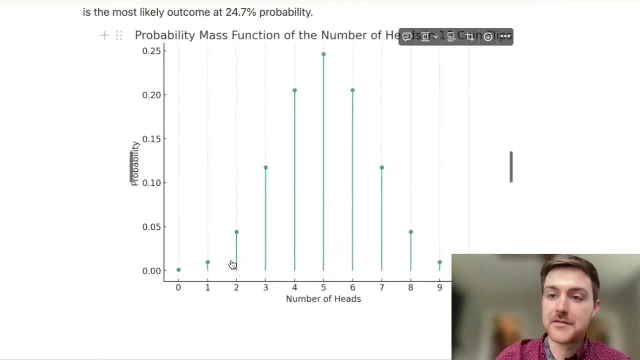 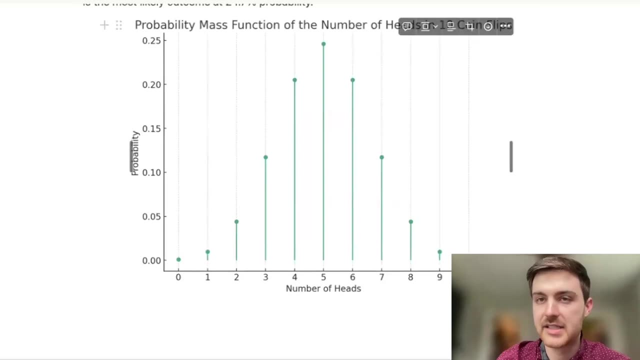 let's flip 10 coins and see how many heads we get right. This graph should be intuitive. Five heads would be what you would expect most often, and you would consider zero heads or 10 heads to be extremely outlying events. But the key is if you were, you know, looking at this function and trying 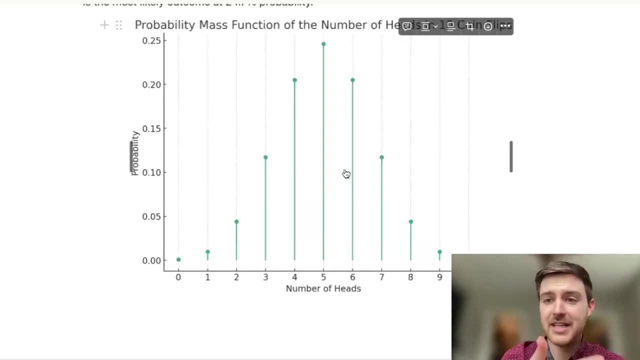 to figure out what the most likely outcome is without knowing it ahead of time. you could feed in zero, see that that doesn't work and step up towards five from there. We're looking to do the same kind of thing With this underlying function. 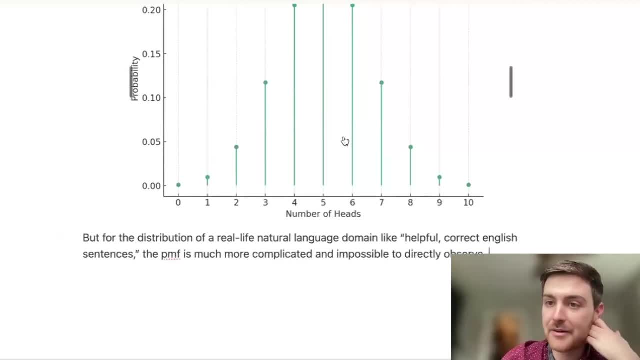 The problem with this is that we are able to model this- you know this small, small scale event with 10 different inputs very easily, But the distribution of things- like you know, helpful correct English sentences or valid Python code- is a lot broader and much more high dimensional. 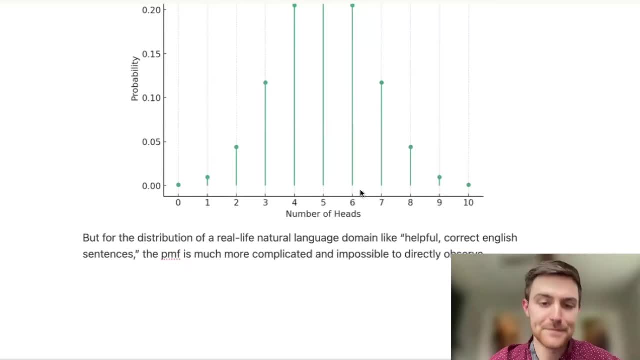 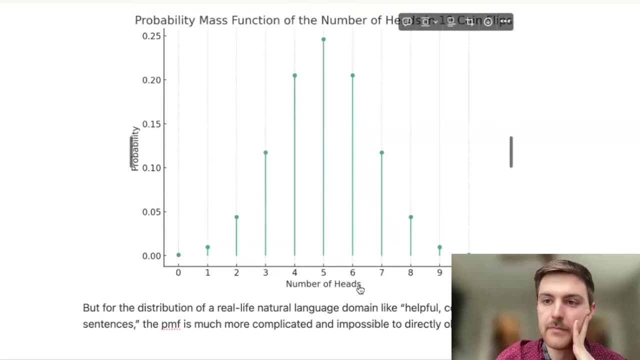 than something like what happens when you flip a coin 10 times. So, Ben, quick question: Probability mass function versus probability density function, Are they the same thing? So yeah, good question. So the probability density function is kind of a equivalent for 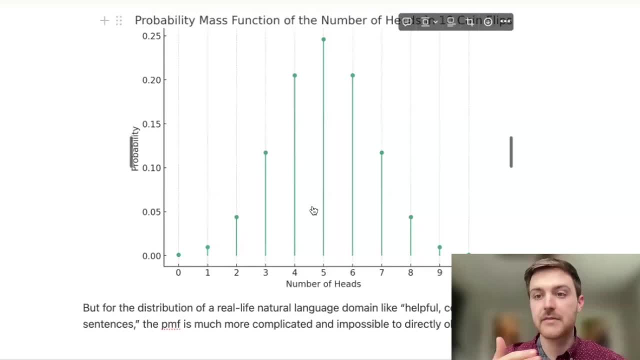 the probability mass function, but for continuous- excuse me, for continuous- spaces instead of for discrete spaces. So language modeling is discrete because you have a certain number of tokens and a certain sequence length and there is a very large number of possible outputs there, but it's a finite. 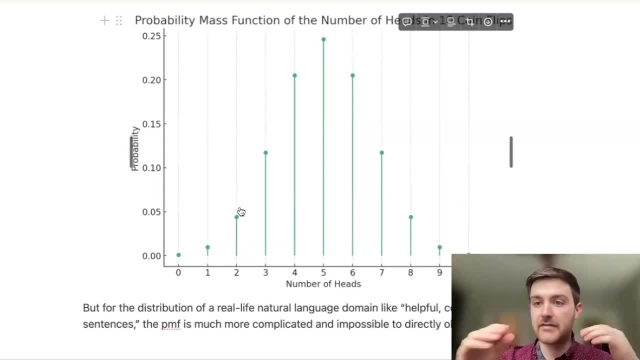 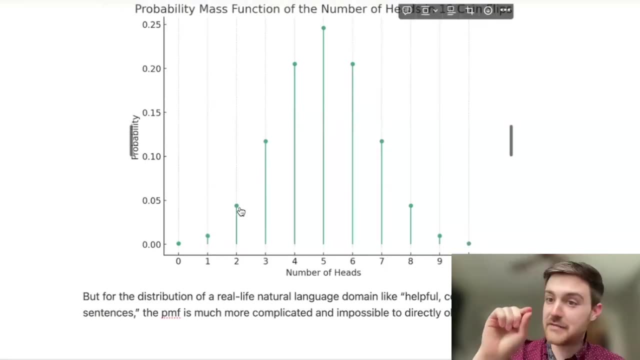 one, Whereas something like generating an image, you have kind of an infinite, continuous sliding scale of pixel values. The only difference with probability density density is that you can't really think of those individual point estimates as probabilities. but that is a little beyond the scope for here for the probability mass function for discrete events. 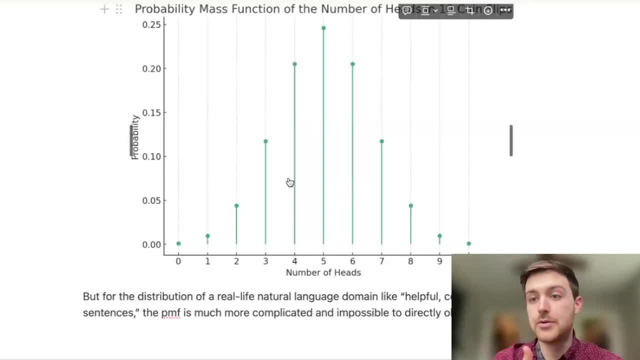 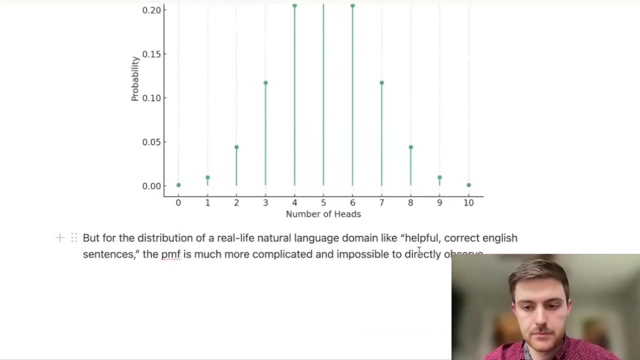 which is what makes language modeling different. They are. you do think of them as probabilities of that event. Great, great explanation. And then the next question is: is this similar to Monte Carlo sampling at all? Yeah, so the way that you could actually arrive at a graph like this would: 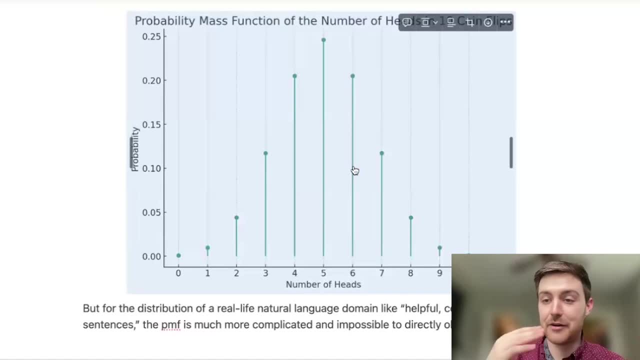 be through you, through Monte Carlo sampling, which would basically just be, you know, flipping, you know computationally or in real life, this set of 10 coins recording the answers and you will see, over time there'll be some noise, but it will converge towards a good estimate of this. 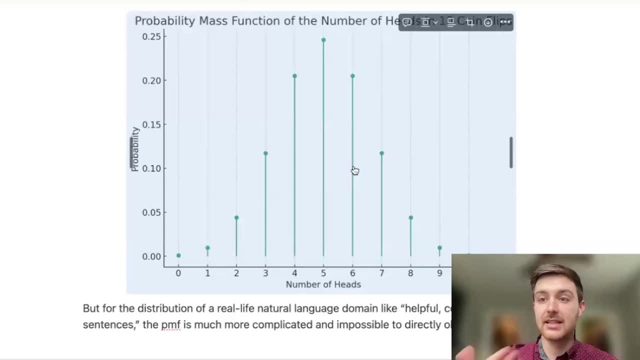 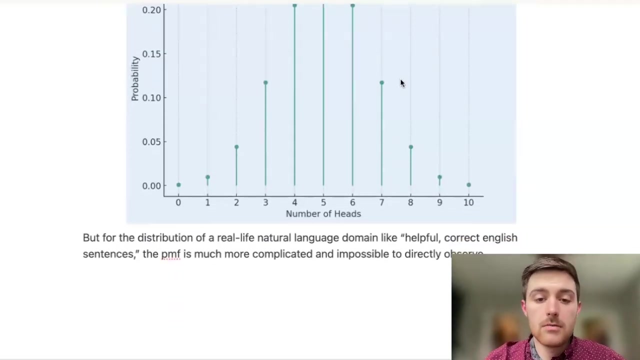 distribution. This distribution also has an analytic solution using, like, the binomial formula that you can derive. but approximating it through Monte Carlo is another good way to get there. Nice, thank you. So what do we as deep learning practitioners do when we have? 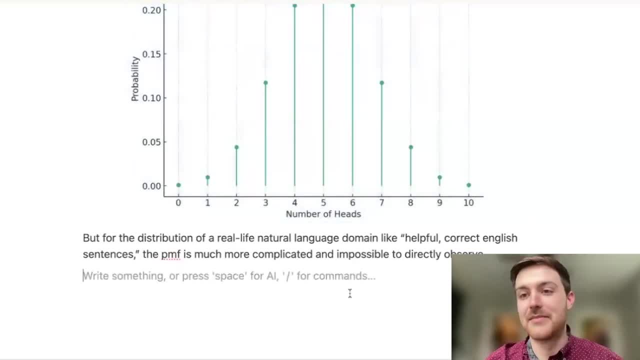 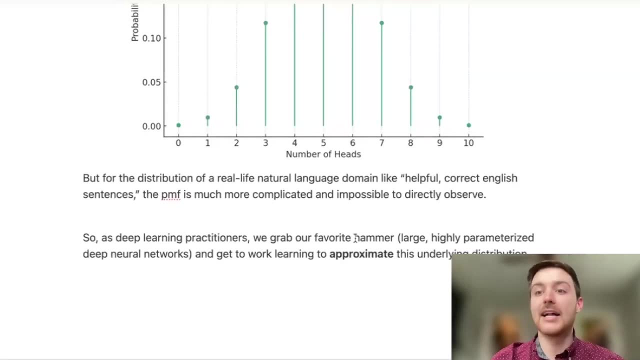 a problem that you know. we're looking to estimate a extremely complex function, while we grab our neural networks and throw a bunch of data from our target population at it and we estimate that function, So we get something that is not a true, exact corollary to that. 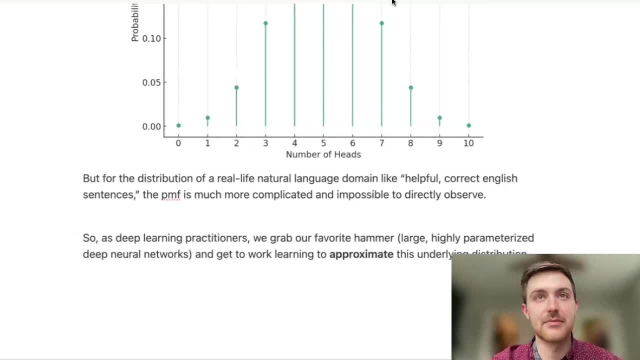 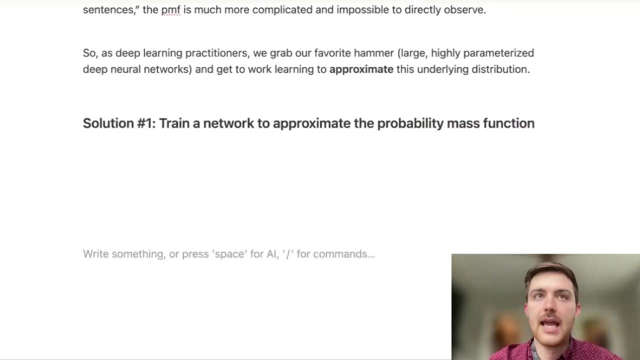 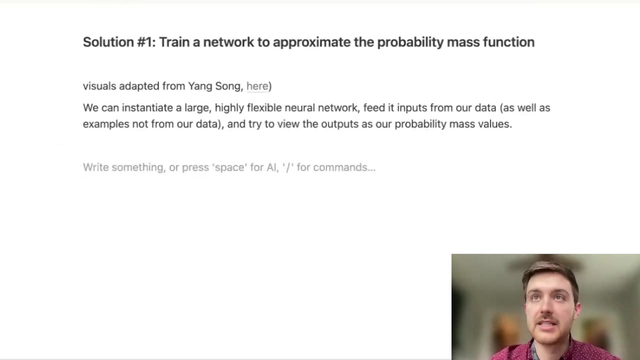 theoretical quantity that doesn't, you know, actually exist and we can't observe. but we train a network to approximate it, And the way that we do this is by instantiating a big network, a bunch of parameters, like I said, feeding in a ton of our data, and we will then be in a world. 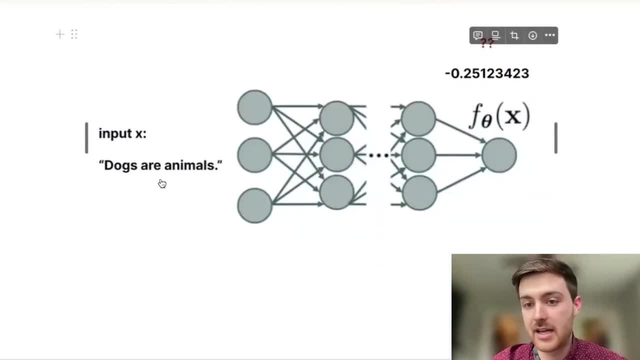 in which we are feeding a sentence into this network- like dogs are animals- and getting out some scalar value right. In this case, we're getting out negative 0.25. And this is kind of a problem because what we would want this to output are our probability. 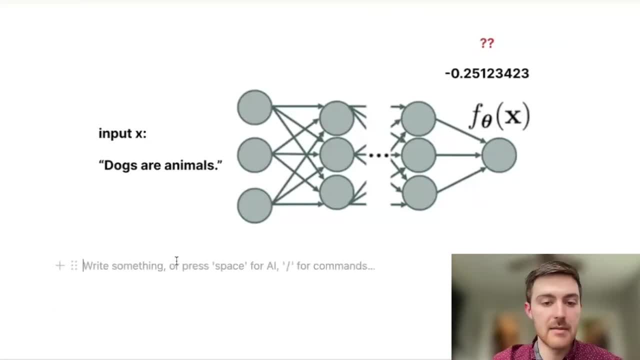 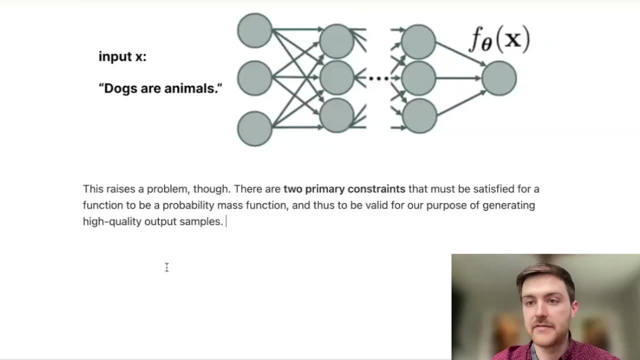 mass values so that we could do the nice stepping towards a more plausible generation that we talked about in the beginning. But probability mass functions and probability density functions have two primary constraints, And those constraints kind of line up with how we think about probability. but there are also requirements for these functions to be valid, and these 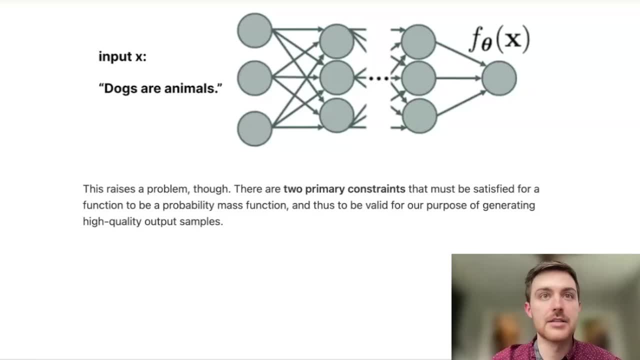 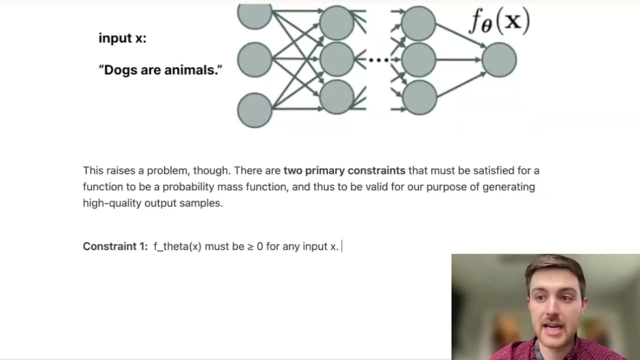 functions to be, you know, useful representations of what we're trying to do under the hood. Constraint number one is that any value in a probability mass function, any output for any given x, must be positive. It must be greater than zero. Sorry, And this is because you know. 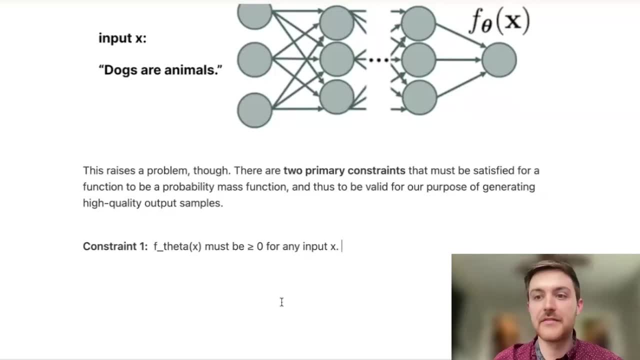 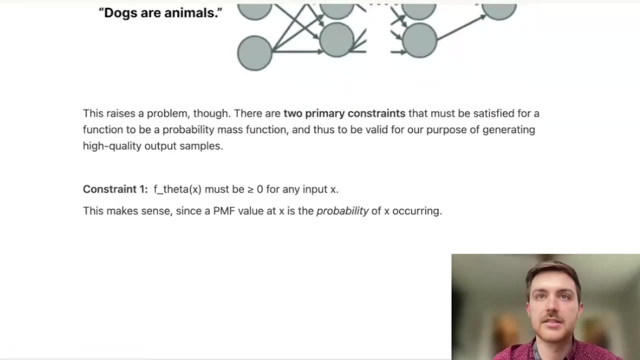 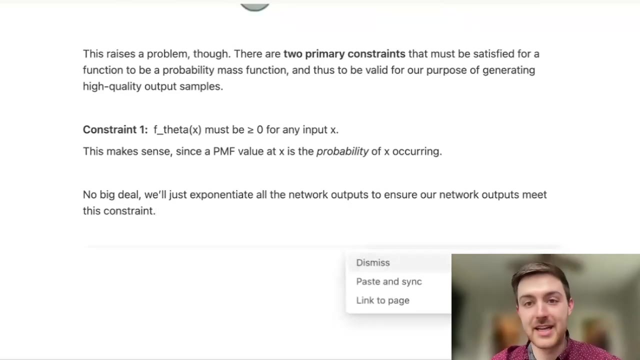 this intuitively makes sense. You can't really have a well-defined concept of a negative probability, And we interpreted the PMF value from earlier as the probability of x occurring. So we have some nice mathematical tools to handle this When we have things that we want to make positive that are not uniformly positive. 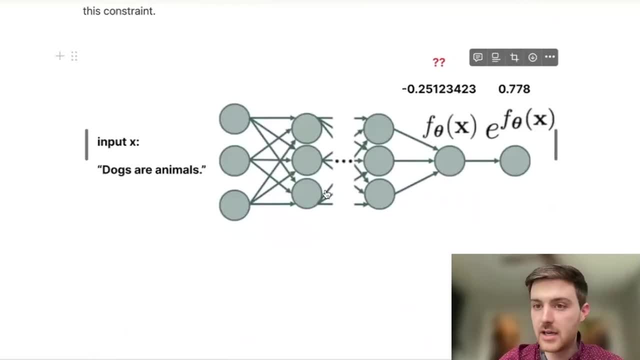 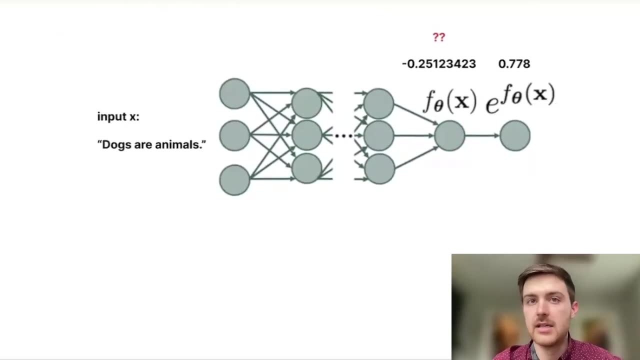 we can exponentiate them. So we've now fixed that constraint. We add an extra check on the end of our network to exponentiate these values And now we have something like 0.778. that kind of fixes our issue with that first constraint for what makes a valid probability mass function. 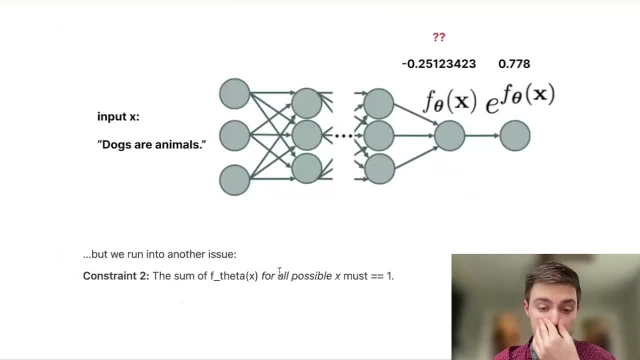 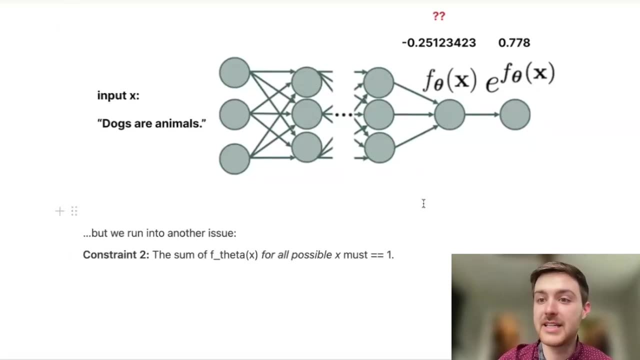 We have another problem, And this is again just how probabilities work- that the sum of that value for all possible x must equal one. This is basically saying the probability of every possible thing happening for a given event has to equal one, which makes sense, And this you know. 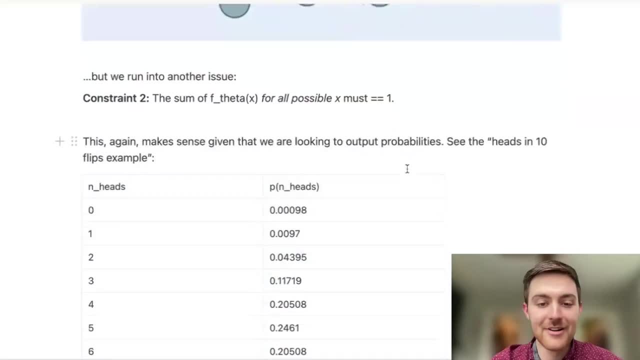 just is an example of that that you don't actually need to look at or you know in-depth, besides the fact that it does sum to one. So this is an example of that that you don't actually need to look at or you know in-depth, besides the fact that it does sum to one. 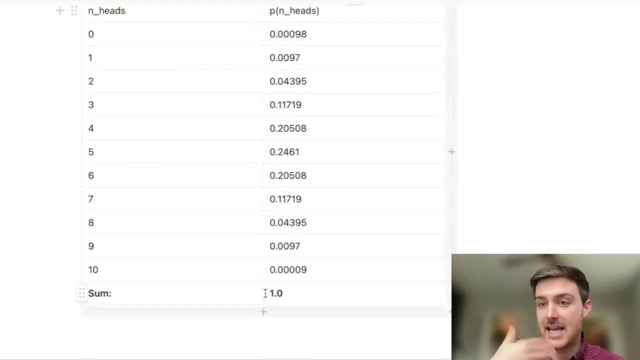 So this is an example of that that you don't actually need to look at or you know in-depth, besides the fact that it does sum to one. This is the distribution of the PMF values for that 10 coin flip event that we defined earlier. 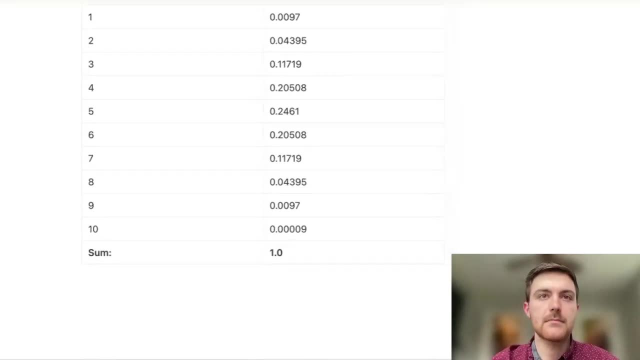 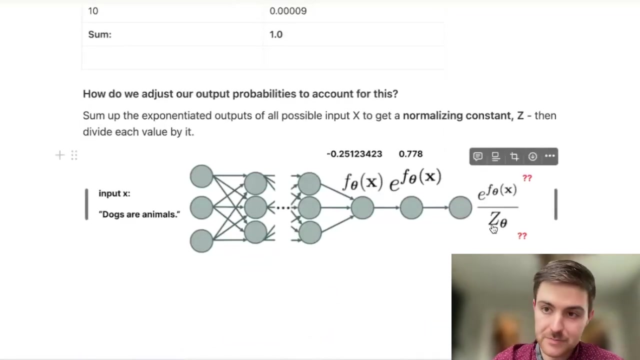 And notice that they all sum up to one. So what math tools do we have in our bag to fix this constraint? The biggest one that I can think of, and that makes a lot of sense, is summing up all of those exponentiated input values to get a normalizing constant that, when 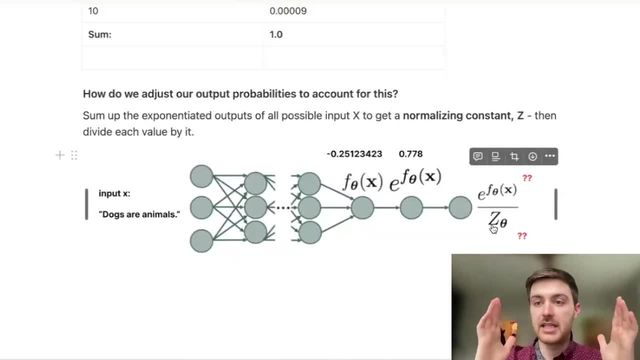 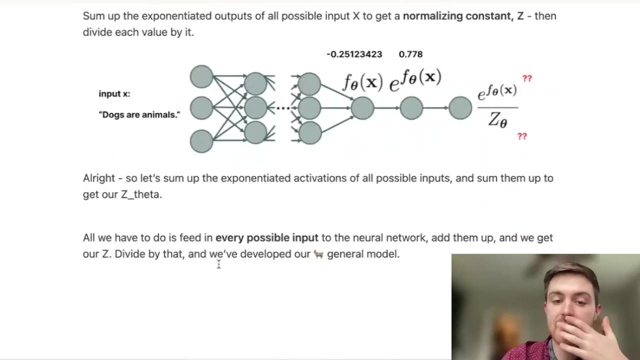 we divide each input value by that constant, it will scale everything down so that the sum is exactly equal to one. So all we have to do in this case to get that model and to be able to properly estimate our density is: sum across every possible input into this neural network, add up the activations after. 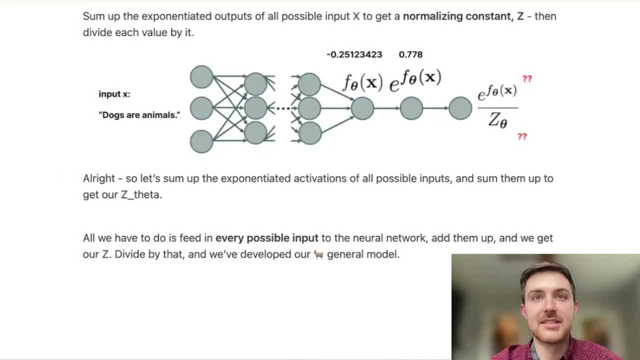 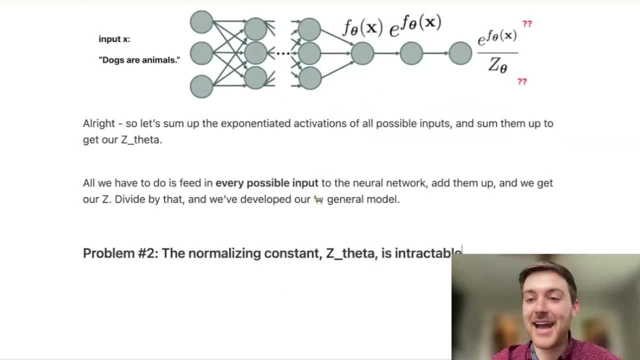 we exponentiate from all of those and then we get our normalizing constant that we can divide by, And we're off to the races from there. Probably know where I'm going with this. That normalizing constant is. I'm going to go ahead and do this. 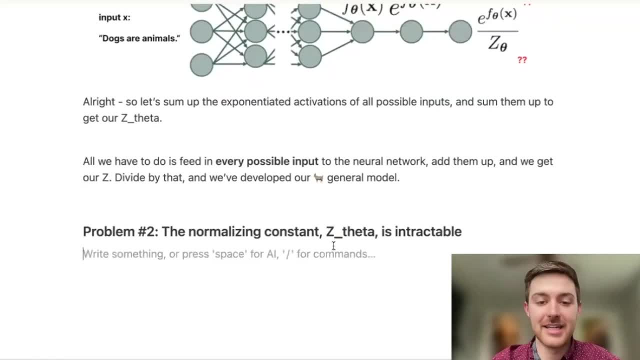 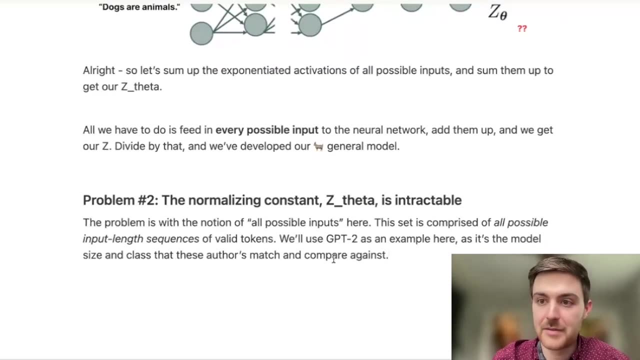 So big. The problem here is this notion of needing to sum up all possible inputs right. That's not too bad for a coin flip. It's not even too bad for 10 coin flips. That's something that we can define and compute. But for a GPT2-sized and input-output structured model, the way that 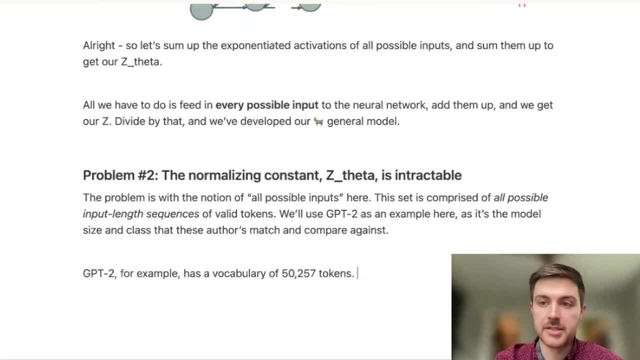 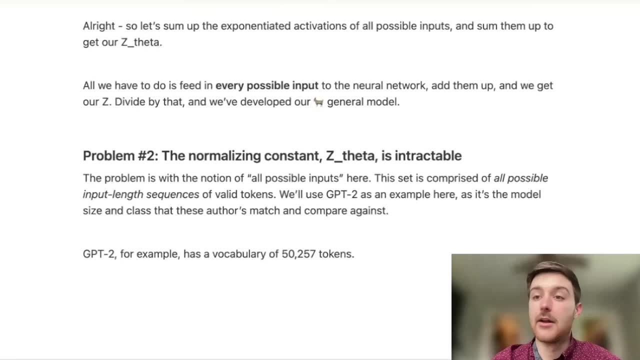 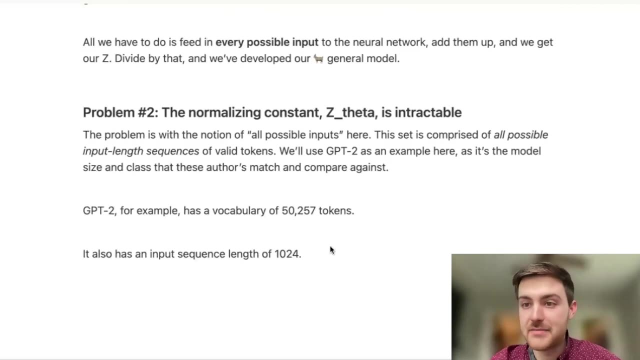 the authors are trying to replicate here. GPT2 and the models used in this paper have a vocabulary of 50,000 different possible tokens that you could put into them in their input sequence, And their input sequence is of length 1,024, right, And tokens can be repeated, right. It's not like we. 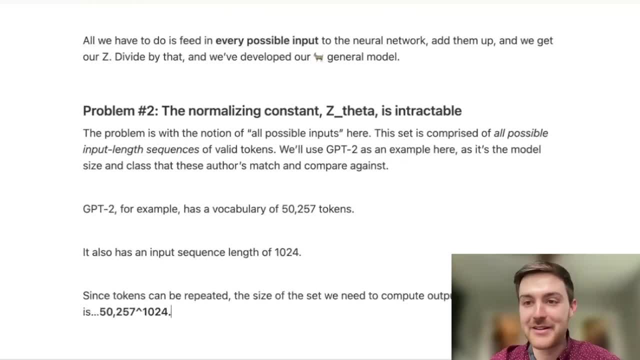 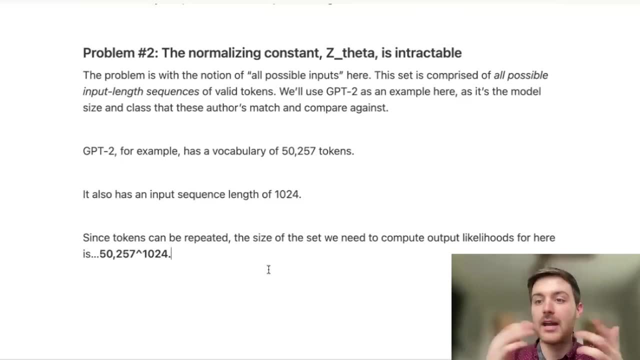 have a 50,000 factorial problem, which would already be a big problem. here It's: we have 50,000 to the 1,024, the number of tokens to the power of the sequence length, That is the raw number of. 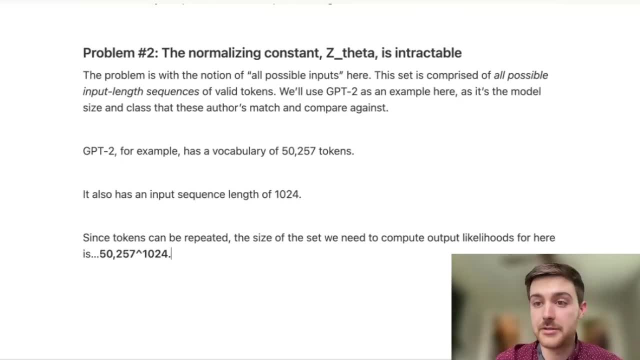 combinations of possible inputs you could have to a GPT2-sized model. The authors said that this is greater than all of the atoms in the universe, and I think it is actually much greater than that quantity, So this is obviously something that we are not going to be able to do. 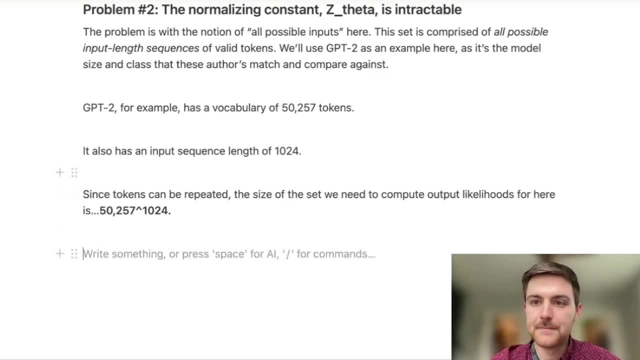 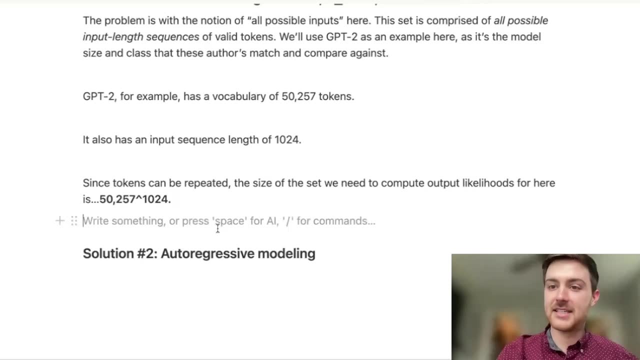 Any questions on that? No, but wow, Big number, Very big number. I started this thinking I was gonna put it and paste it into the document just to show how big it is, and then I realized that would be completely impossible. 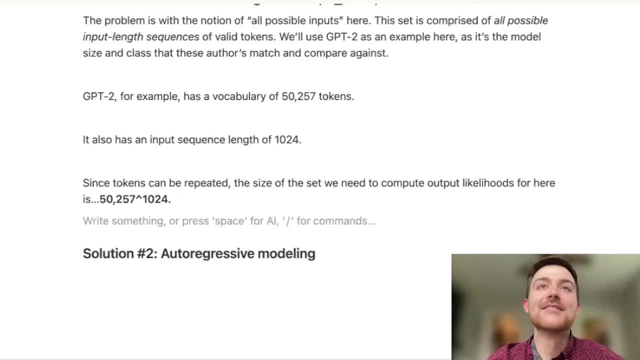 That would have been hilarious, Yeah. So what is the solution to this Right? And this is actually how we arrive at autoregressive modeling. This is a very legitimate and possible solution to this conundrum, And I'll show you why. 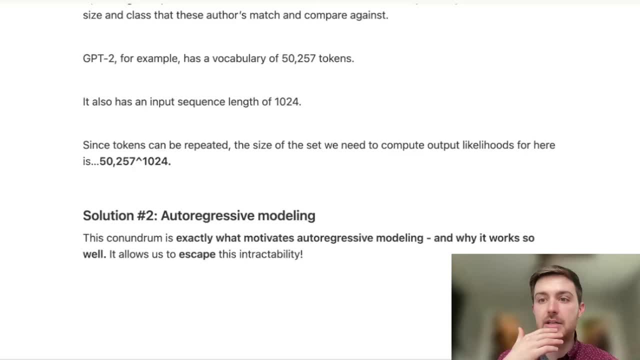 It lets us get out of this intractability. It lets us out of having to deal with- 50,000 times, you know, to that power number of different tokens. So when we do autoregressive modeling, what are we doing? 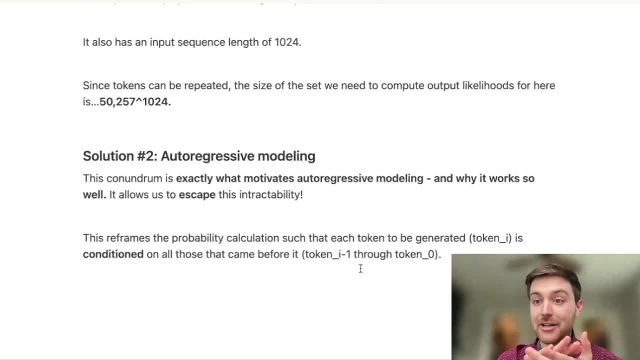 We are reframing the probability calculation such that we are not kind of independently viewing all of those tokens at the same time, the same way that we would in a diffusion model. Instead, we are only concerned about the specific token. we'll call it token I, that is being 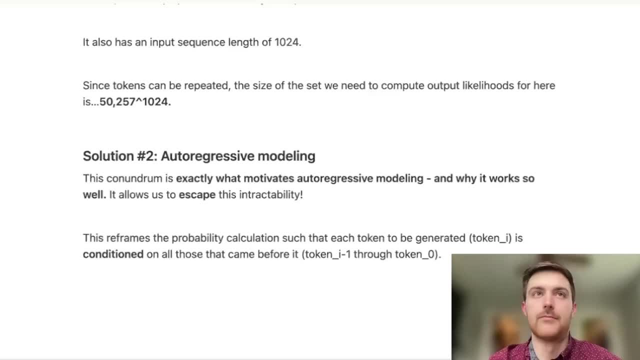 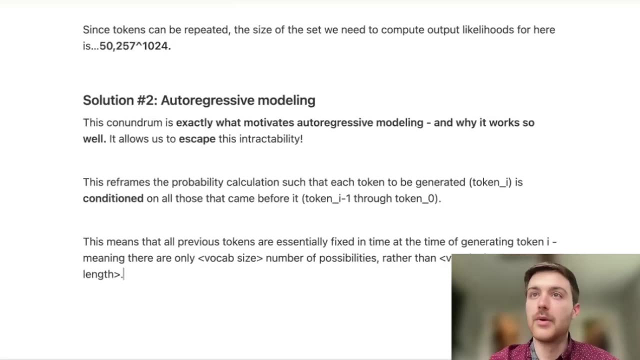 generated, since these are generated one at a time at inference time, right. So this means that all of the previous tokens are fixed right. They're not kind of like degrees of freedom that are varying with the model, And I made a visual for this that is hopefully helpful. 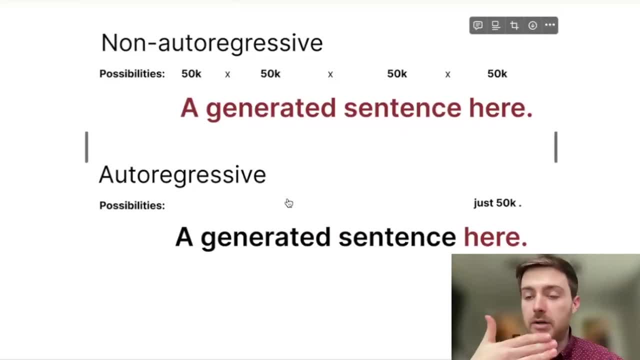 The top is. you know, when we're looking at red words here, these are words that can vary as possible inputs, That's when we're looking to calculate a probability right And in the autoregressive case, any of those words can vary. when we're looking to sum up, 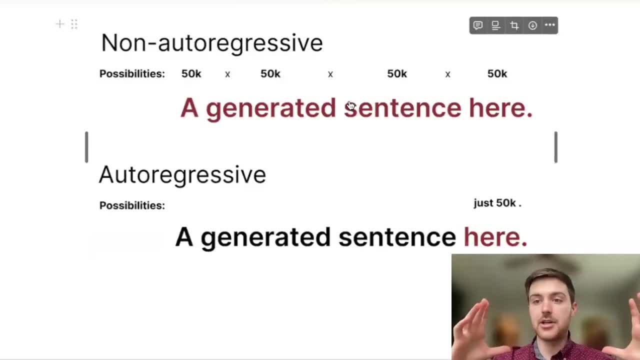 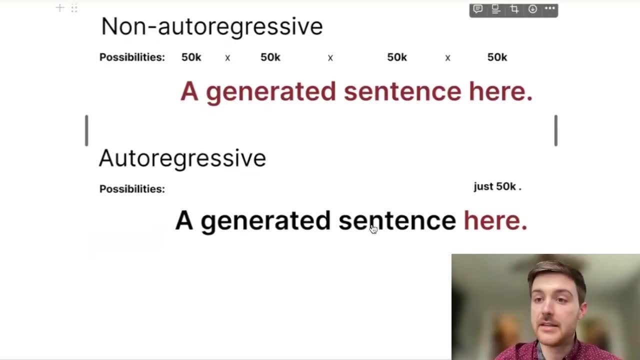 all of the possible inputs for that specific scenario, because we're trying to generate an entire sentence, not one word. So we get 50,000 times 50,000, times 50,000 onto the sequence line In the autoregressive case. we've already generated here the first three words. 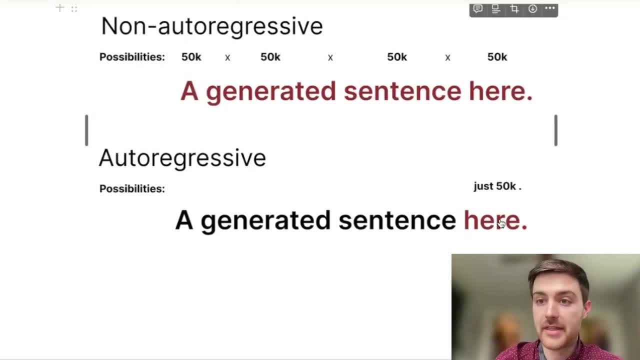 They're notated in black And the last word is the only thing that is going to vary. So the possible options for that are just the total And the last word is the only thing that is going to vary is the token size. So that kind of makes this problem a lot more tractable. 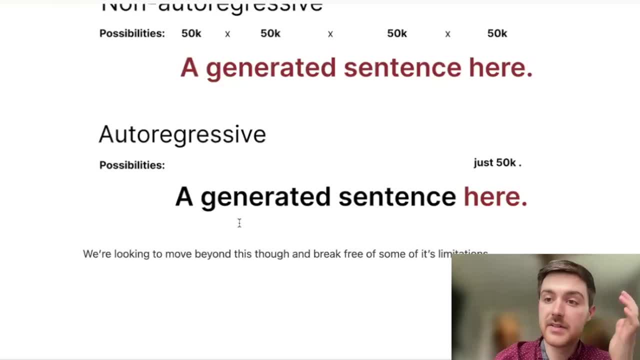 It's a big reason, Whoops. It's a big reason why it has had so much success so far. but because of the limitations that we mentioned around um, you know just the inherent constraints posed by left to right generation- we are actively looking to move beyond that. 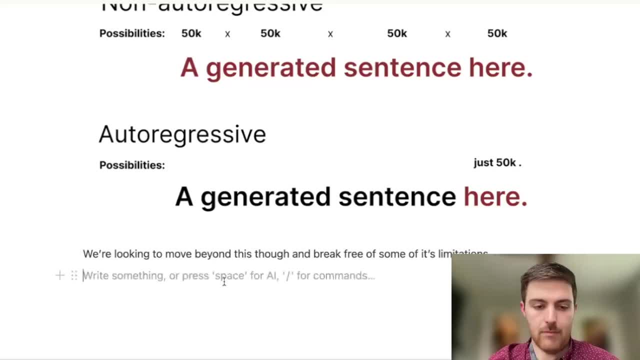 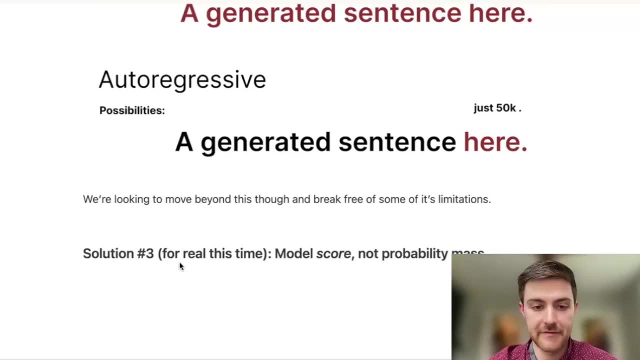 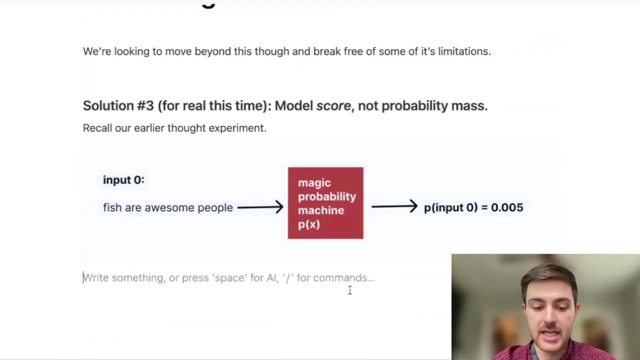 Um, and that's what this paper is all about. The solution that we will actually use is modeling something called score rather than the probability mass It's self, and I will motivate this. going back to our experiment from earlier, Remember our magic probability machine. we get outputs from this and we see which direction we want to take a step in right. 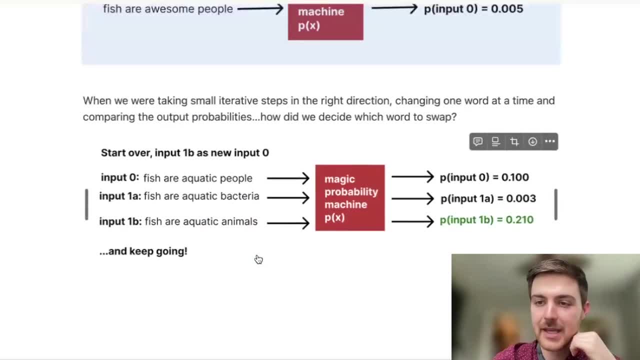 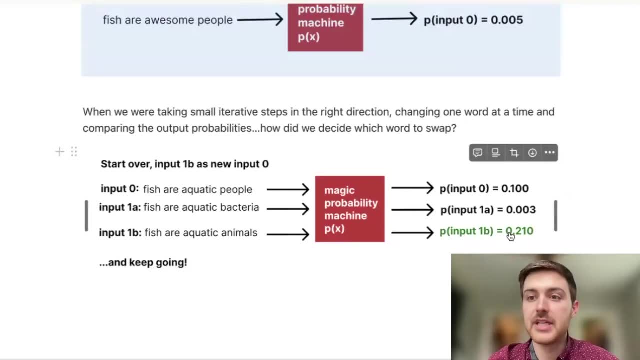 Well, how we want our sentences to be more like going forward, Um, but if you notice this, what is important here is not actually, uh, the raw values. right, We don't need to know that the probability of this is 0.2, 1, 0,. excuse me, 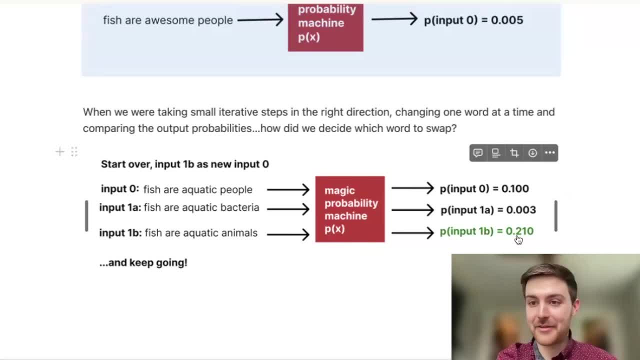 We need to know that the probability of it is more than the other things. So we're much more concerned about the directionality in which we need to go um to have a more probable sentence than the actual value of that probable sentence. We're not interested in the actual value. 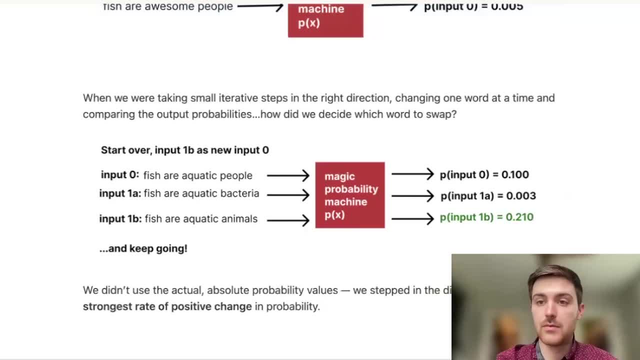 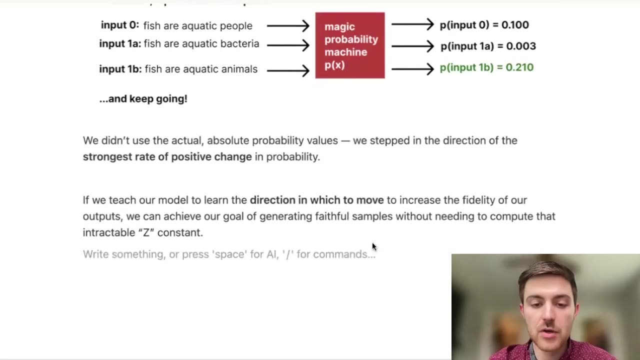 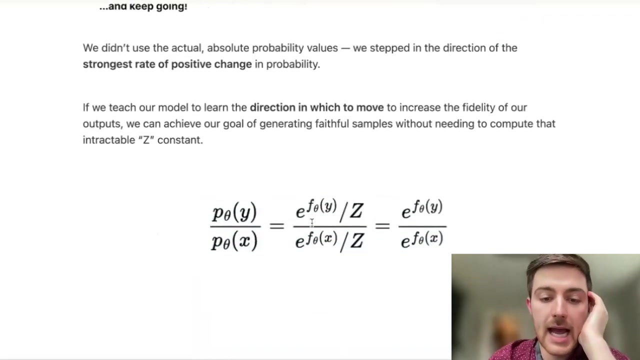 We're interested in stepping in the right direction, wherever that might be. So we can formulate this mathematically and say that we are, like I said, we're, interested in the direction in which we should move. So we can think about, rather than looking at one of these scores in isolation, like the probability of input one B, we can look at the ratio of those scores to each other. 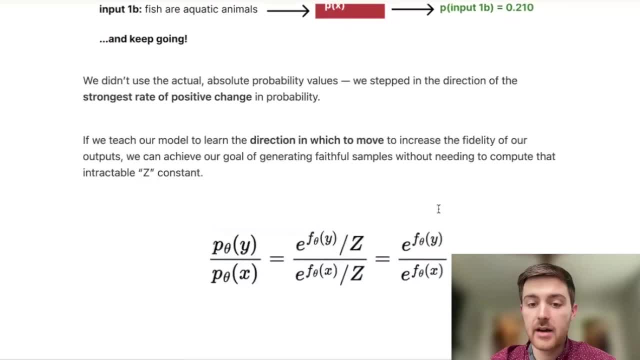 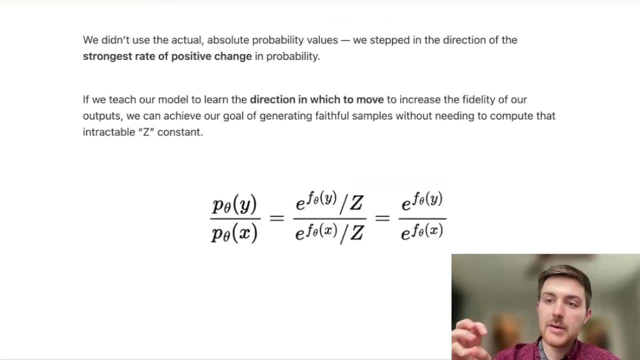 So, for example, the ratio of score one B to two, that of score zero. this then forms a quantity that we can call the, that is called the concrete score, And if we're able to model this quantity, this ratio, throughout our network, you can see that this is something that's automatically a lot more tractable, because when you divide these two together, 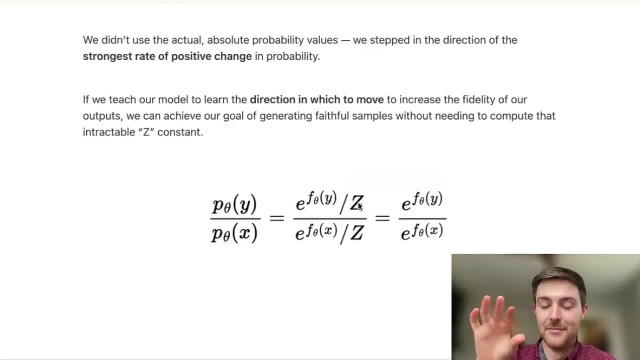 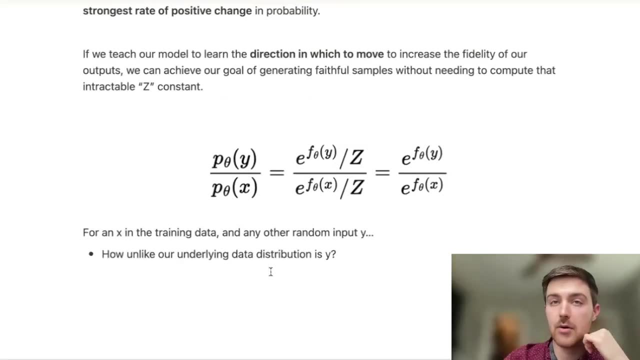 That big Z number that was ruining our lives, uh, gets canceled out. So all we really need to find out is for any observation in our training data. take some other random input- Y- like we did up here with our Y zeros, and we don't need to understand what's the probability of that Y versus what's the probability of that X. 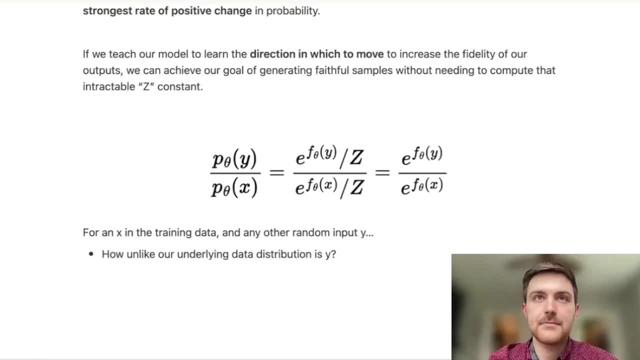 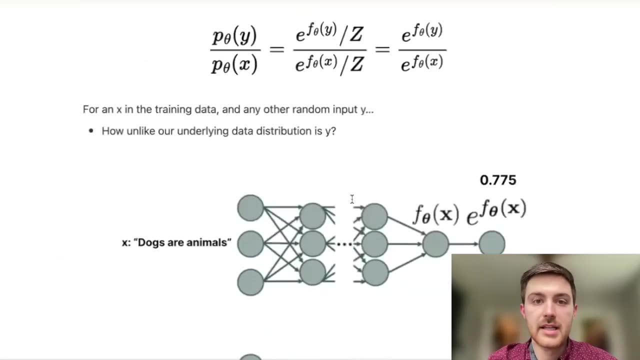 We just need to understand the relation of those two. Cool, I have an example of modeling this with our networks to understand, Right, What a concrete score actually looks like and kind of the direction that they're pointing. So here we're, calculating those three things, right? 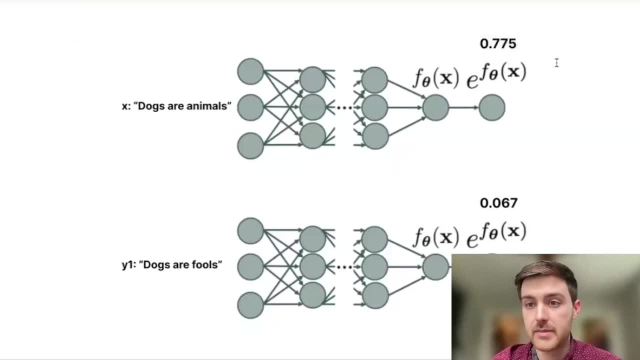 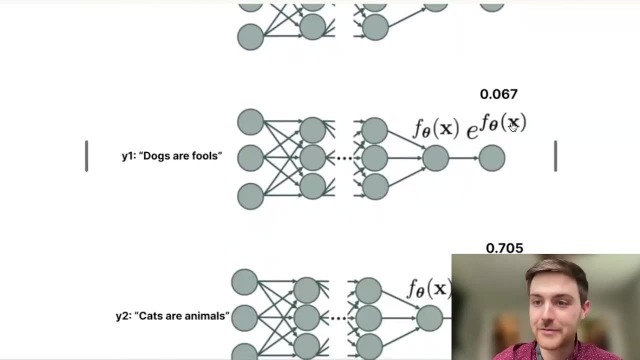 Dogs are animals. Let's say purely like: gets us an activation. That's again not a valid probability of 0.775.. Dogs are fools, I mean. maybe you know what I mean. I don't think so, Right. 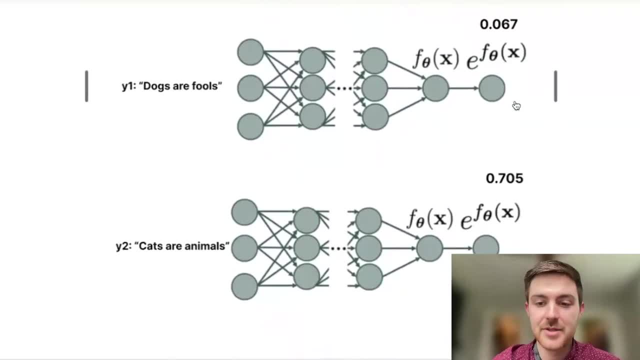 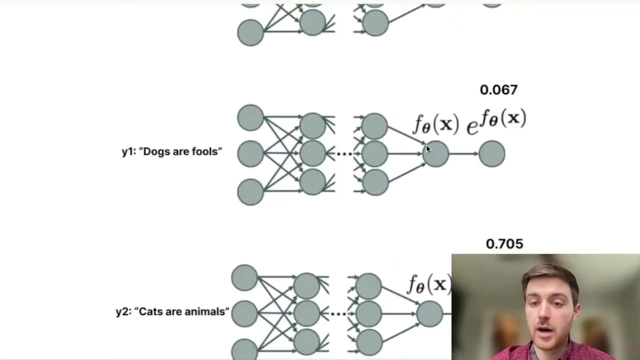 That gets us something that's much less, much less plausible in our underlying data distribution. Cats are animals. That is pretty plausible, right? So if we look at the concrete score, the concrete score of X with regard to Y, one is going to be pretty. 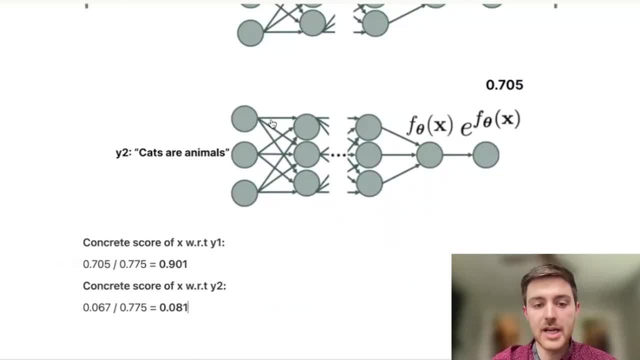 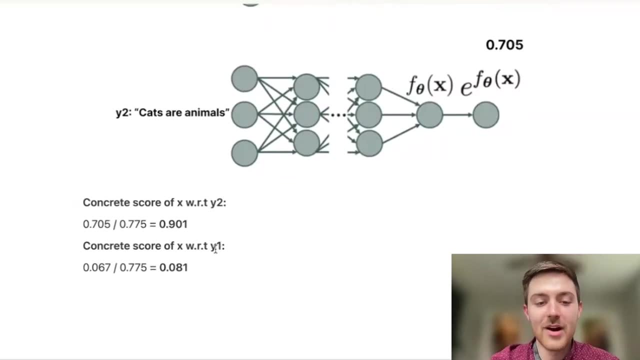 Close to one right. Saying why is basic, why, why or sorry, why. two down here is basically as plausible as Y one, And you'll notice I have the numbers flipped so I'm going to put them back. Whereas you know the dogs are fools. sentence is: you can see through this low, concrete score, much less possible. 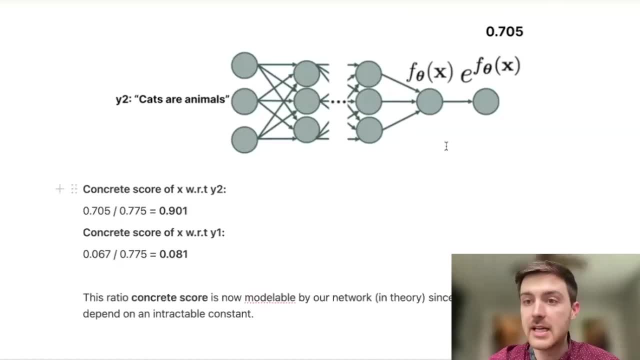 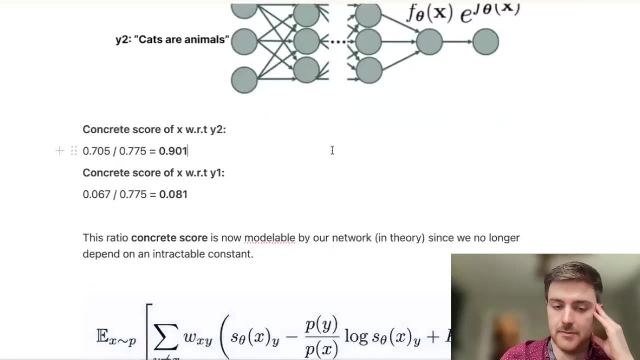 And, like I said, the big deal with this is that this is a quantity that we can actually optimize for in our network, because we no longer have a big intractable constant. So we can Formulate this into a loss function, which the researchers do. 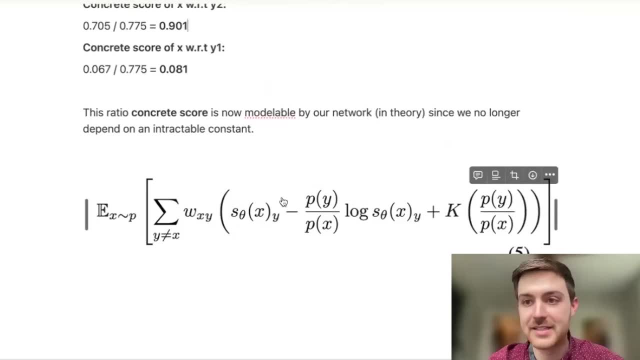 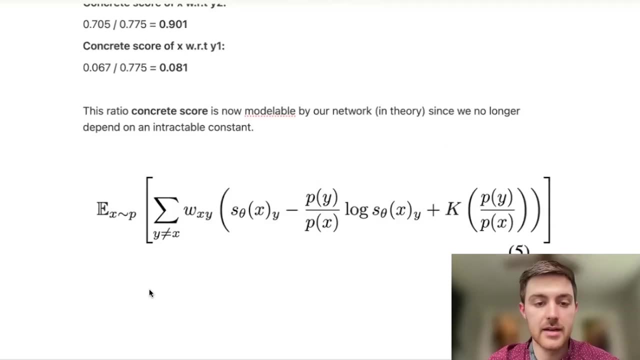 This is what the um, the uh, the loss that the paper is named for, the score entropy loss, And there's a lot going on here. I'm happy to take questions on the parameters, but I kind of typed out some intuition for it as well. 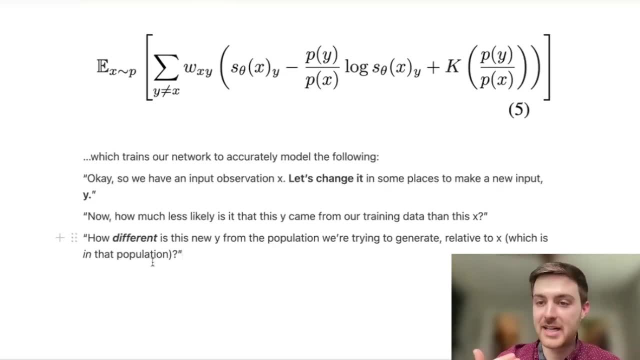 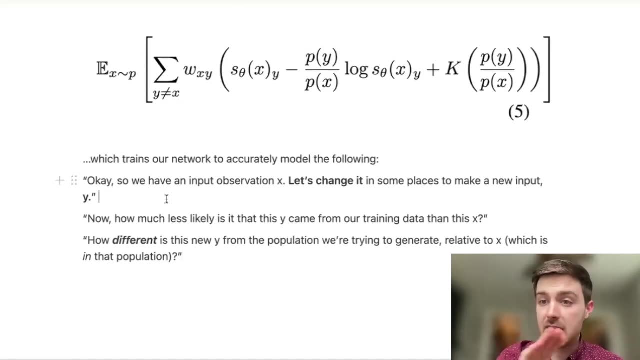 Remember, when you're having a loss, function you. that is something that you want to minimize. It points you in in the kind of right direction as you work on minimizing that. Um, so what we're looking to model in our network is we have an input. observation X: 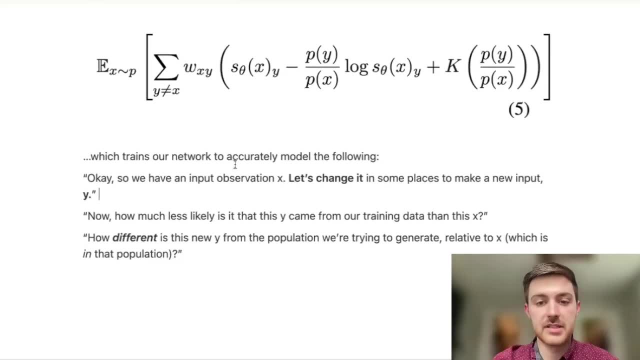 We have A bunch of changes to it, a bunch of wise that we've considered. that are new inputs And we want to understand which of those inputs make X, make the new kind of uh, according to our network, are much less likely to have come from our data distribution. 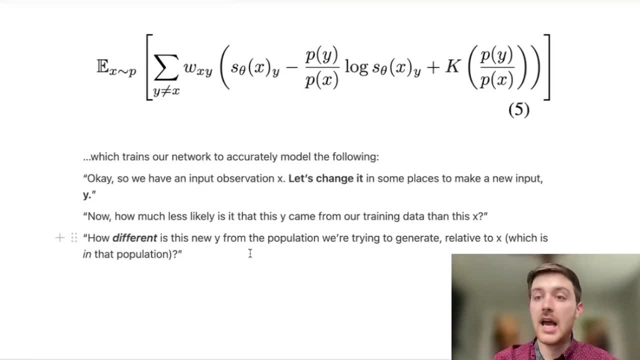 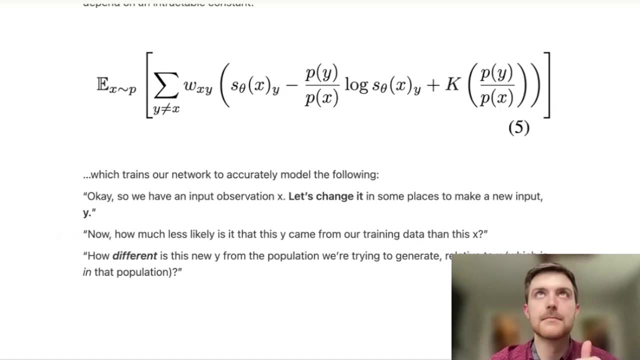 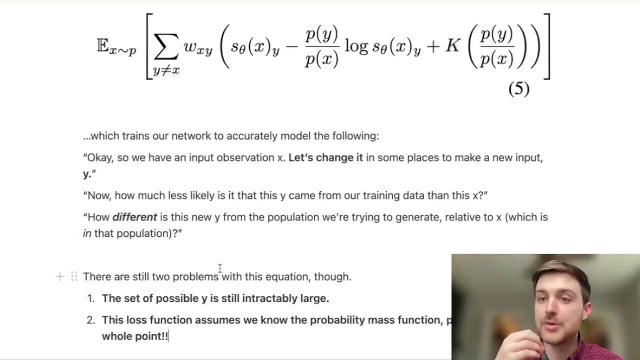 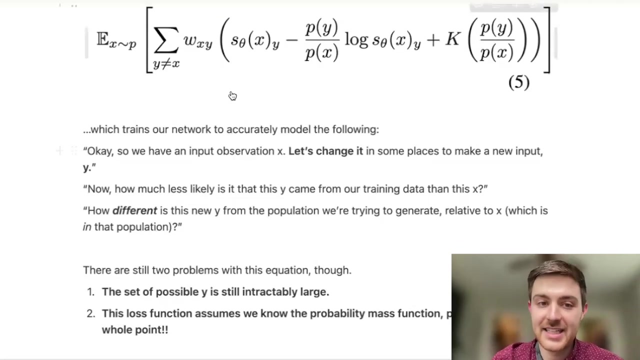 Like dogs are fools or dogs are broccoli or whatever, and which ones are kind of steps in the right direction. Does that make sense? Yep, Cool. There are two final problems with this uh model. Um, all you have to do is ask, or, if you have this, if you've used network based or. 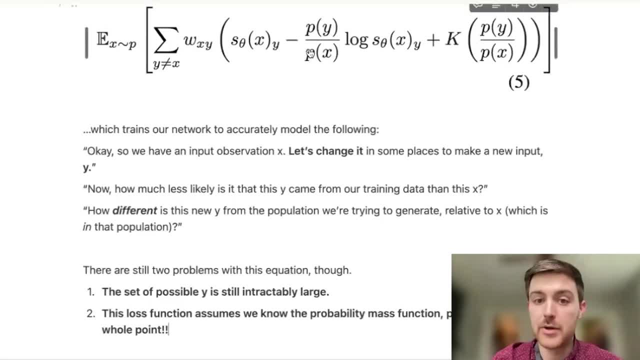 linear analysis, one, you know, Y would be probably more accurate than Y is, And you're right, This is a bit of a way of dealing with the the this problem that we're in, and the problem that we're struggling with, is that we just need to subtract the Y from the input X, and that is a very useful way. 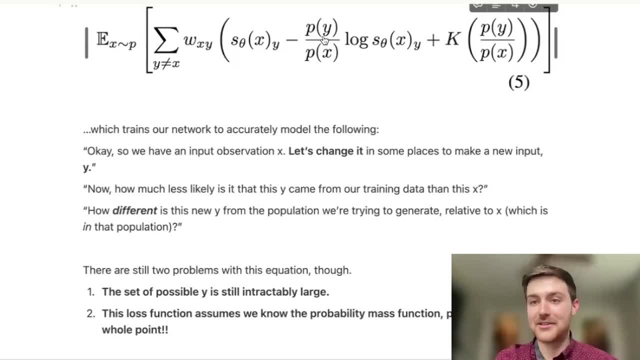 The problem is that I can't calculate the Y from the input X. I can't do the equation. In other words, we aren't able to do it at the engine Sounds like And I don't have that. Okay, This is a creative approach. 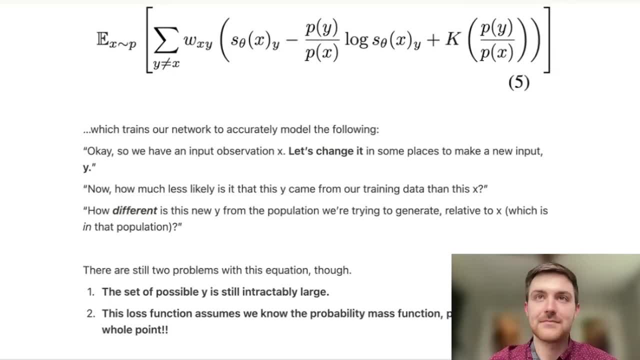 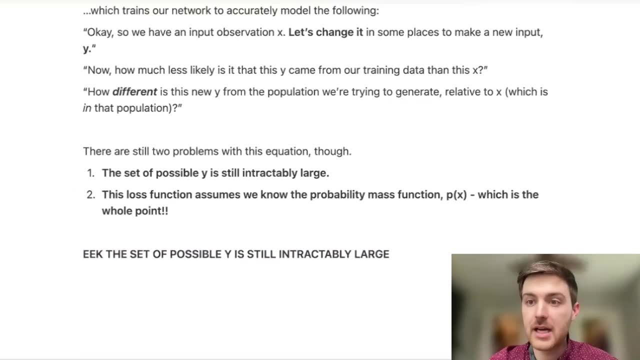 So we need some other way to estimate that. On the first piece the set of the possible y is still very, very large, because y here is defined for each x as every possible input. that is not x. So this is a slightly better number than we had before. 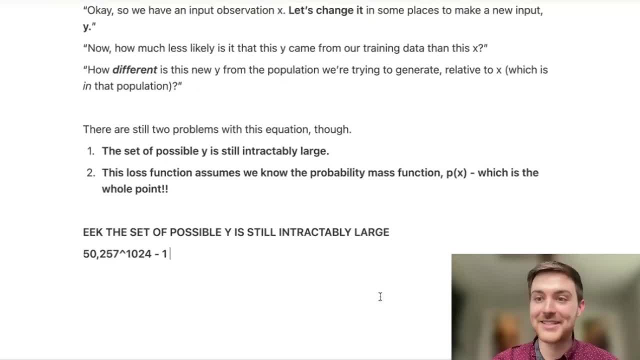 This is now 5,257 to the 1,024 minus 1, because x is excluded. But we also have to calculate an x number of times. That's obviously not going to work. So what we do, or what the authors do, sorry- is they restrict this instead of all possible. 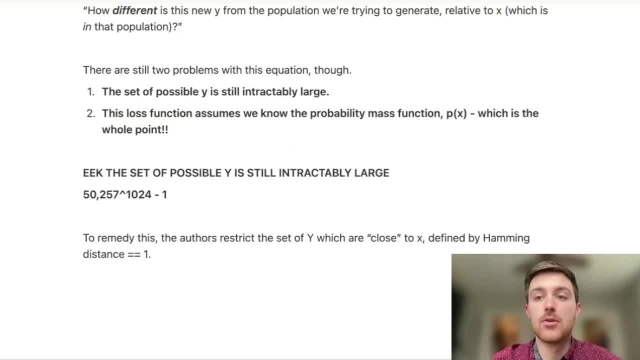 y that are not equal to x. they restrict it to all possible y that are close to x, And they define this by having a Hamming distance of 1, Hamming distance being the number of tokens that are different from the original sequence. 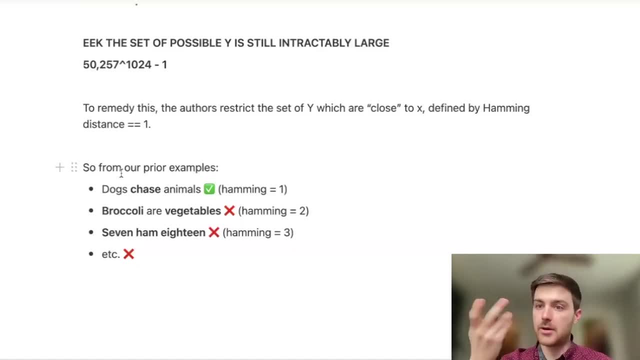 So the possible set of y, which are neighbors in graph theory of x, includes dogs, chase animals, but does not include broccoli or vegetables because that has a Hamming distance of 2 or 7, Hamming 18,, which has a Hamming distance of 3.. 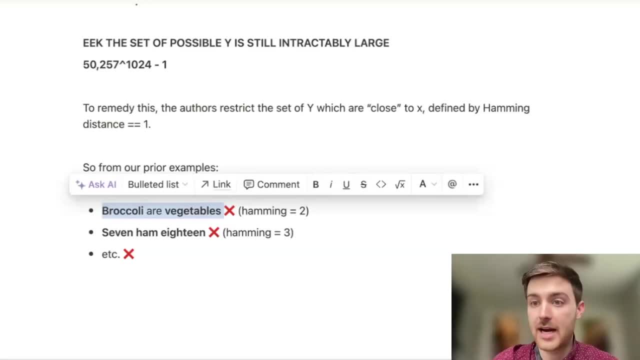 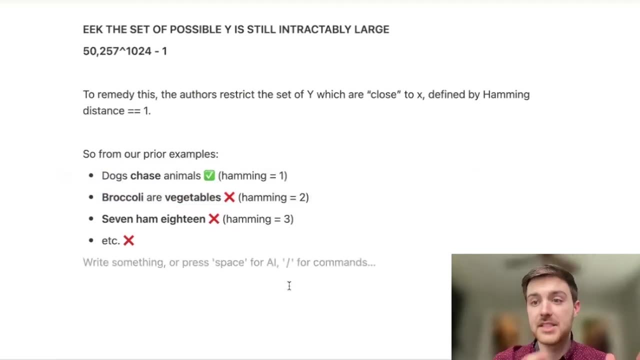 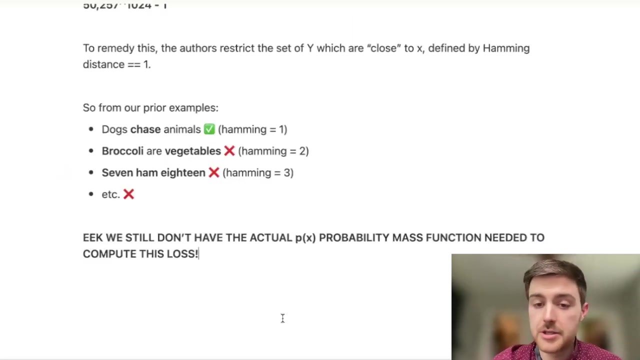 So that reduces our scope, And in a kind of future practical dive where we go over the actual code implementation behind this, we will talk about some further optimizations that allow us to kind of work with that still large number even more effectively. Second big issue is that we don't have that p of x probability mass function. 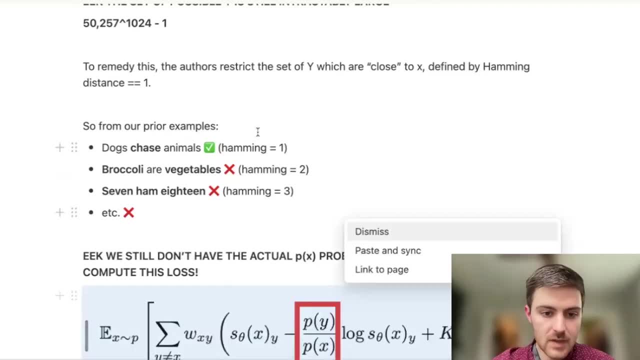 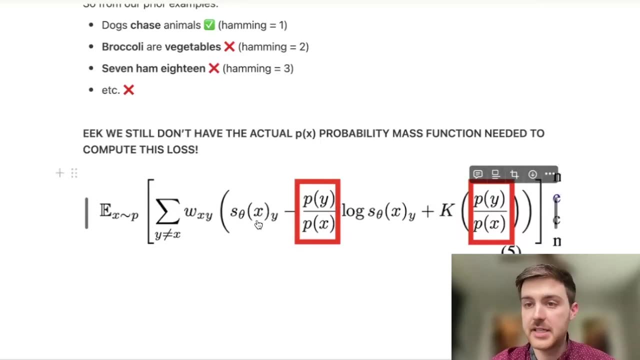 And if you see here when we are, you know this is kind of the golden quantity that we're looking to estimate. this s? theta of x here is the value through our network. So as part of this loss function we get the value through our network. we compare it to. 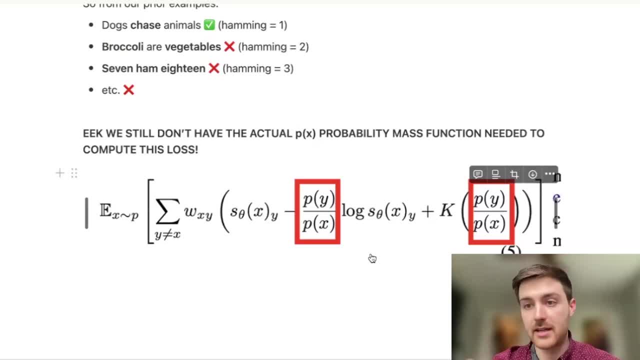 the ground truth value, which is p of y over p of x, and penalize it in various ways. But we don't have the ability to check our work with that function because p of y, you know, the function that gives us p of y or p of x- is our magical black box. 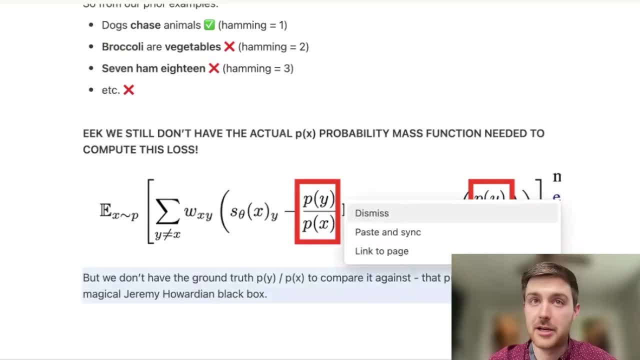 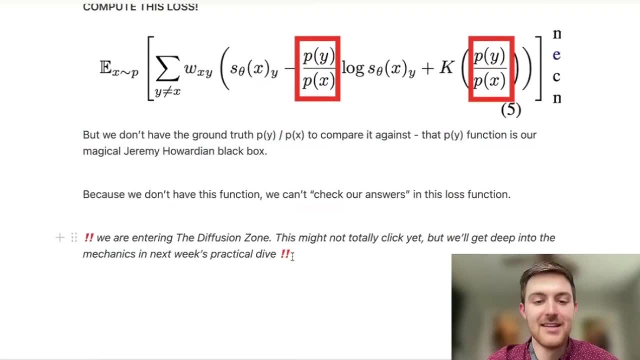 So we don't have the key through which to check our answers, And that is why we end up turning to a diffusion process, which we have now arrived at, And this is where the math gets a little crazy. Um, again, we'll be kind of elucidated further through actually digging into the 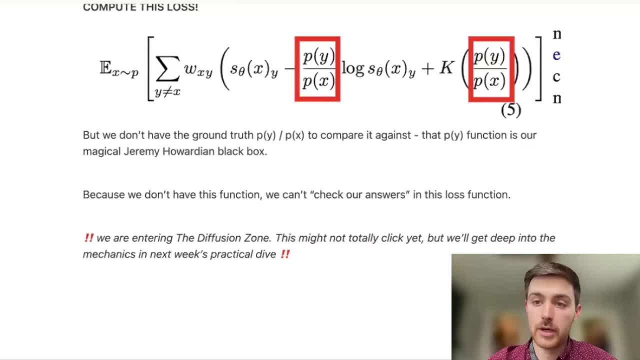 code in a future practical with I've, which I'm really excited for, Um, but we're going to give some intuition today for, uh, what adding diffusion noise does and then how that's actually executed by the researchers and what advantages it gives us in the output. 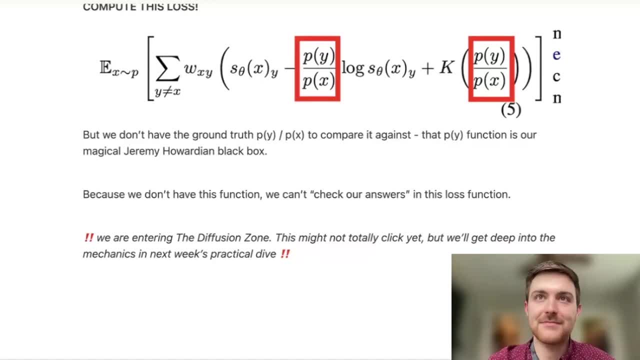 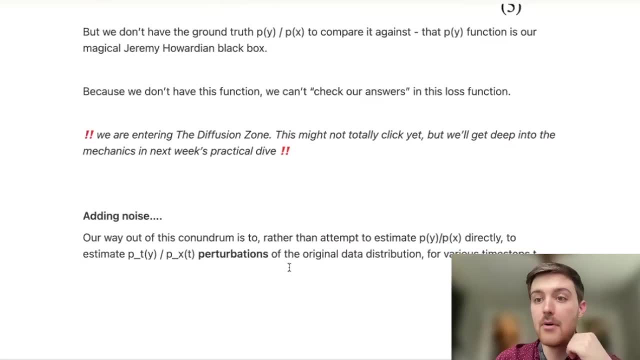 So we were entering the diffusion zone. So we can't estimate those probabilities directly that p function right, Cause we don't know them. but what we can do is add some noise to that probability distribution, random noise that we know and we control right. 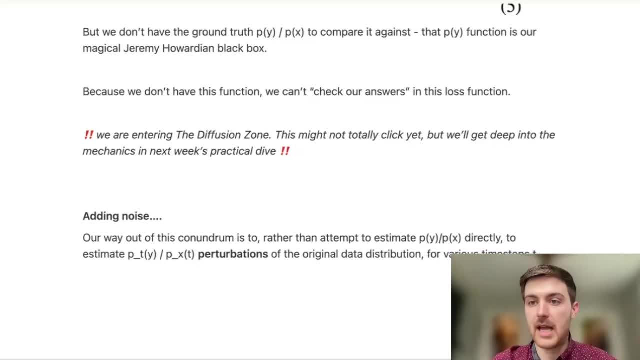 And that makes a new distribution that we are able to reason about and we are able to optimize for and we are able to learn those concrete score ratios. So we have a distribution that we don't understand. We add noise to it And now we don't fully understand that distribution, but we know that there is a 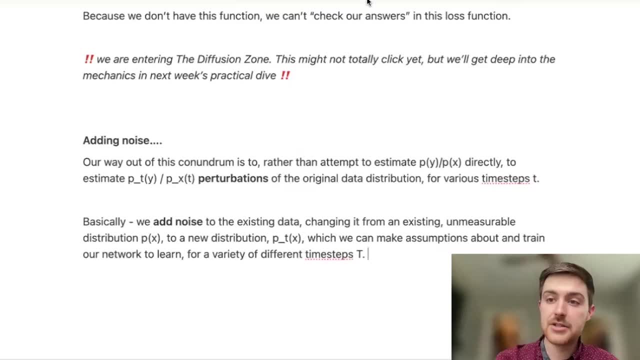 part of that. that is, noise that we have added, and we can teach the model to be able to, for a given time, step T um understand how much noise was added and predict the noise that was added, because if we can do that, we can then subtract. 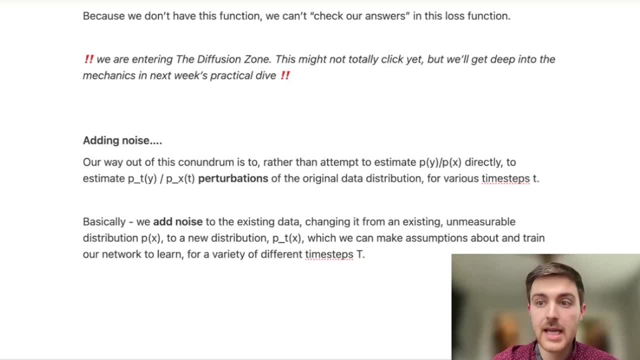 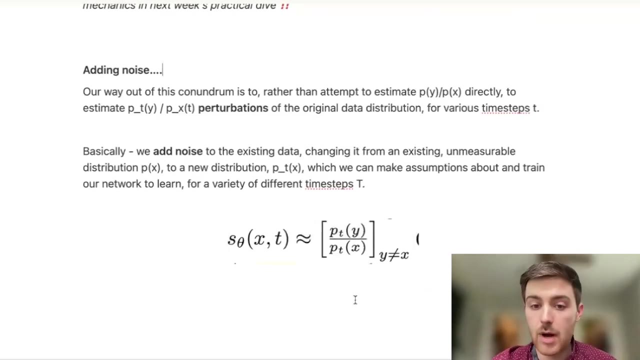 the noise out, just like we do in uh diffusion for image modeling, and iteratively step our way towards a less and less noisy- uh you know- chunk of texture. So, instead of optimizing for and learning what we were showing earlier as that P of Y. 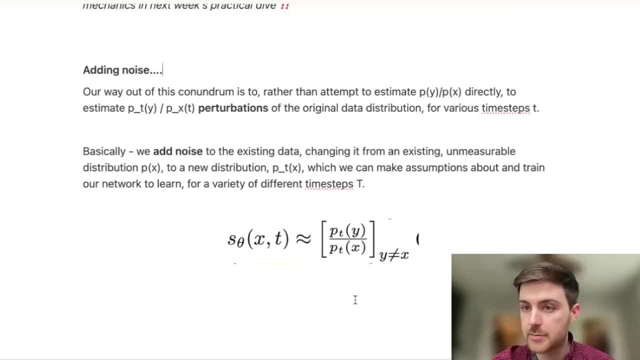 over P of X, which is the true probability in the underlying data distribution. we are learning the PT of Y and PT of X for a bunch of T's that we introduce, which are different timestamps, And you can think of them as different amounts of noise that are being able being added to. 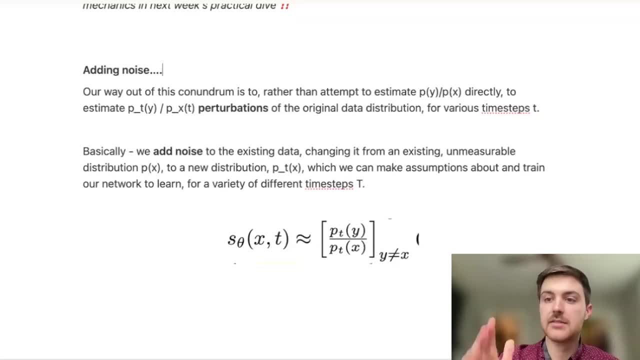 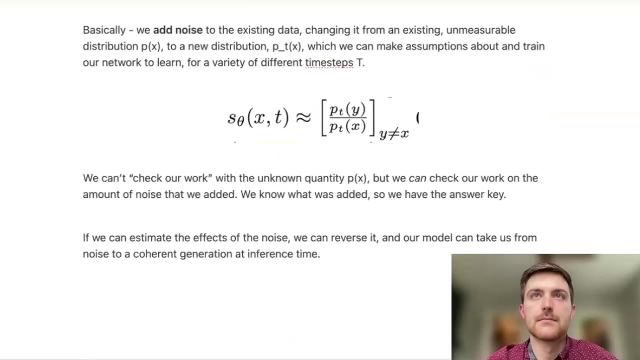 the data right And if we're able to learn these, we can facilitate that backward step, uh, which we're going to show in a second here, but any questions up until this point? Okay, That is where we leave most of the math behind and get into the actual kind of implementation. 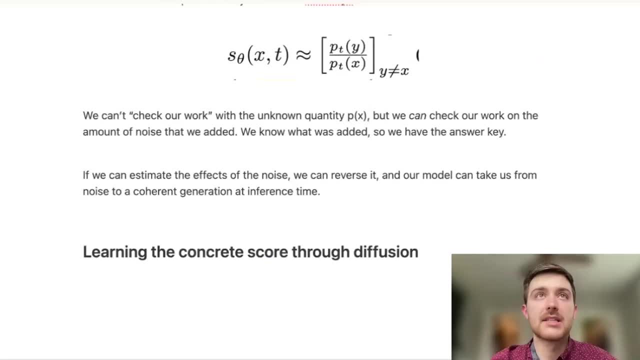 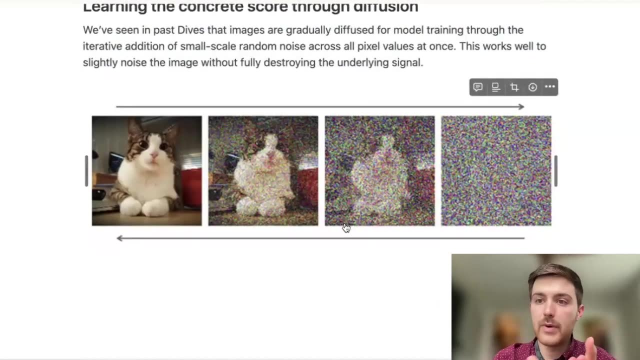 of the diffusion process, which I think is very cool. So in past dives we have talked about, uh, diffusion work in imagery and in video, And the way that we add this noise to the distribution of our images, the way that we 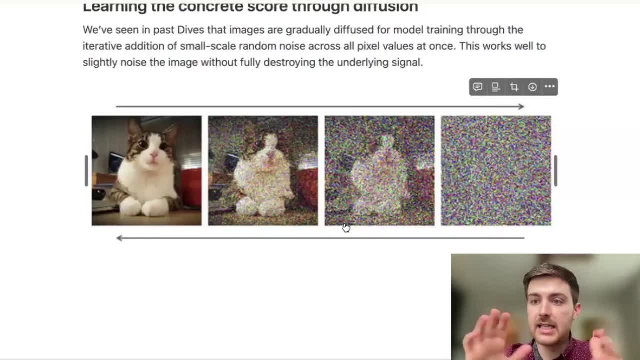 noise, our training data, so that we can learn how to uh do this. You un-noise. it is by kind of simultaneously, you know, applying some random change to each pixel in the underlying image, And when you do that to this cat here, you apply a little bit of that noise. 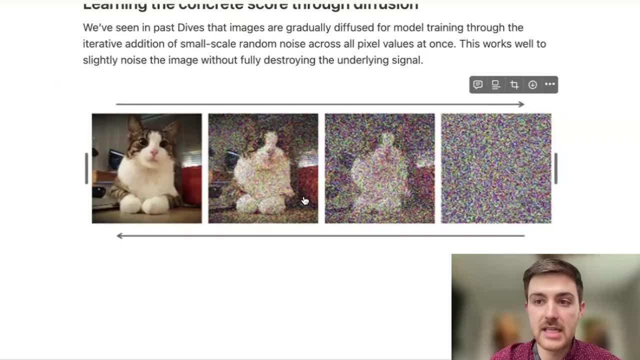 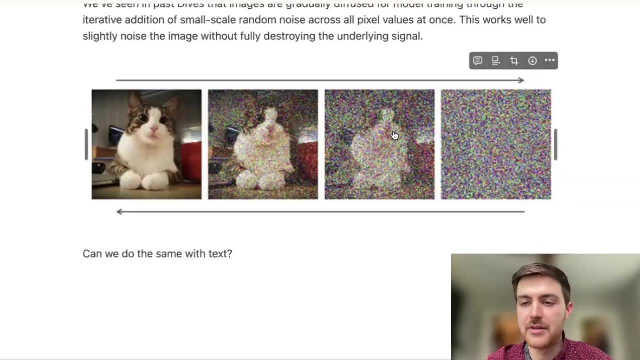 It's still recognizably a cap right. There's still signal in the image that you can detect and that you would be able to train a model to reverse, And the authors had this question of you know, can we do the same thing with text? 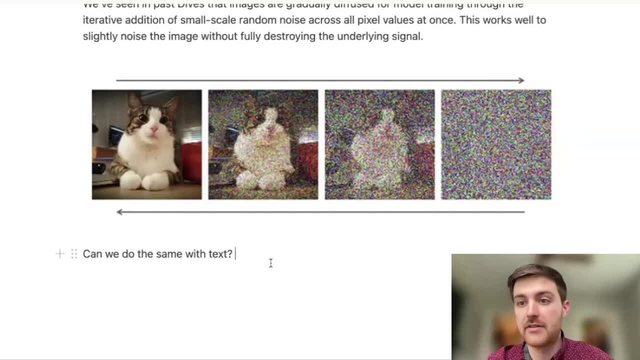 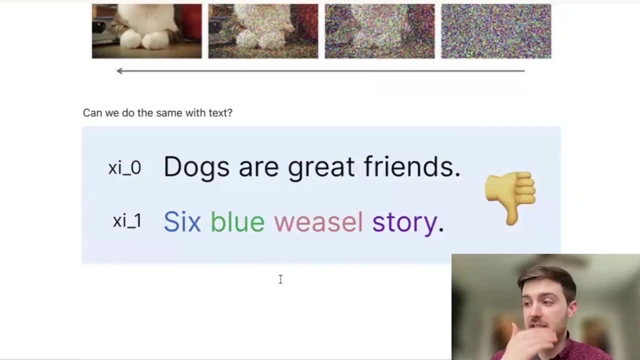 right. Can we jitter every token instead of every pixel, have it flip to some other pixel? And they argue: And it makes total sense. Uh, no, you can't, because since we're dealing with discrete data instead of continuous data, when you jitter these things all at once, you are losing all of the signal. 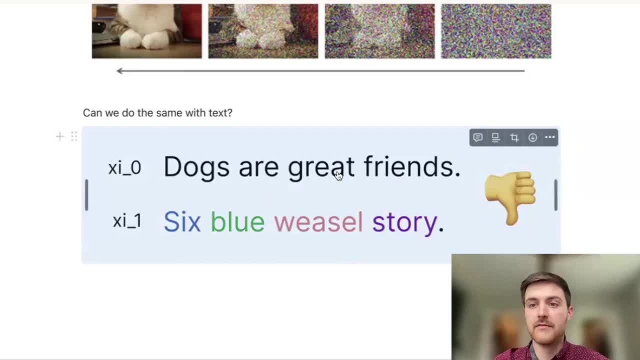 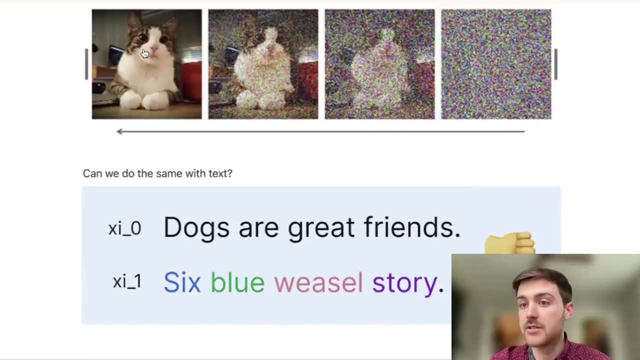 It's being destroyed immediately, right, There's nothing that we can recover from this initial sentence about how dogs are great friends. uh, that is still left in this. in this six blue weasel story, It's like we went from this first image of the cat directly to the last image, without 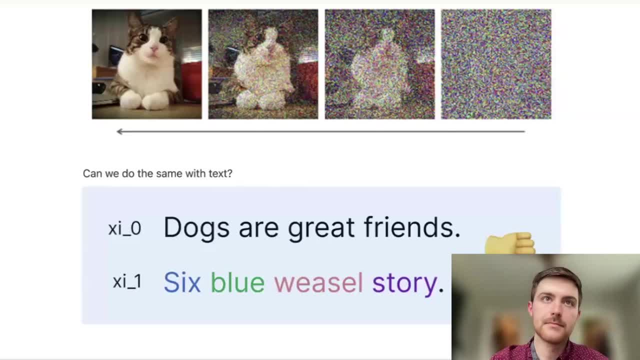 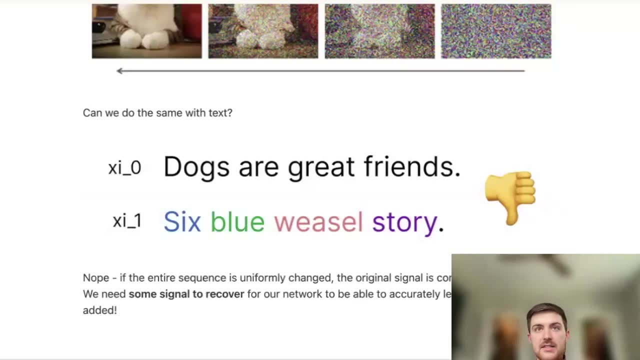 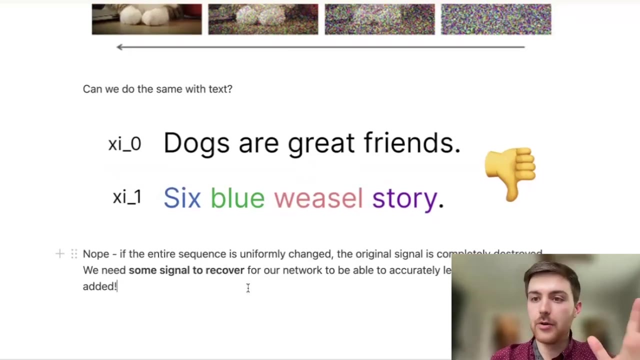 these crucial intermediary steps. So we need to leave some signal For our network to be able to learn to recover that. again, this is a problem with the discreteness of text. So what the authors do, instead of changing everything at once, is kind of set each token. 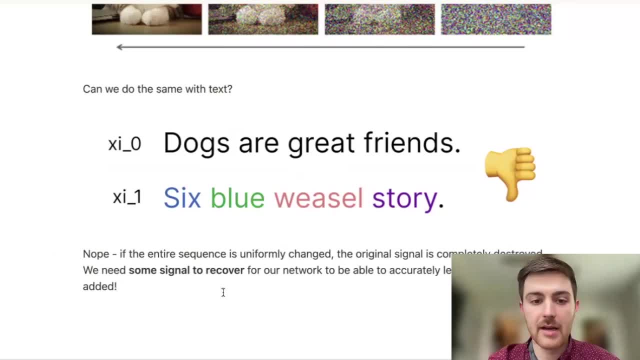 on a timer, to you know, flip to some other token independently, So these are not all going to happen at the same time. This is a process, a continuous process, that they let run over time and they sample from it um at various timestamps along that process to get those various T distributions that 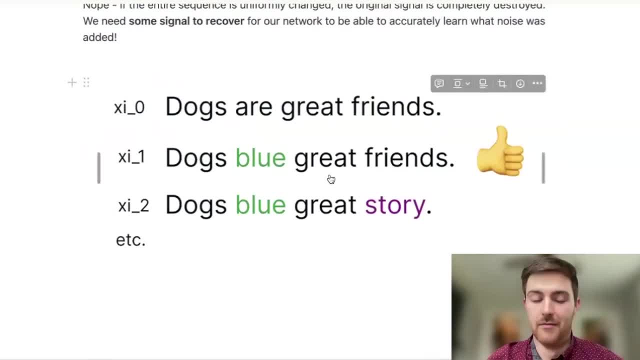 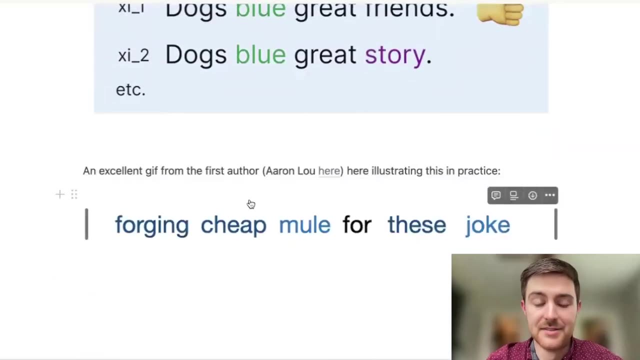 they will predict. And um, this is My take on it. You can see that we are iteratively adding this noise, not just immediately changing you know one thing in every place and then destroying the entirety of the signal. Um, but the author, the first author on a really awesome blog post, um, has a uh. 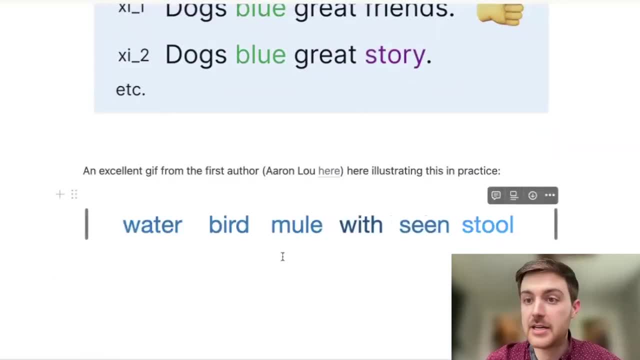 illustration of this. you know how this kind of goes: from an initial sentence that you see in all black to just progressively more and more destroyed, but each token flipping independently, so that there is still signal in those intermediate steps. I wonder and I don't. 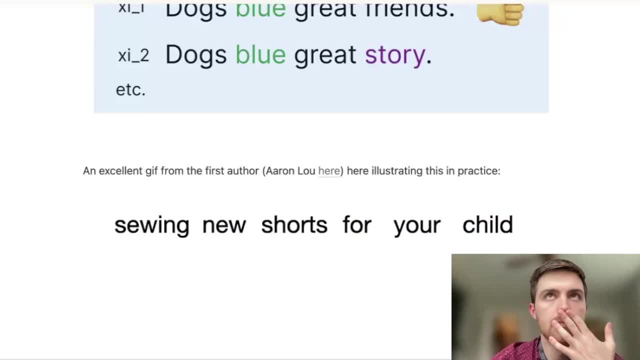 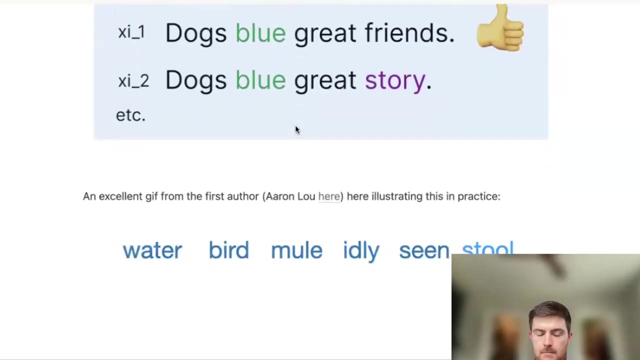 Remember if they talk about this at all. but like, even those flips are destroying a lot of noise, like cause it's discreet and you could flip blue to uh dog or something like that, It feels like it could be interesting to even perturb in the embedding space itself. rather, 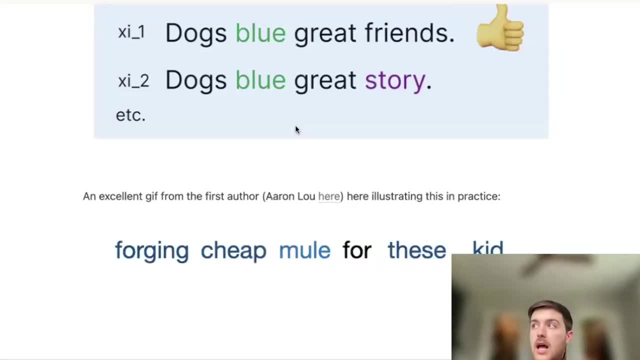 than the indices. Did they talk about that at all? Uh, I saw some previous work that was talking about. like you know, this is really one of the first uh like really highly performance discreet diffusion models, like operating purely just on those. 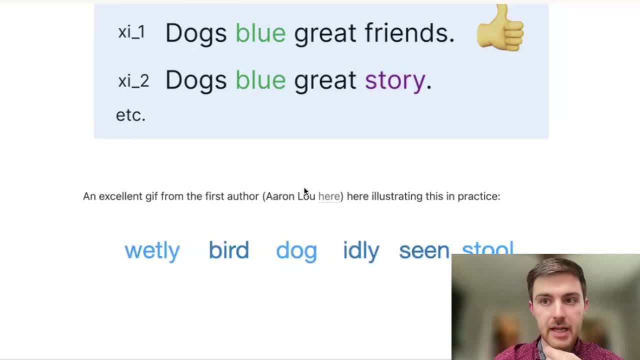 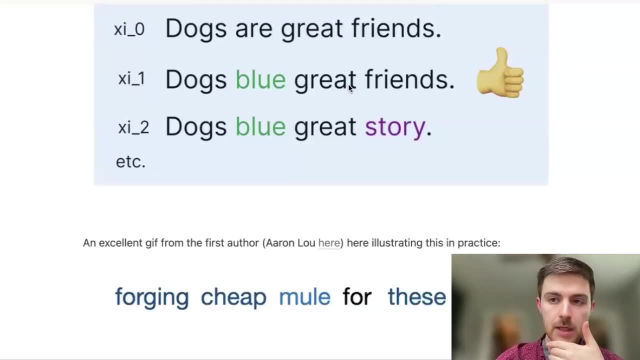 tokens, But there were, I believe, attempts at doing it continuously, And I would think that that that would be how they do it, Cause you're right, If you want to make a small perturbation from, dogs are great friends, you, the smallest. 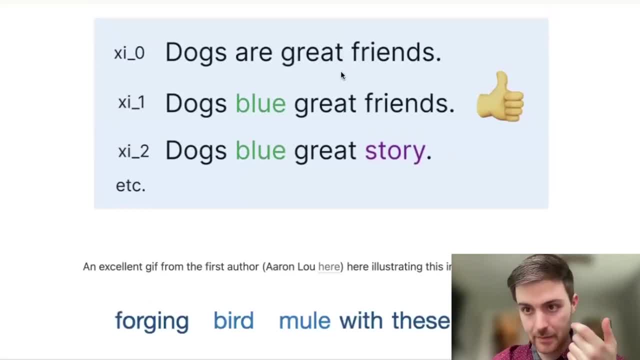 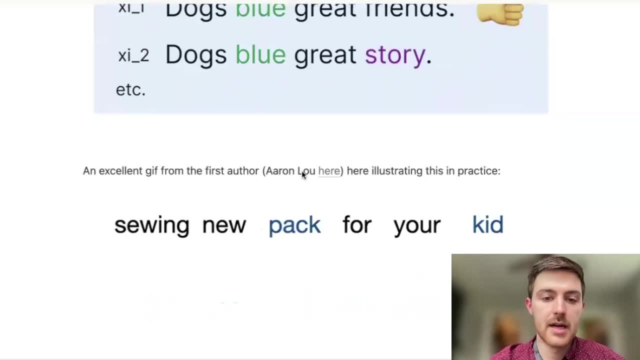 possible perturbation would not be what the authors do, which is, you know, randomly flip one. The smallest would be to change to a similar work, change great to good, change friends to buddies, or something like that. So I think that's a really good point. 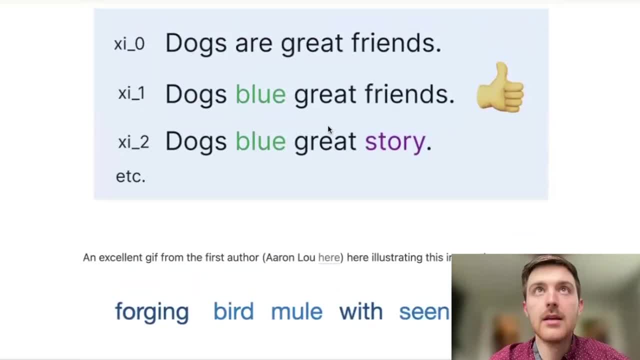 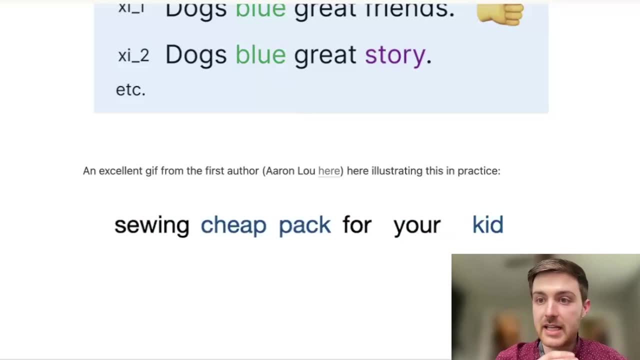 Totally Okay. So this you know kind of is is a nice like you can kind of think of it as a data augmentation process, right? So we're kind of creating these derived versions of our training data and then we lean learn. 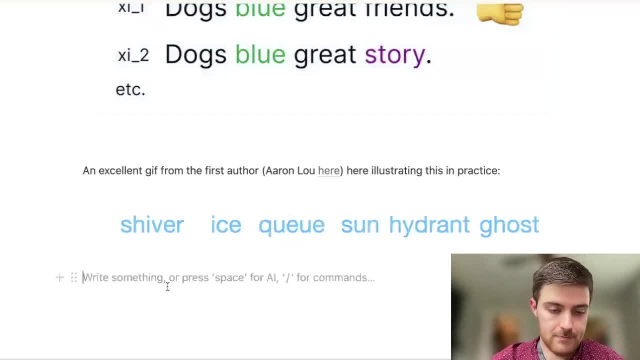 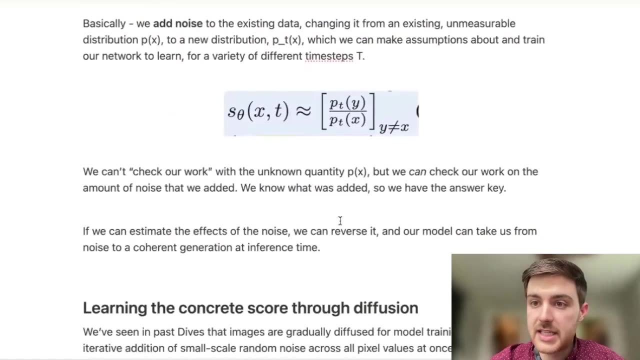 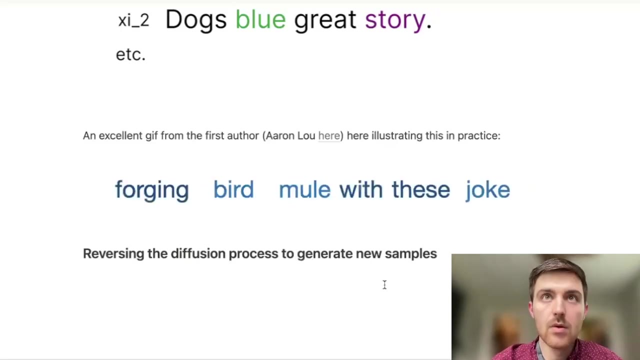 to uh reverse that process. So again we are learning that concrete score from up here, or all of the various T timestamps right For all of the various levels of noise. And once we have learned that, Once we have learned that we are able to kind of use those quantities that we've calculated, 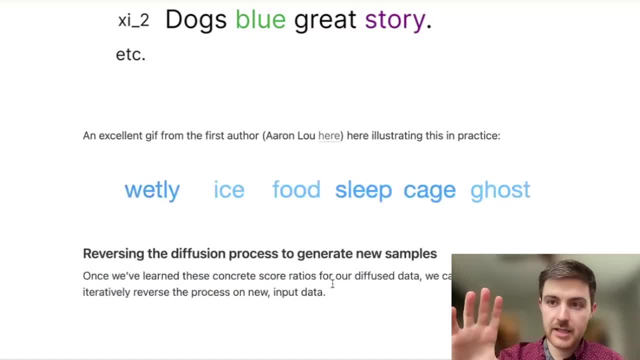 to step back in the opposite direction and D noise the data, and more than D noise the data, D noise just random noise. right, We can just generate a bunch of words, put it in there, um, and get out a coherent sentence. 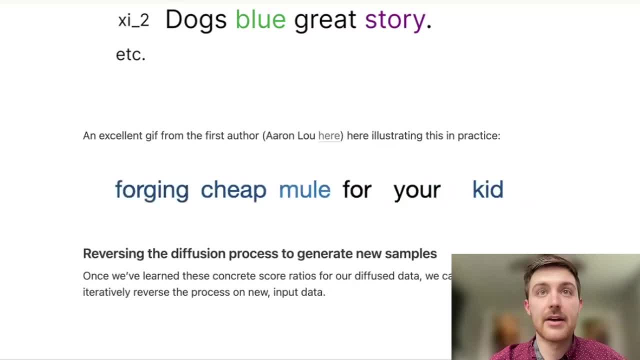 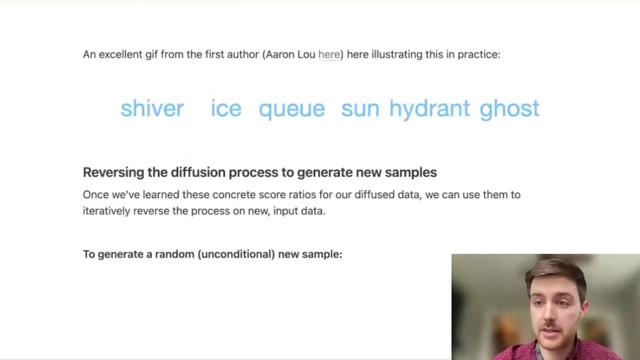 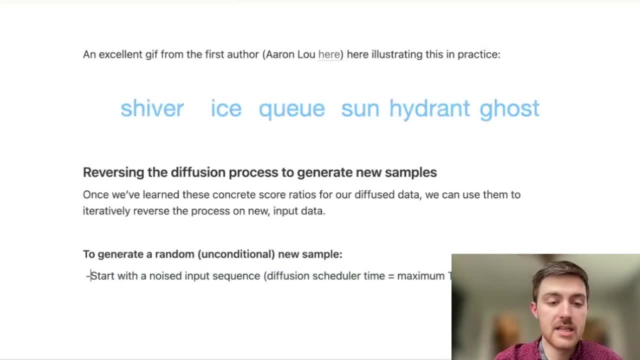 say to you, you start with a noise input sequence in the length of what you want to get as your output. So you know, for this case, 1,024 tokens. you then take those concrete scores that were learned and step backwards in time through, you know, removing a little bit of that noise. 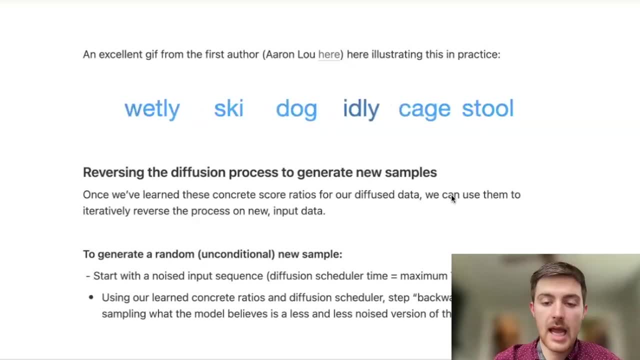 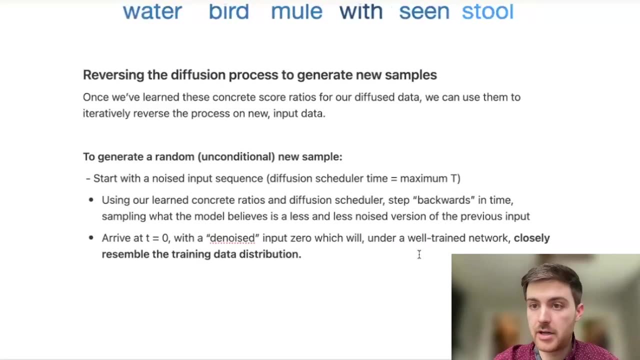 to the best of the model's ability at each time step And then when you get back from time, you know whatever your max T was to T equals zero. you in theory, if your model is trained well, And then you have a new generated observation that closely resembles your data distribution. 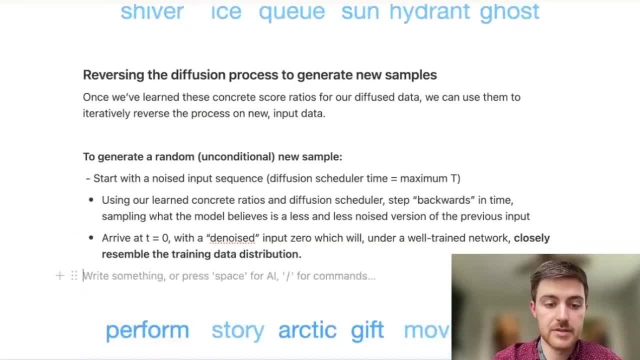 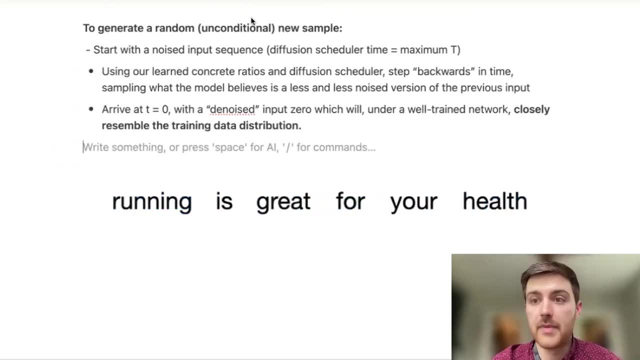 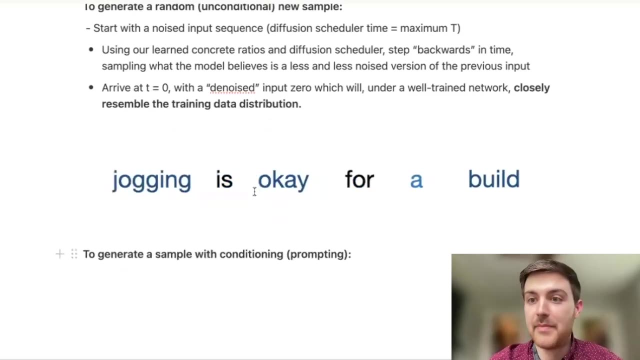 And the author has another really great uh visualization for this: um, moving in the other direction, starting from total noise and gradually introducing signal uh through that reversal process. But, uh, random samples are fun, um, but conditioned samples that we were able to guide and get. 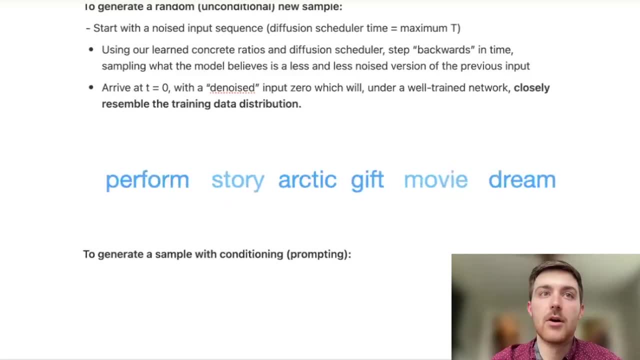 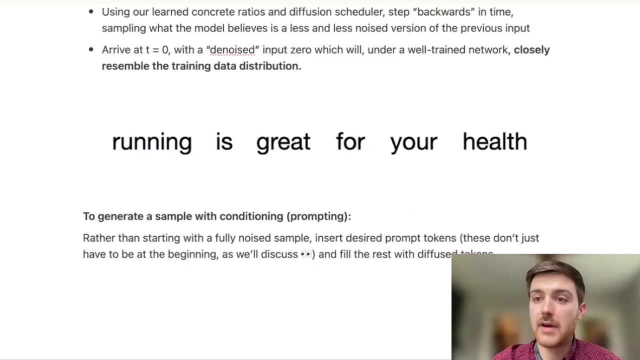 kind of you know what we want via prompting are even better. Um, so this is- This is pretty intuitive- rather than starting with a fully noised sample instead, um, insert some tokens, rather than a fully random token list, uh, that you are interested in retaining. 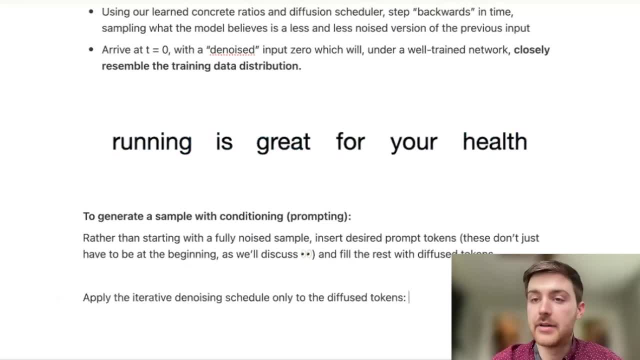 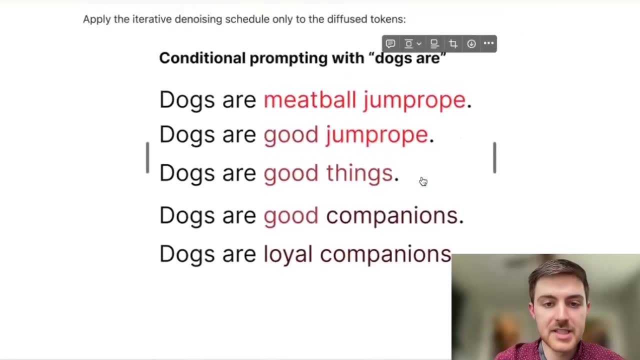 Maybe it's the first two, and then you only apply that iterative denoising process to the tokens that you did not provide. So this is kind of my take on what that looks like If you were to just prompt with dogs. are you initialize the rest with random noise and 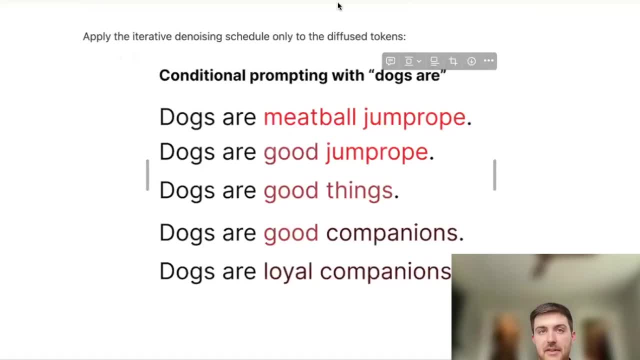 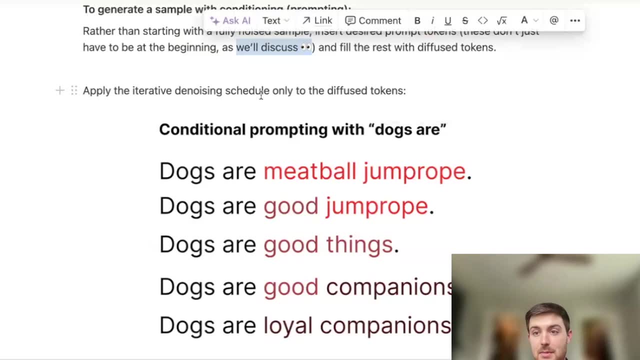 then only perform those denoising steps on the part of the sequence that you did not provide. The interesting sneak peek with this that we'll get into when we talk about why this is all a good thing to do- is that this is really the only way that you can prompt auto. 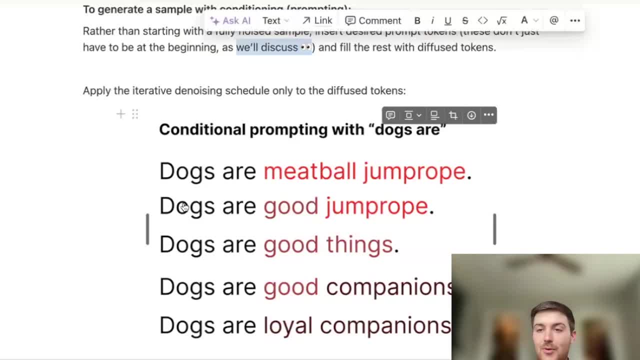 arrested LLMs right Start at the beginning: Um, but you can prompt much more creatively uh with these, which is really interesting. You could do every other word if you want and just have kind of an alternate with uh. 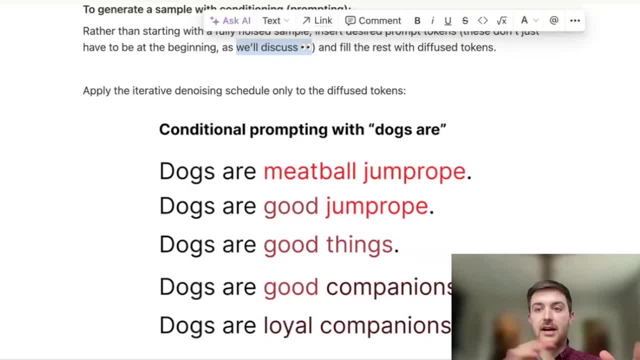 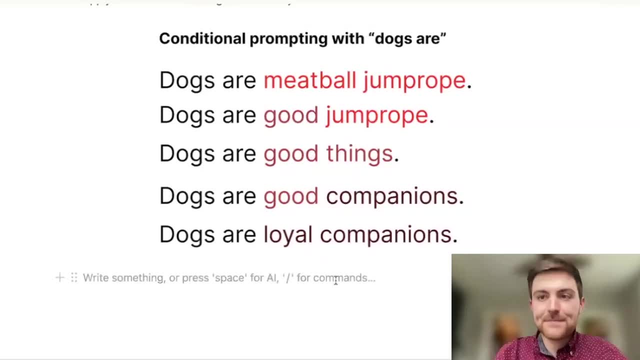 with randomly generated words that are then diffused within the context of your sentence that you already provided. It makes me think of, uh, code completion. Yeah, Code completion too, Cause you might want, like context on the top and context on the bottom and then fill in. 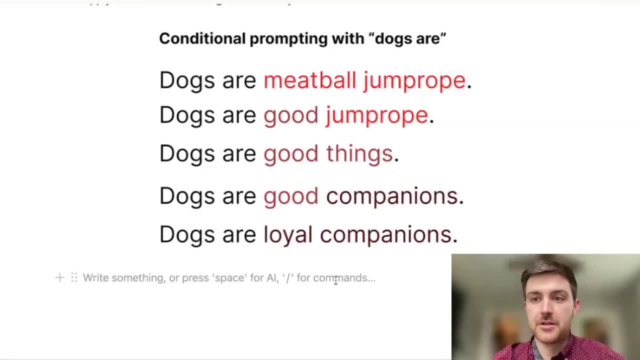 the middle. Absolutely Yeah, And it's just so much more efficient to be able to do that directly and naturally rather than uh, saying you know, as a part of your full prompt, saying, Hey, do all of this, and then have the LLM have to repeat your beginning and your end and fill in the middle, um, in. 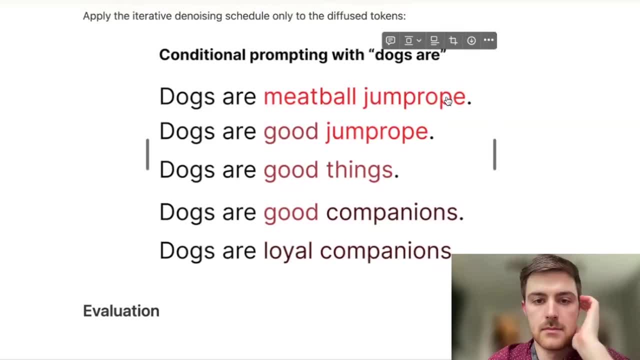 a way that's coherent, But this doesn't. this doesn't have the ability to change the length of the text in this case. right, You can only change individual tokens, Correct? Um, so, like this you're, you are still kind of limited by your input sequence, or sorry. 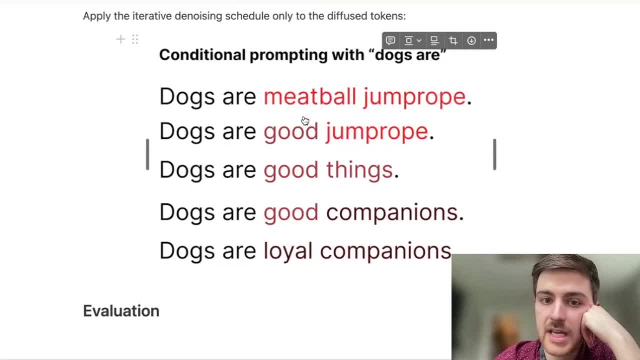 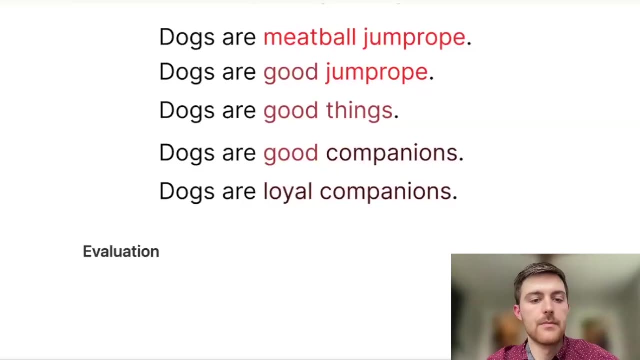 your desired output sequence length: Um, but you could kind of have the, the. you could still get short, um short output sequences by just having you know like early stops being predicted by the model Cool. So that's what they did. 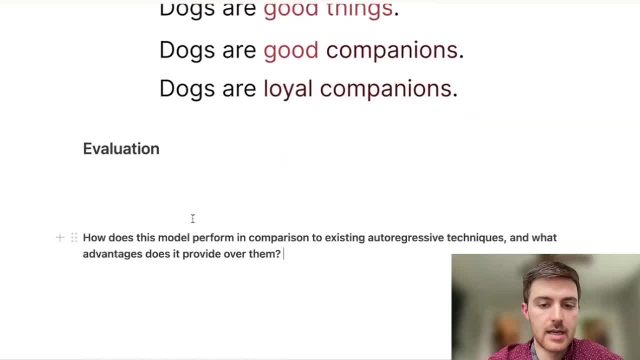 Um. the question then becomes how well, Um, and in particular, how does it perform to a the existing text diffusion approaches that existed prior to this paper, and be those auto regressive techniques, um, that have been state of the art for so long? 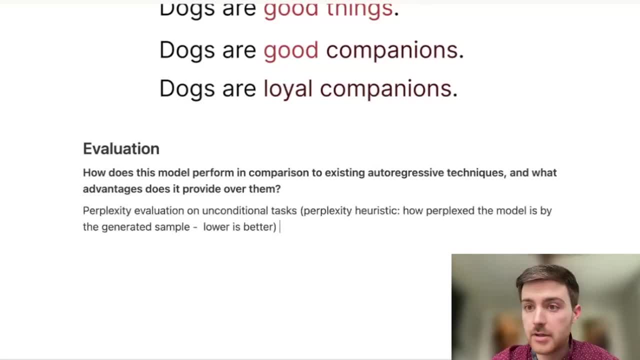 So what we're using for evaluation here is the perplexity score um for the unconditional tasks, which again the heuristic um is how perplexed is the model by the generated sample right. So less perplexed is more coherent, more likely text. 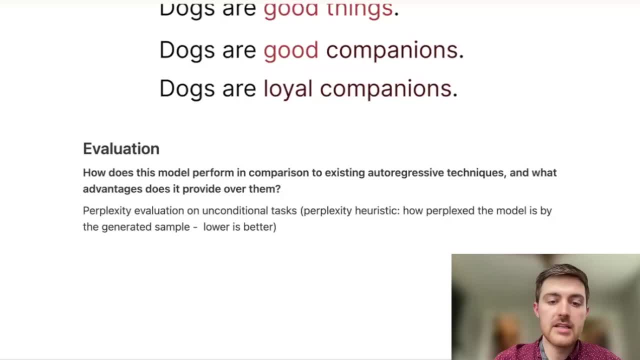 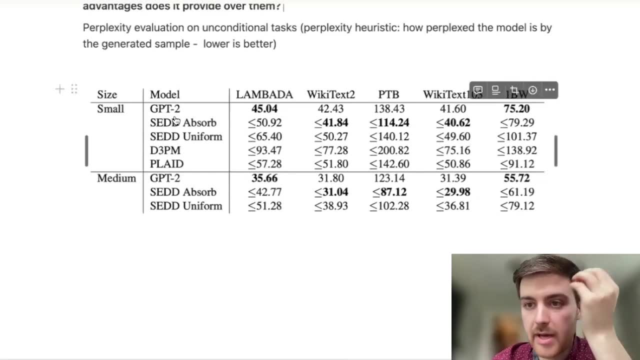 Um, so that's a better, a better thing. Um, here is their eval table on a variety of data sets across uh against. you know they compare to their small model, to GPT two small model, So similar size. there you can see the SEDD absorb and uniform are two variants of uh. 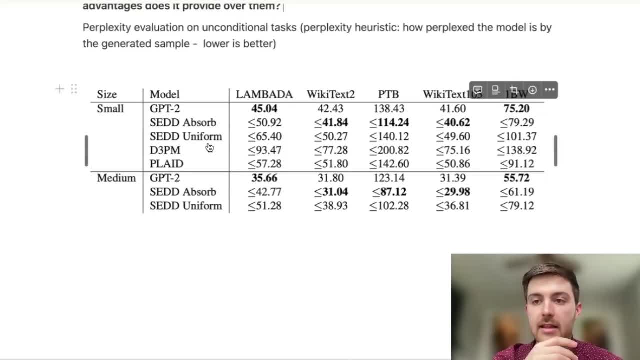 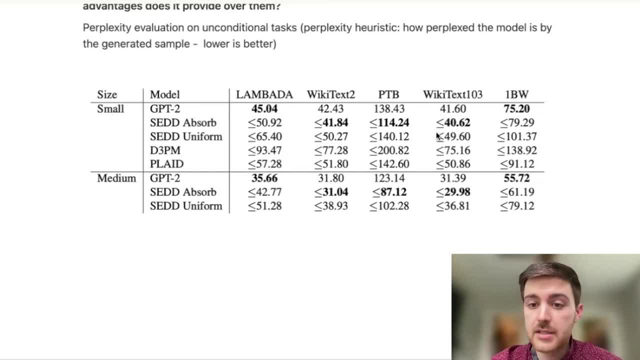 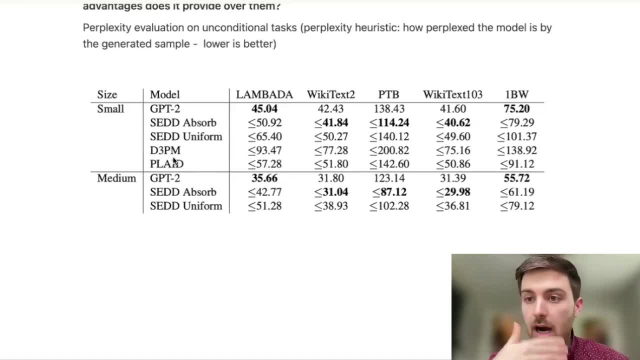 categories, Um. but it is better than D3, PM and Plaid which are other discrete or other uh text based diffusion approaches, Um. so it is kind of a significant state of the art for diffusion and is also competitive with those auto regression models, at least in unconventional. you can see in both small 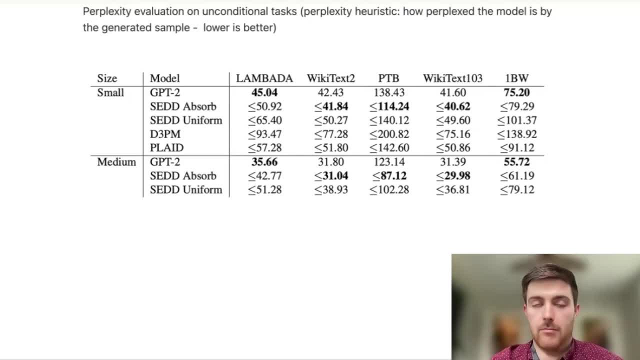 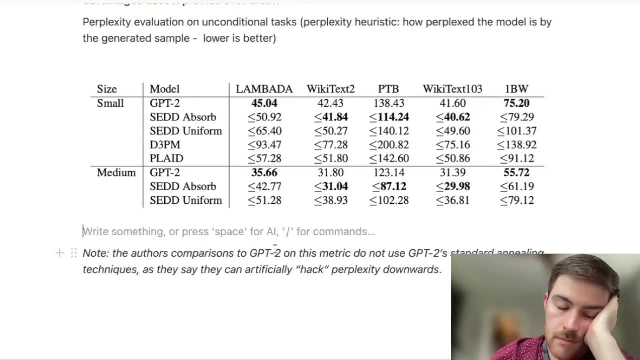 and medium, beating GPT two, three out of five times. Yeah Right, little bit to you know. at the start we said sequential sampling is slower and it has this dependence on being parallelized. at inference time Seems like we still have to sequentially. 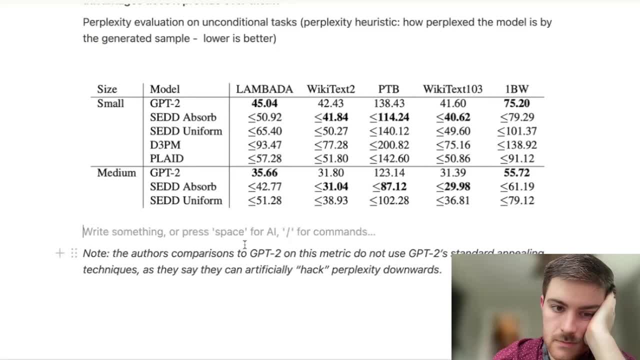 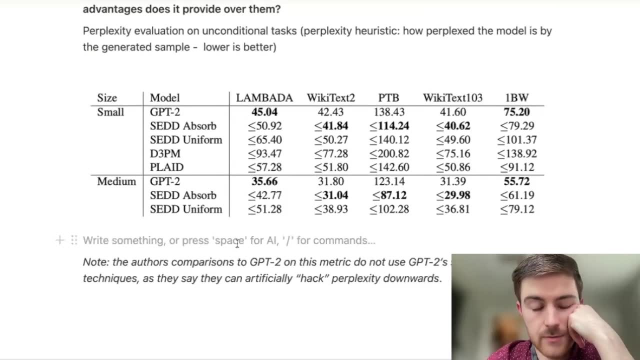 sample in this case, but like there is some parallelization we can get from this type of model. Uh, what do you mean about, like, like the continuing to sequentially sample? Well, we're, we're sampling in time instead of in. uh, yes, 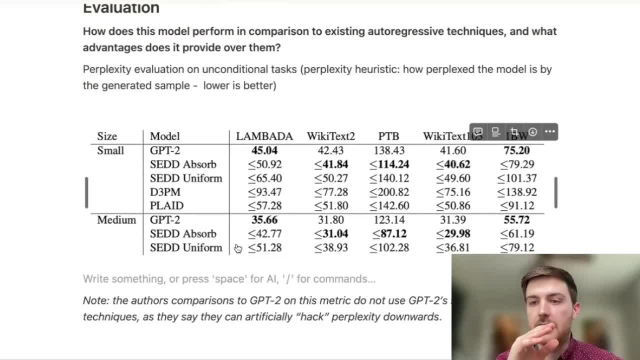 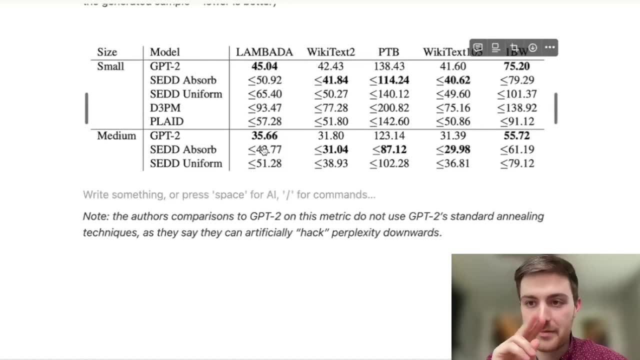 Yeah Yeah, Okay Yeah. So, instead of like, I might, uh, I might- stick a pin in that, because I have a graph about it in a second. Um, but the point, the biggest point there being, yes, we're still taking many steps, but we're taking steps in a different dimension. 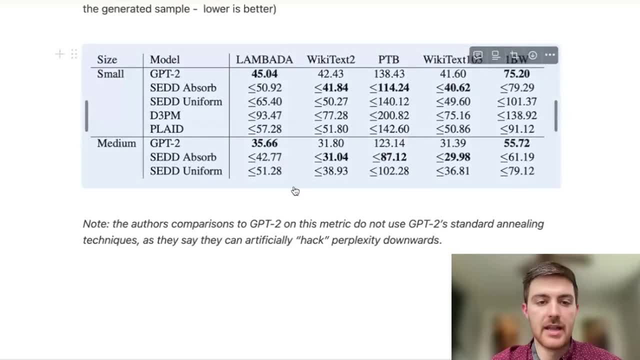 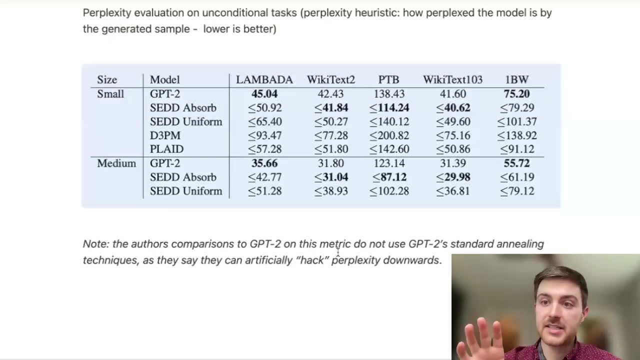 uh, which will come up in a second. So one note on this is that the authors basically say: uh, we talked at the beginning about how there are those kind of additional ad hoc tech techniques that are included to prevent the sequence from running wild in autoregressive generation. 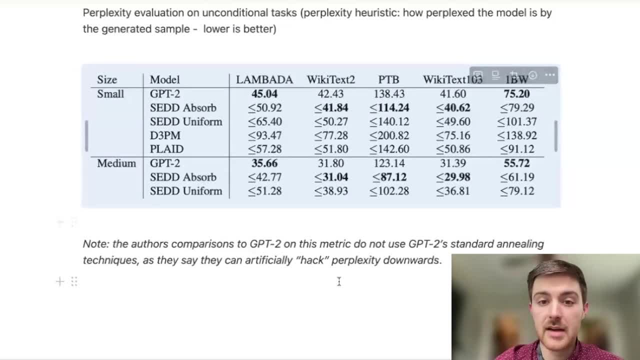 Those annealing techniques like nucleus sampling. this comparison, I believe, is done with those techniques turned off for GPT-2, um, because the authors believe that the uh, those uh sequences are kind of almost definitionally uh improve that score kind of artificially above what the 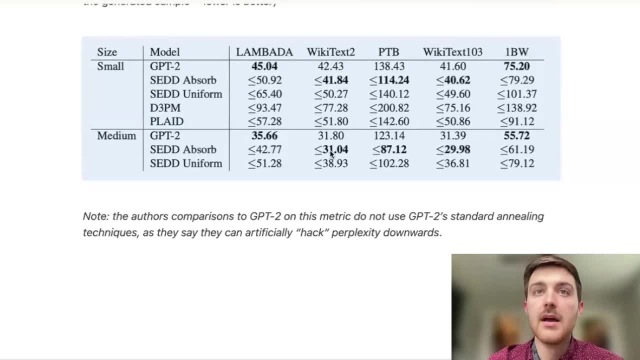 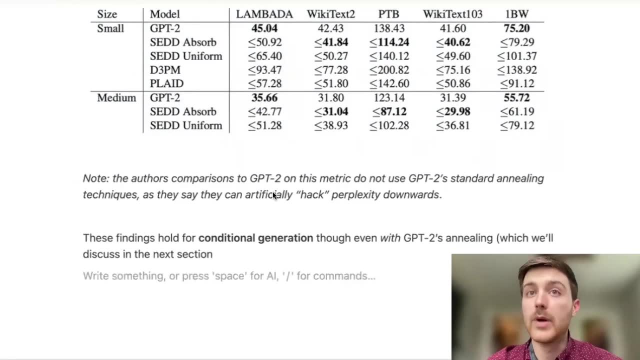 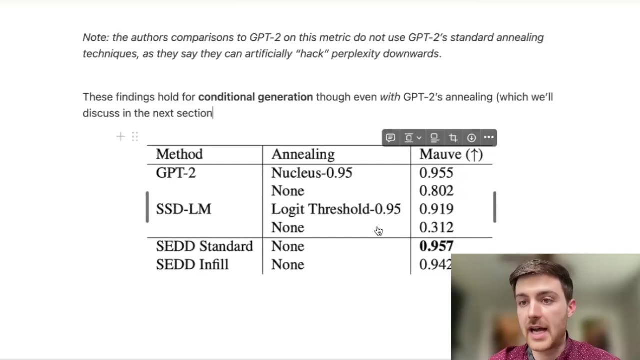 model would produce under, under, you know, natural empirical conditions. but they do have a conditional generation test where they use a different metric that does not have the same um weaknesses. So they are then able to compare against um GPT-2 with its nucleus sampling, and they are still, you know, find that their approach is. 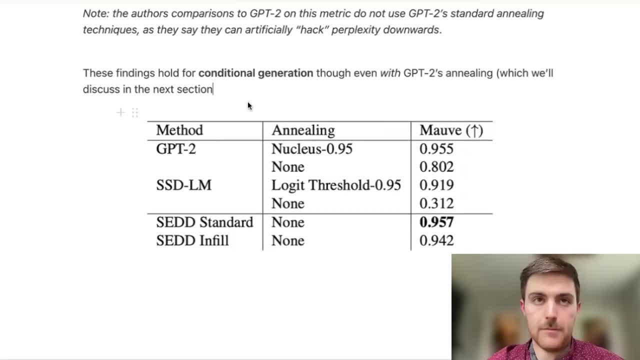 able to able to improve, um, improve on that, So competitive at both conditional and unconditional with existing autoregressive approaches and, uh, a lot better than existing diffusion approaches. So again, we're talking about GPT-2 here a lot. Um, why is this something that's impressive? 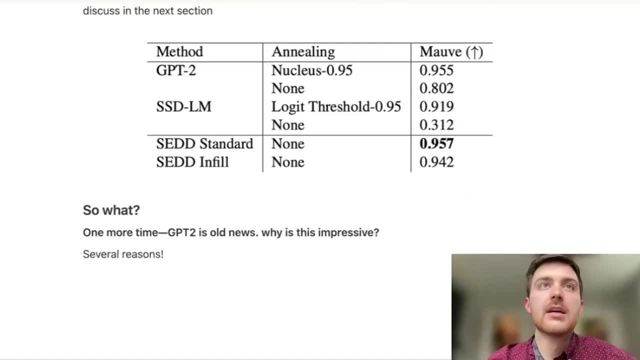 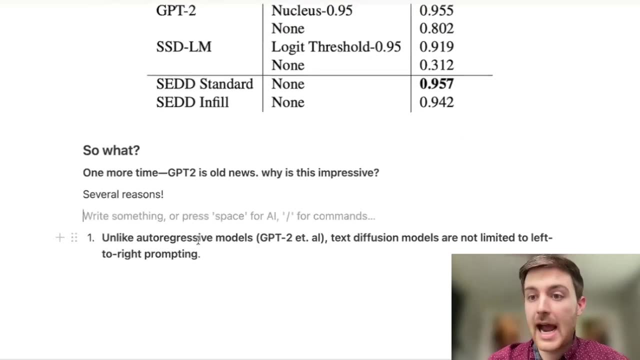 This is a little bit of a rehash of the things that we discussed at the beginning, um, but with a little bit more context and understanding now. So the first is that we said autoregressive models like GPT-2 have to prompt, from left to right, This text diffusion. 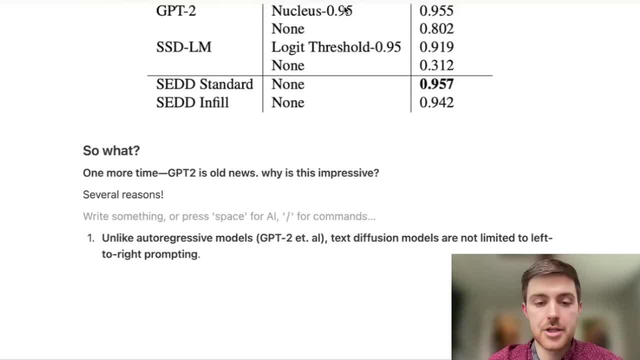 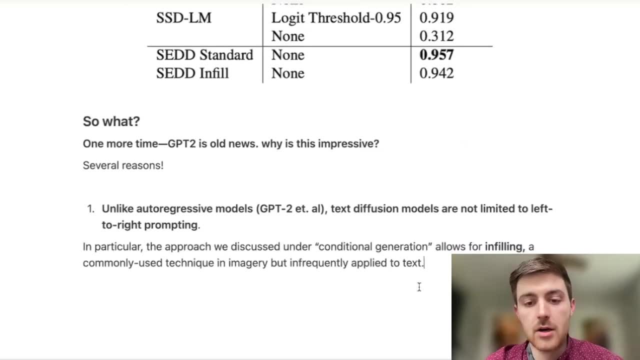 model does not have to do that. Um, and you know, in addition to being more parallelizable, that also gives us what we were talking about in terms of code completion earlier right: The ability to infill. So, instead of just prompting- um, you know from the beginning and letting the 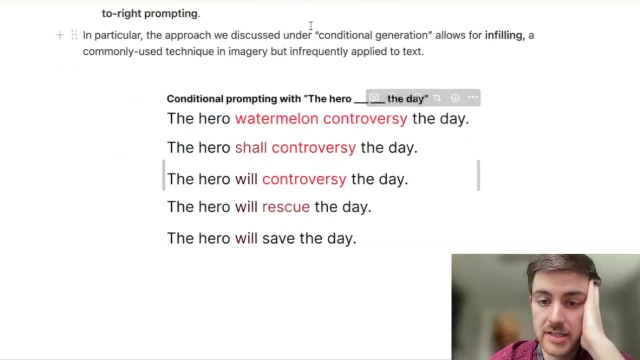 model fill on the rest, we can, you know, diffuse a couple of tokens surrounded by a couple of other tokens. So that's a little bit more context and understanding now. So the first is that we said, you know, autoregressive models like GPT-2 have to prompt from left to right. So that takes us from. 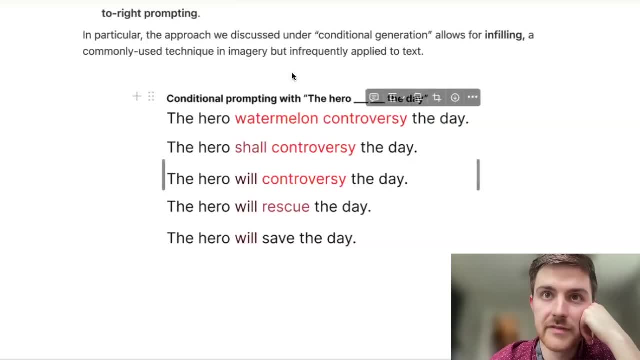 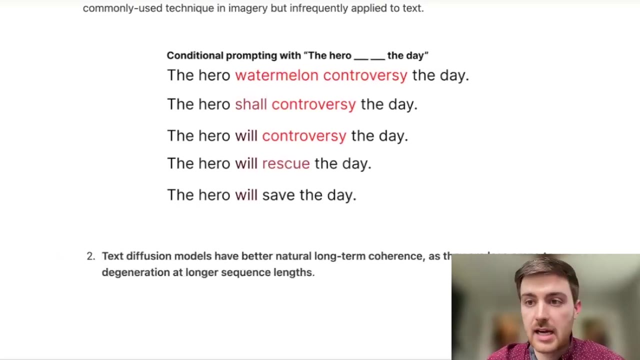 the hero- watermelon controversy of the day- to the hero: we'll save, uh, we'll save the day, and you know, simple example, but lots of, lots of possibility for our extension there. Whoops, Sorry, Okay. Second of our big three things is that, uh, there's reason to believe. 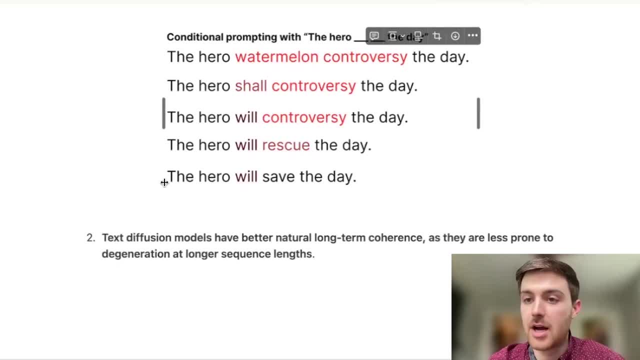 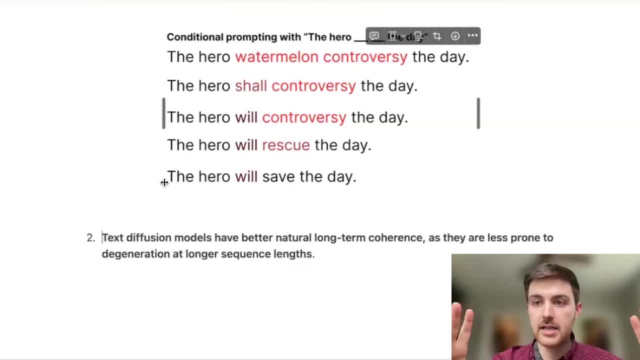 and degeneration at longer sequence lengths. right, These are all being generated, as you know, over time as one coherent whole, which we'll talk about in a second Um, but they don't need. they're able to achieve the performance of autoregressive models that do employ those. 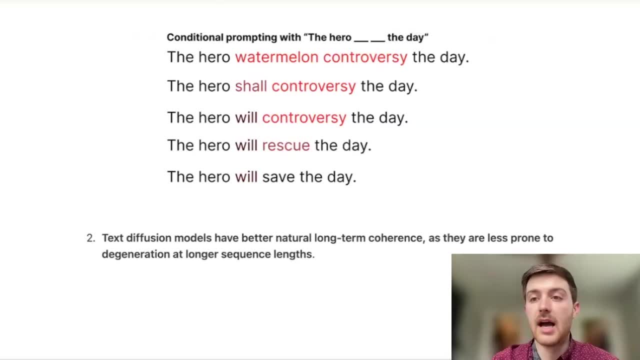 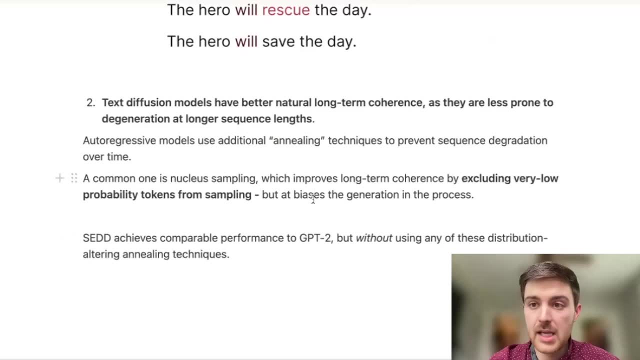 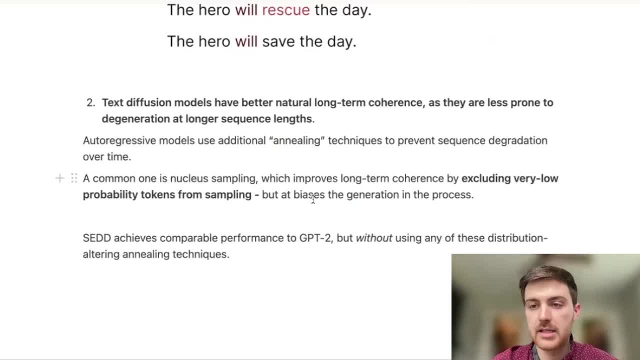 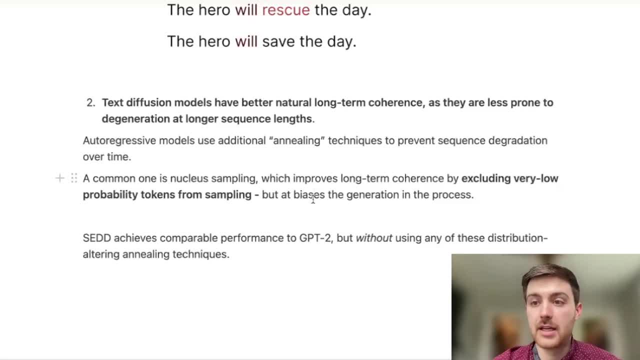 from flying off the handle, Um, but I would argue that it also can kind of, uh, limit the, like you know, creativity and variance of possible outputs, Um, if those kind of lower probability spaces at at higher temperatures are not being explored as frequently. 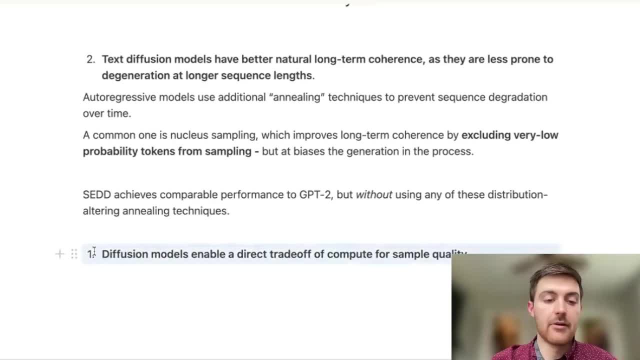 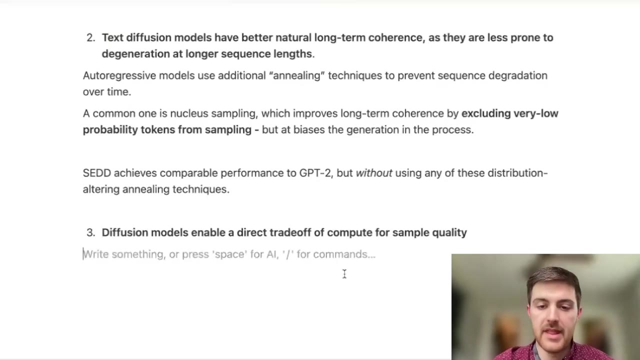 And then this third one is the big thing that Greg was talking about, and this is that diffusion models allow you to you know, know, establish and pick, pick your spots on a trade-off between how much compute you want and the sample quality. So I mentioned this earlier, that and Greg was talking about it just a second. 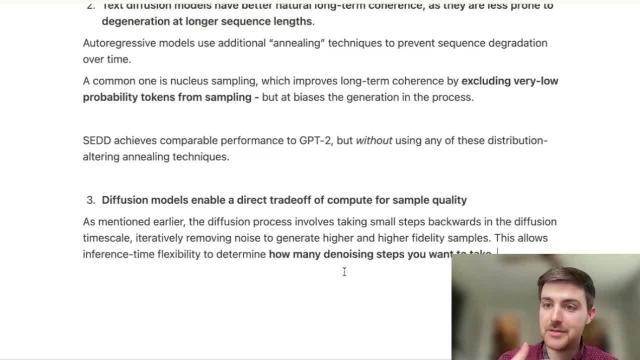 ago that the diffusion process still does require you to. you know it is still iterative, but rather than generating token one and then token two and then token three, you generate a bad version of the entire sequence and then a slightly less bad version of the entire sequence, And you continue. 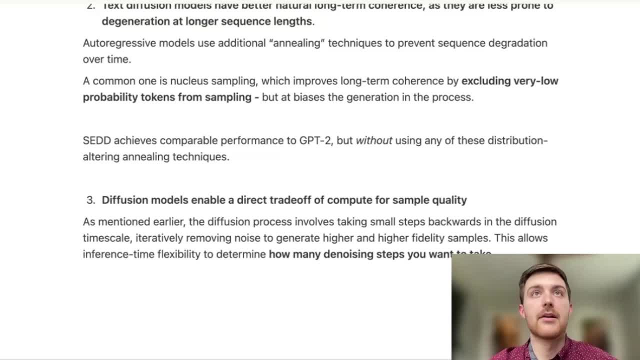 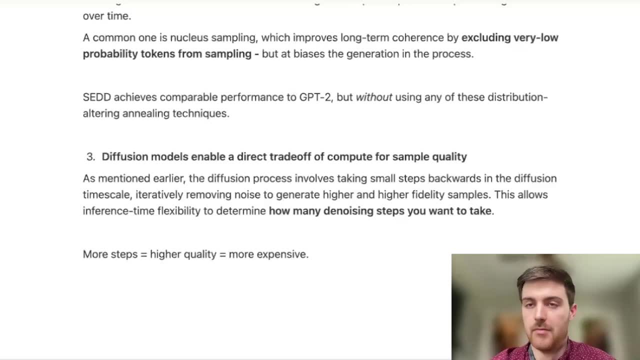 to do that, stepping through time and getting a little bit better each time. So, basically, more steps of that generation process leaves you with a higher quality generated sample, but also means you have to, you know, evaluate your network more times. And this type of trade-off because of the 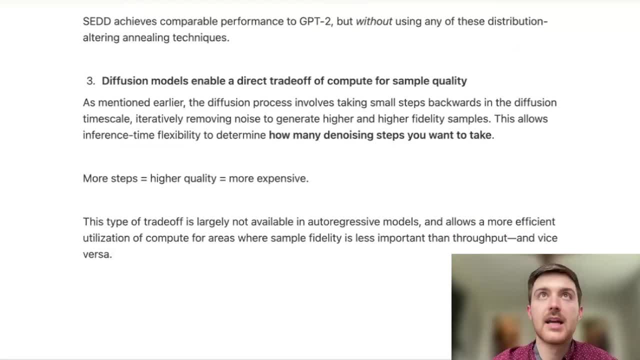 autoregressive nature of things like GPT-2, is not something that we typically have access to in that case, because the GPT-2 is not kind of iteratively improving its sample as it goes on. It is, you know. 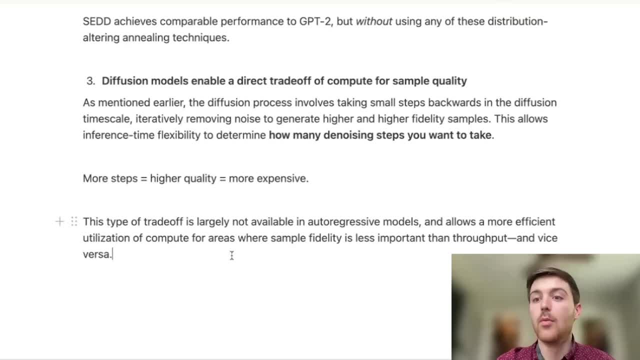 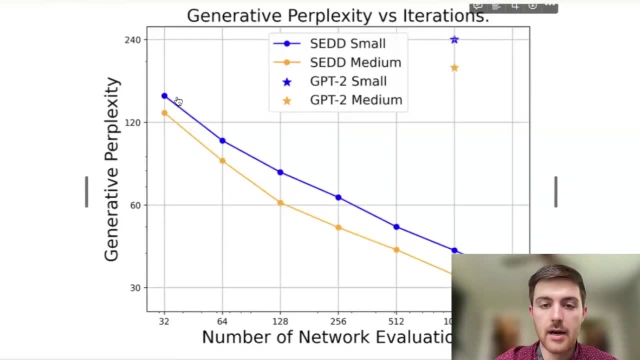 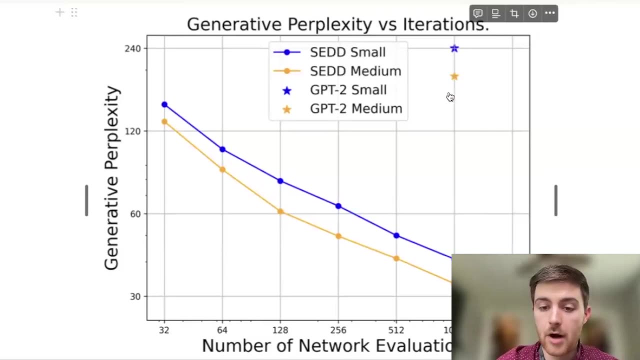 running 1024 network evaluations, but that is to generate 1024 tokens. So the authors did a perplexity comparison. You can see that the circles are their networks, these SEDD networks, and the stars are GPT-2.. You'll see that GPT-2 are just frozen at 1024.. That's because they 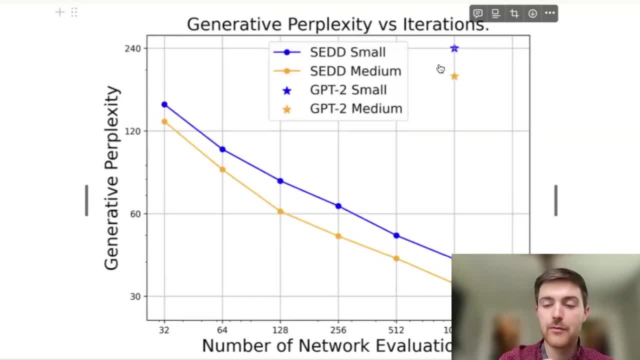 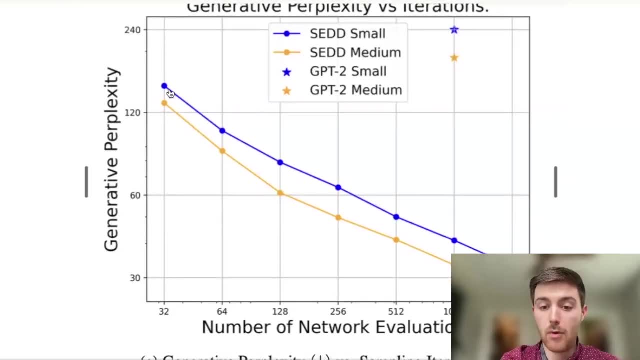 have to make 1024 evaluations to generate a 1024 length sequence. no matter what, They don't have the ability to participate in this trade-off, But perplexity again going down here. so more network evaluations is better, with these lines indicating the performance of SEDD. 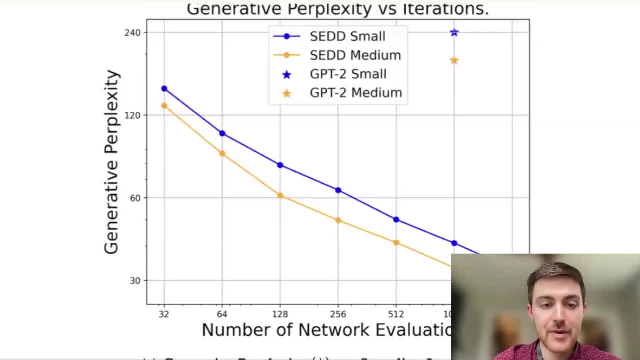 If you want a really cheap evaluation that is not going to cost that much compute but is also not going to be that good. you know, you can evaluate it as few as 32 times and get comparable performance to that of GPT-2 without that annealing process that we keep talking about. Or if you want to go. 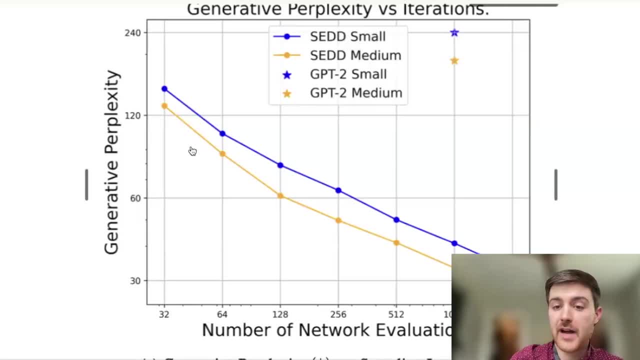 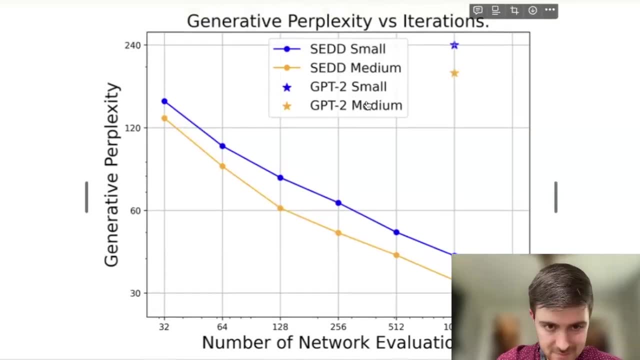 even beyond that and you have compute to spare. you can choose to evaluate it double as many times as you ordinarily would and get an even higher quality sample as a result. So that type of trade-off does not really exist in autoregressive modeling, And I think it is a really exciting. 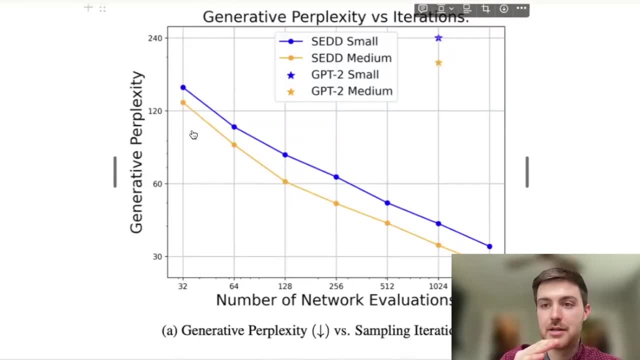 piece of this because it lets you kind of make the decision rather than by having to choose a different model. You can kind of make one model a little bit less expensive to run while kind of trading off some of the quality, for that. Does that get where you were going, Greg? 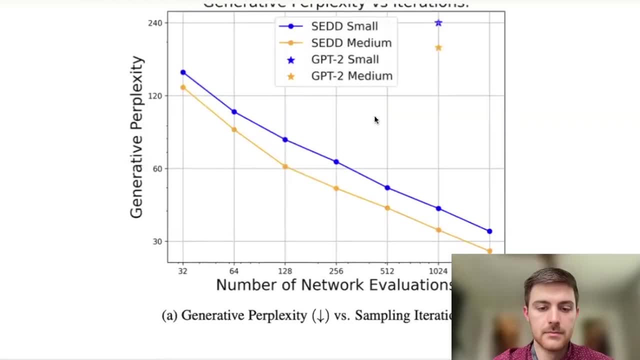 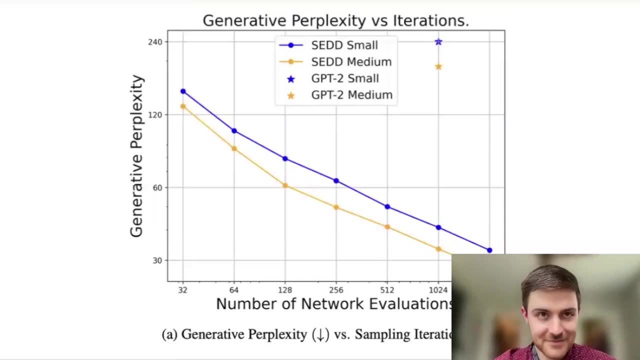 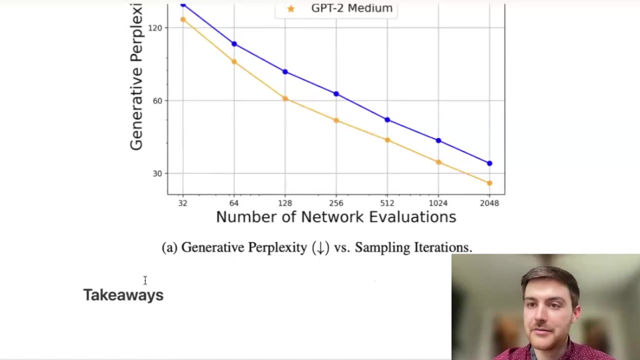 Yeah, totally. This chart is really cool. I wonder if you could even use this to like auto-generate training data To make better samples in like a DPO context. That would be wild, Auto-diffusing, Cool. So takeaways and then we can kill the recording and talk about any questions. 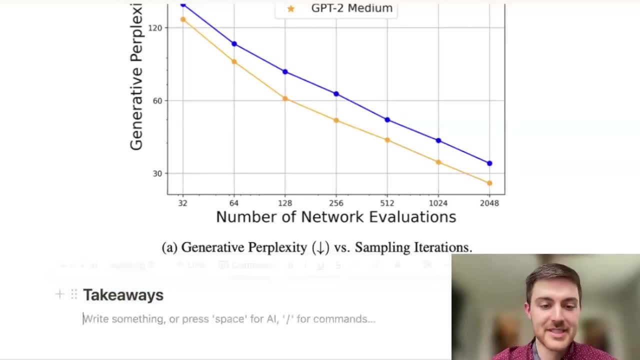 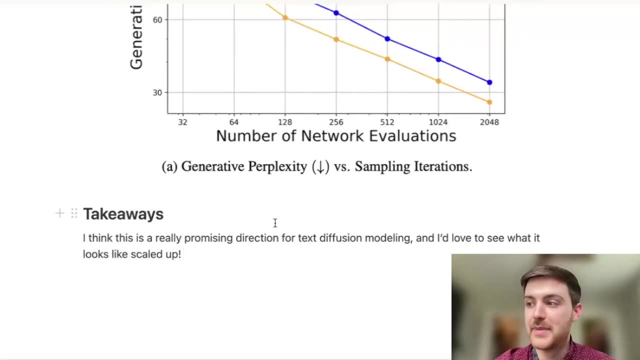 I think that this is a really promising avenue of research. I think it's very cool seeing diffusion methods catch up on text, because they have kind of been so dominant everywhere else. They've been really successful in imagery and video And very recently and topically, in audio and in music generation as well. I do think that just because they are 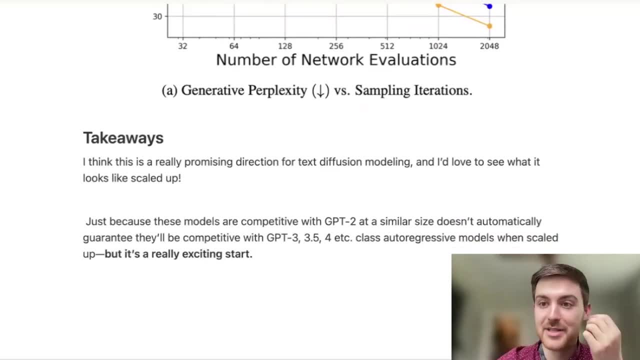 competitive at this particular model size does not mean it will not be challenging to scale them up, does not mean they will necessarily be competitive with these larger models at even larger model sizes. But I think it's a really exciting start and I thought it was super cool. 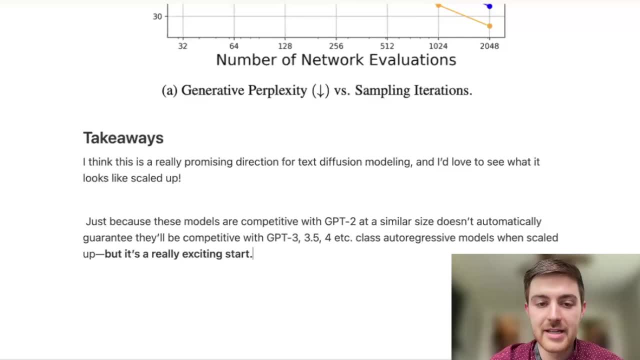 I'm excited to kind of dive into the code next week with Greg about it and present it back to you guys. Cool, Anybody, Awesome. Thanks, Ben. Like Ben said, we'll be diving into the code next week And if you guys, you guys probably. 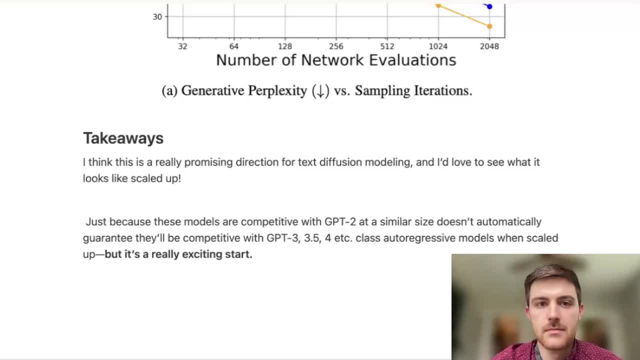 couldn't tell, but Ben is kind of like Michael Jordan on the flu game today. He's been sick all week and still pulled this off, So big round of applause for him. putting this all together. That was super impressive And I learned a lot even having read the paper before. 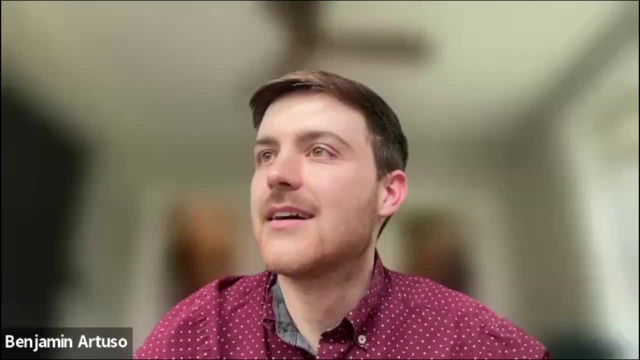 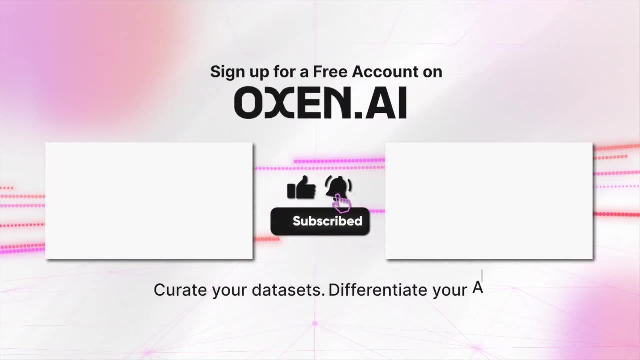 Awesome. We'll kill the recording and open it up for questions here. Thank you so much for tuning in. We'll see you guys next week.